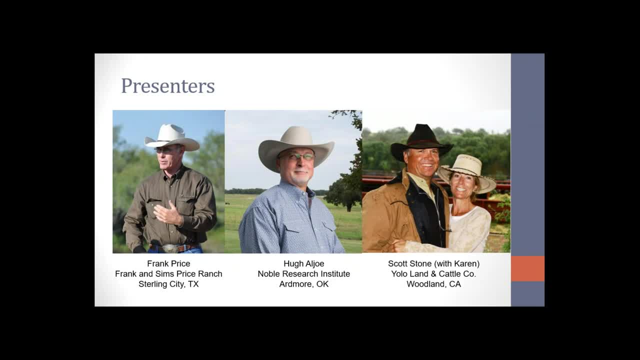 introduce themselves as they speak to you. uh, i'm very interested in this personally, this topic, because some of you may know that i ranch in a six inch to ten inch rain zone on both sides of nevada, so in our operations we're always on drought alert, if you will. with that, i'd like to thank 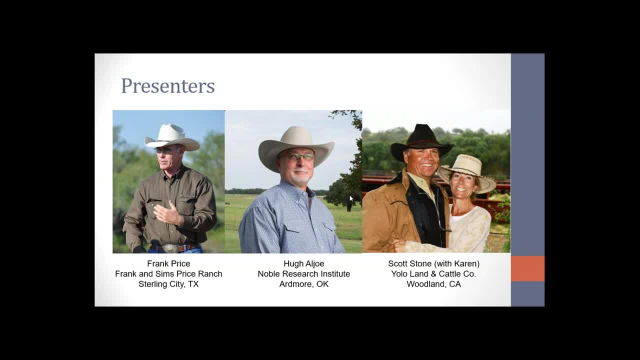 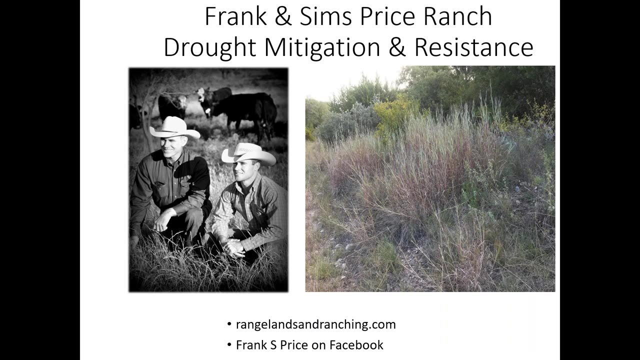 you for taking the time to be here tonight and i also want to say thanks to all of our panelists for joining tonight. and, uh, it's my pleasure to introduce frank price, who, with his son sims, operates a ranching enterprise in the sterling city area of west central texas. he was selected. 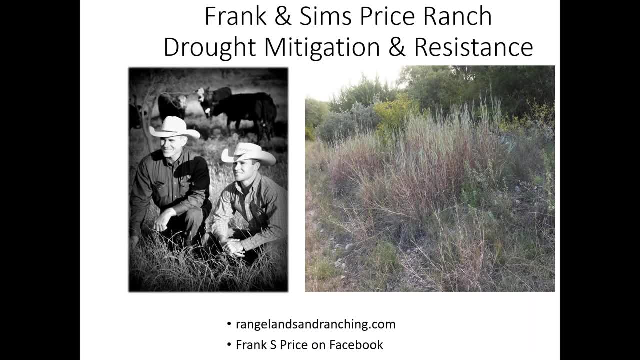 as the national winner of the 2013 environmental stewardship award. Good afternoon. I hope to give you an overview of what we've done to make our ranching operation sustainable and drought resistant. Remember that I certainly do not believe that what we do is best for everyone. Everyone needs to build their own program that fits their operation. 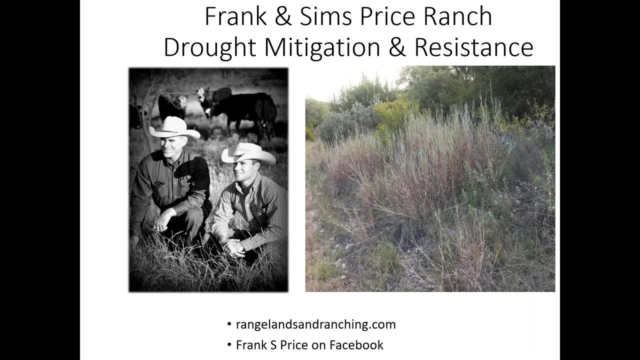 and there's much room for improvement within our operation. Looking at this picture, on the right there's some big blue stem that appeared on some of our rangeland. It was not seeded. I had no concept that we'd ever had big blue stem in this area. 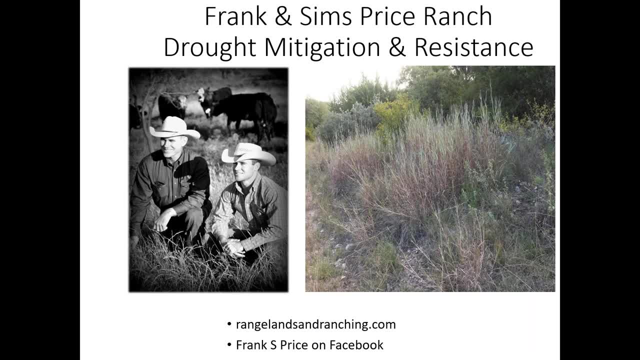 but when we went into a more intensive grazing program it just came to life in tears and I have determined from the cattle's the way they graze it. it is extremely palatable. They'll graze it in the states. you see it now plumb to the ground while they're standing there. 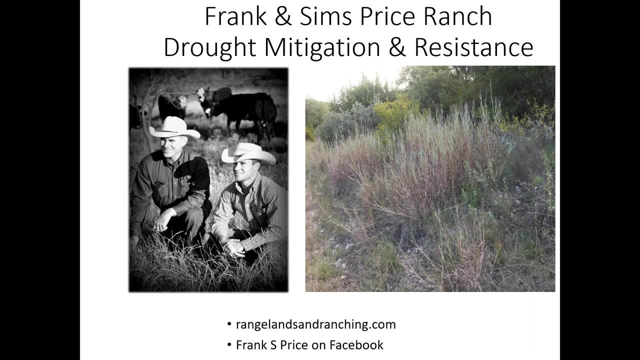 providing them with a lot of food. They're not going to be able to graze it in the fields. They're not going to be able to graze it in the fields. They're not going to be able to graze it in the fields. They're not going to be able to graze it out in the friends Percentage. 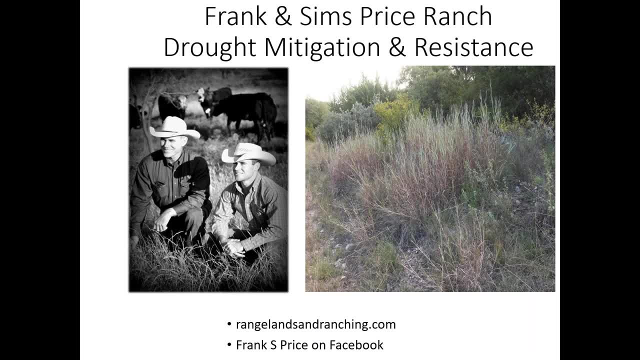 of feeding schedule on Simmons, as you put it actually broadens the reference point for how they health. So it's so chicken, you have to always be very, very careful with it. Good, let's get some the soil. this is what we're going to be using in the next few minutes. 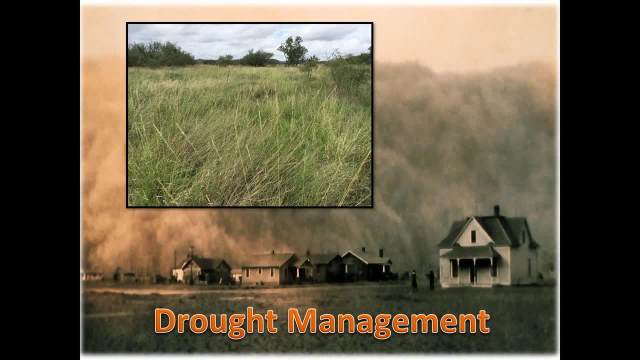 There's a hold of this. It's a, it's what it looks like. It sticks to the grass, So it's not got any from the same issues. Some areas are more susceptible than others, but all rangeland managers are continually facing this management issue of drought. 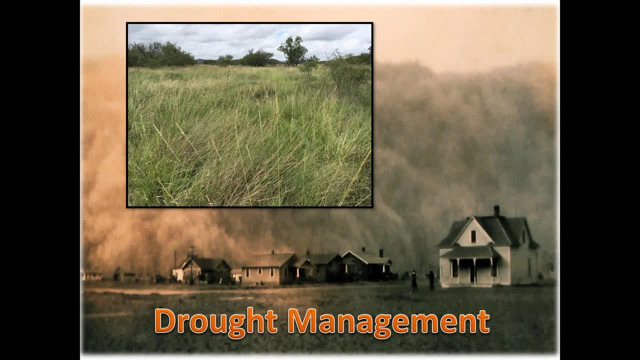 Since 1965, that's the year I became closely involved in the ranching enterprise. I was a freshman in high school- I've witnessed no less than nine extended dry spells. When you divide that out, that comes out to a drought, on average every 6.1. 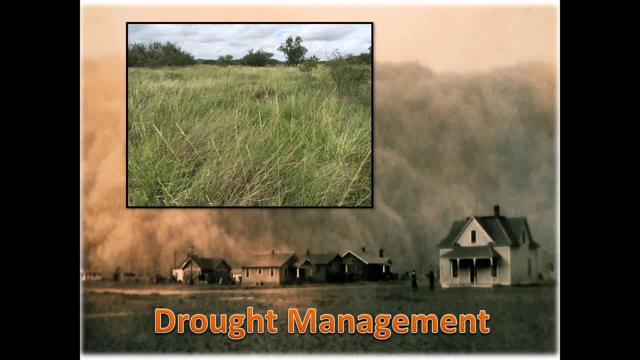 years. This historical study of sorts tends friends show how important it is to be continually cognizant of and being prepared for the next dry spell. Drought isn't an ever-changing event. It is a continual part of the rangeland management process. Here we have a chart showing our rainfall annual. 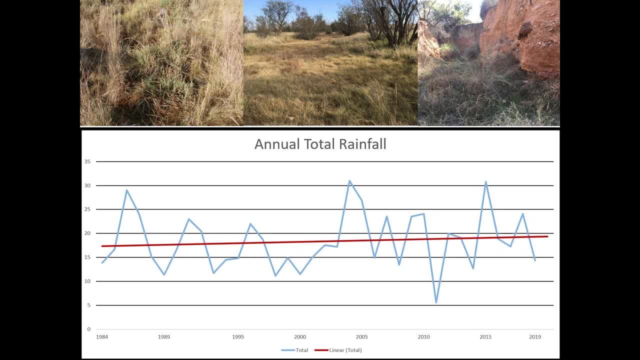 rainfall: Here we have a chart showing our rainfall. annual rainfall- Here we have a chart showing our rainfall. annual rainfall. rainfall: It ranges from 32 inches to 5 inches, an average of 18 inches. You can look at this. 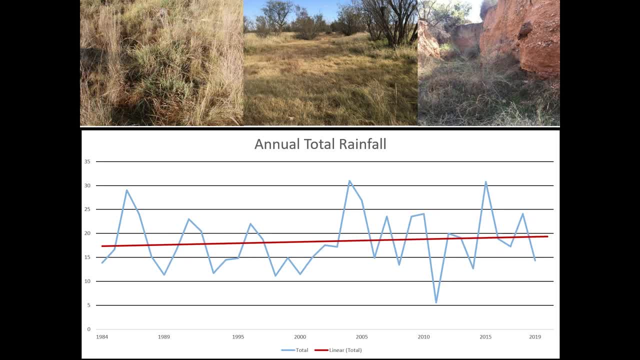 chart and everything below that red line, which is the trend line, is drier than normal conditions. When you have two to three years below that trend line, you're in what we consider to be a drought condition. When looking at this chart, you can see pretty regularly that 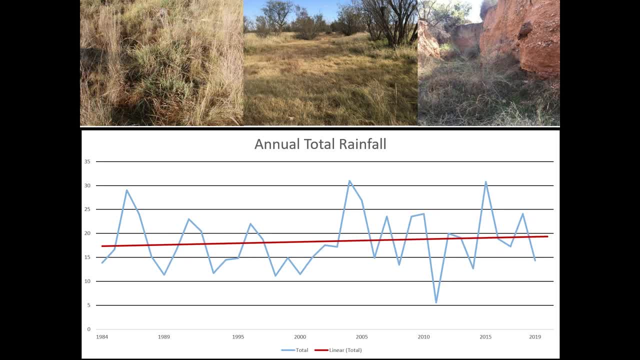 that happens. We're very fortunate to ranch in this area. It's been a cool season and warm season country. I believe I live in God Country. God Country is where a man resides, provided he understands the land and the environment in which he's operating. This chart, I'm not. 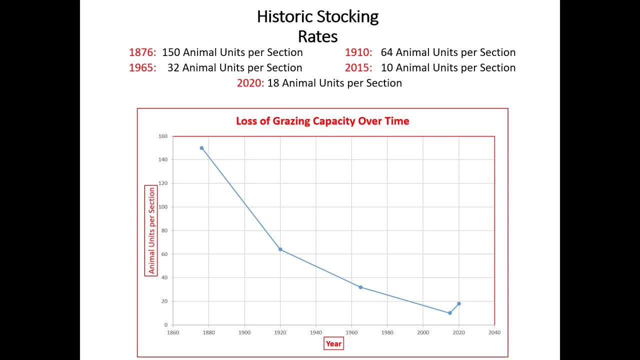 big on charts, but this one is amazing in itself. It starts off in 1876, 150 animal units divided into seven percent Number to the section which is mind-blowing to me In the early 1920s, my great-grandfather's records. 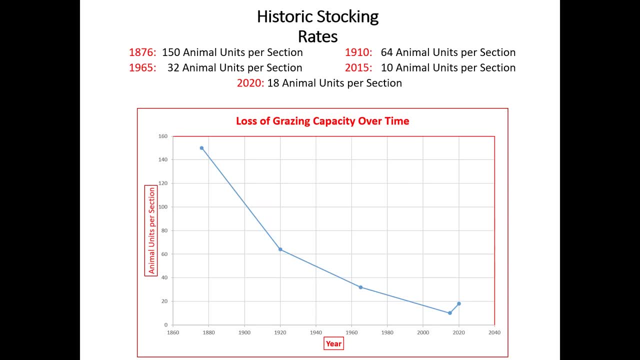 showed that he was running 64 animal units to the section. In 1965, when I was a freshman in high school, my ag teacher told me it was 32 animal units to the section. Then, in 2013,, NRCS did a study in Stirling County. 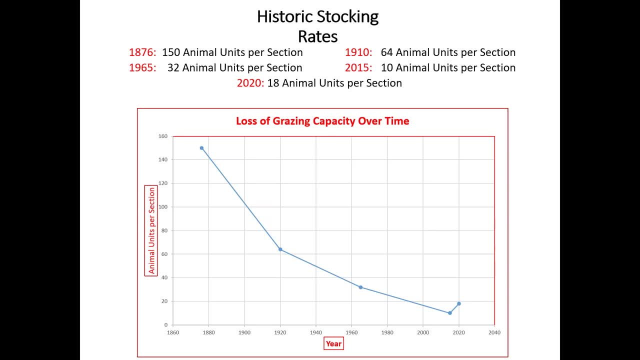 and they came up with 10.. We're going the wrong direction, folks. It's just getting worse and worse. Now that little uptick on the right-hand side shows some improvement we've seen since we initiated the more intensive grazing program. 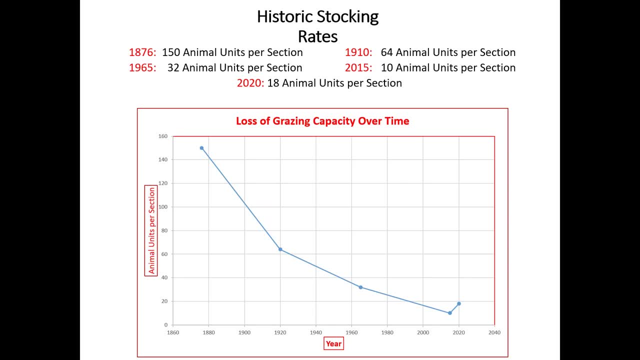 Some would say that understanding the common, almost regularity of drought and the loss of grazing capacity of our rangelands can be correlated, to prove that drought is the cause of that loss of grazing. A long-time friend, mentor and neighbor told me very early in my career, with each succeeding dry spell, 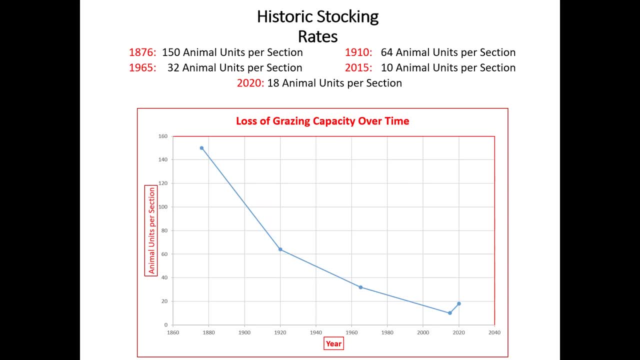 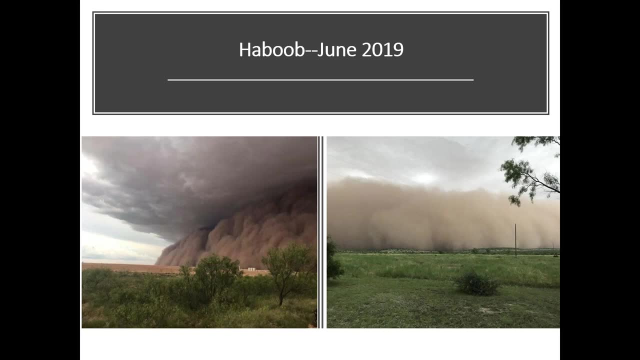 or drought. we can never run as much livestock as we could prior to that dry spell. Now, the first weather-related event of my life that I remember. I was three or four years old, playing outside. I looked up and in the Northwest. 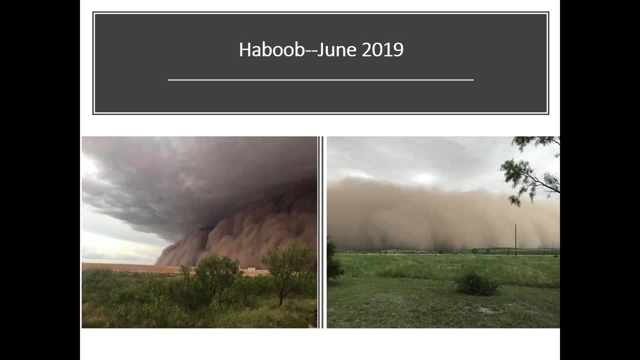 here came this huge rolling red cloud. Like a scared puppy, I ran for the house And, as far as I was concerned, before I got to the house it was totally dark. That's quite a childhood memory. That was in the 50s. 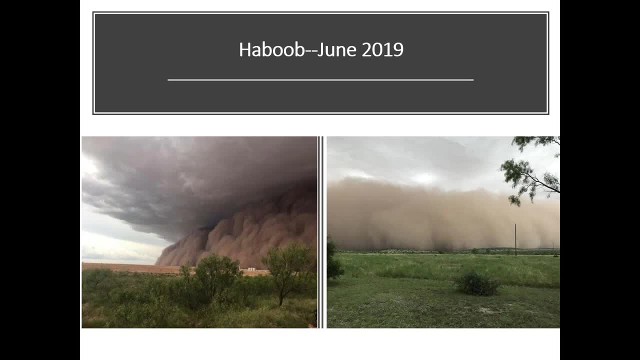 In the 30s, the dust, storms, the hubbobs, if that's what you want to call them, were much worse. The picture you see here was in June of last year, But they're still occurring. Studies of tree growth and sediment studies show that drought 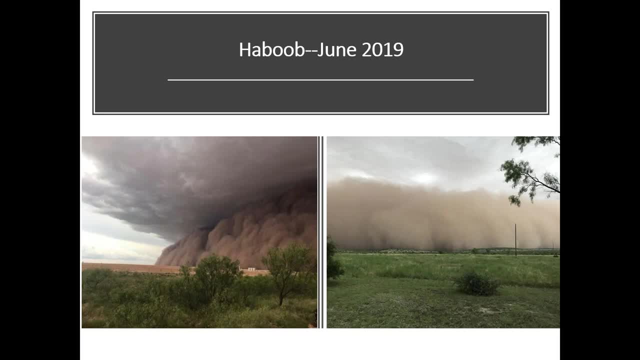 which has been with the land for hundreds of years, probably thousands or tens of thousands of years. And yes, drought has on grazing conditions And, as my neighbor said, those droughts permanently reduce the grazing capacity, in particular when you're in a continuous grazing program. 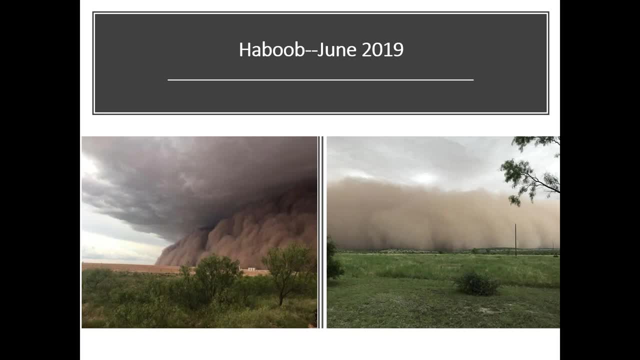 My opinion that we, as rangeland managers, have failed to recognize the cause of rangeland degradation as a result of continuing drought. That cause is the lack of giving the rangeland the opportunity to recover from not only the effects of drought. 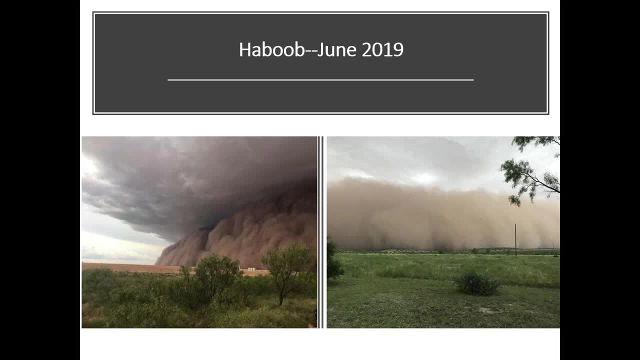 but the effects of grazing. The cure is proper grazing, utilization of rest after grazing. Total rest is not the answer, As, over the millennia, the Lord and his helper, Mother Nature, developed plants adapted to the graze-rest process that the buffalo, elk and other wildlife create. 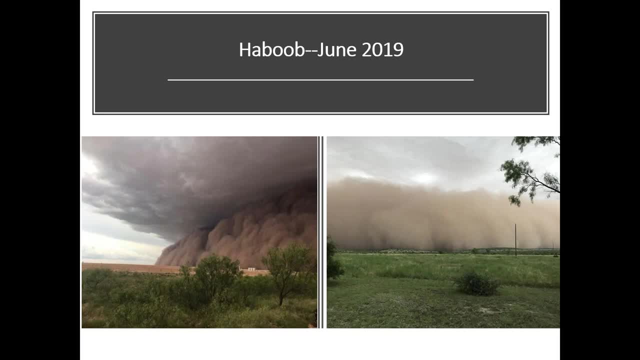 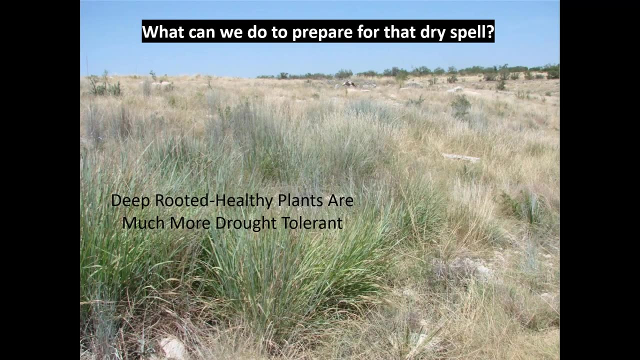 Understanding the relationship of drought and rangeland management are what we're going to discuss today. What can we do to prepare for a dry spell? First and foremost, use a planned grazing program that produces a healthy, deep-rooted, continuous solid turf of perennial grasses and farms. 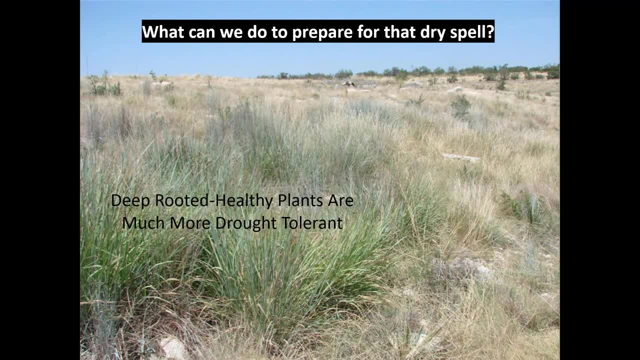 both cool season and warm season. This puts the ranchman in the position of getting away from a continuous grazing program and utilizing a planned rotational grazing program. That is the hardest management change for most producers, but it is by far the key and most important change. 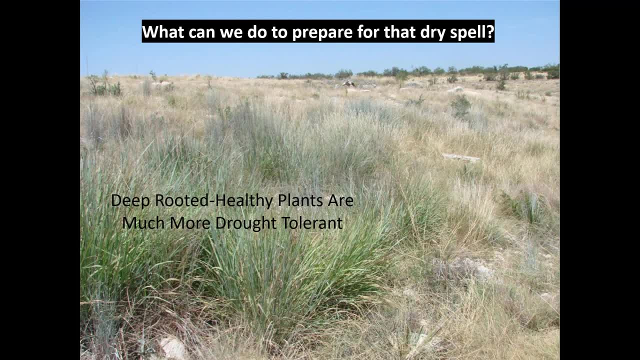 a manager can make to establish long-term profitability and drought resistance. It's possibly the largest determining factor to that profitability When it comes to a half-inch of rain on sparsely-vegetated, unhealthy soils bare ground home. most of the time that variable moisture 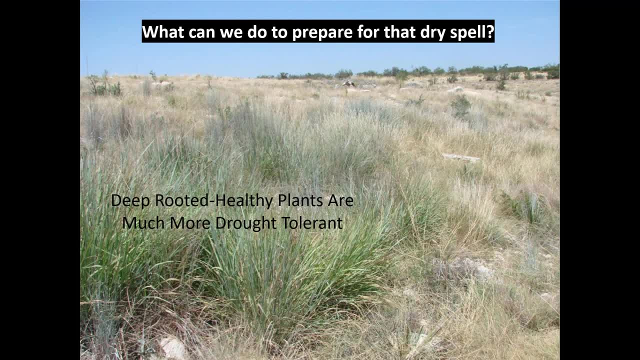 valuable moisture is quickly lost to wind and sunlight evaporation that runs downstream to the neighbor's rangeland, effectively producing no rangeland recovery. Conversely, that limited rainfall on healthy rangeland that is shaded by dense perennial plants in the litter that is always present. 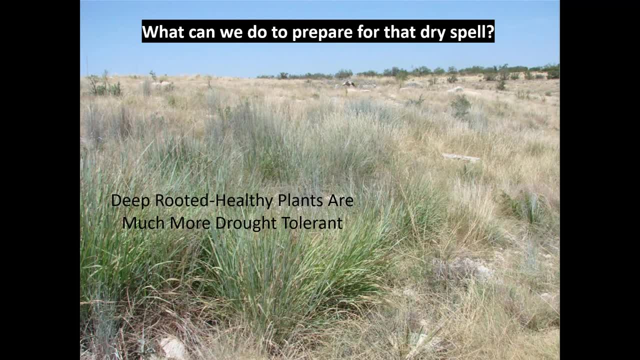 healthy soils can be an effective rainfall, even after an extended dry spell. I observed this last early fall. We've had no rain through the summer months. Came a half-inch of rain Four days after that. rain go down into those areas that had that dense cover of grass. 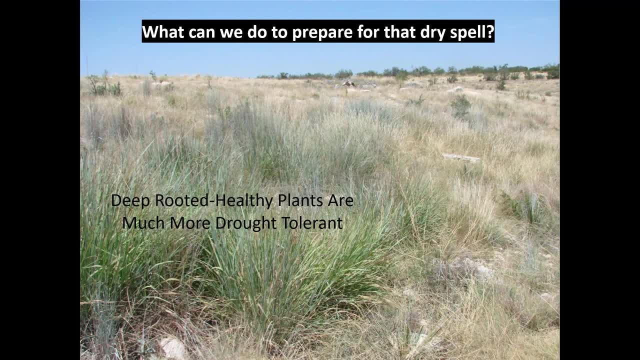 there's still moisture there in the soil. Pretty exciting to see that happen. Now, then, utilizing this, of course, approach has produced recovering rains that is much more drought-reducing than continuous rangeland. We have run from drought, sending livestock to other areas. 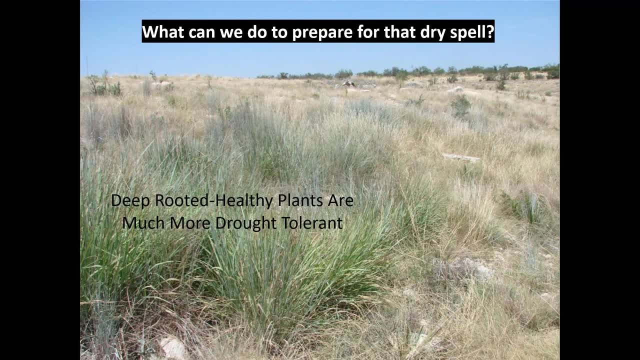 utilizing heavy feeding or cut numbers drastically. However, recent dry spells with rangeland recovery due to the intensive graze rest program, we've been able to limit reductions in numbers and certainly have not had to utilize the very expensive options of moving livestock to rangeland. 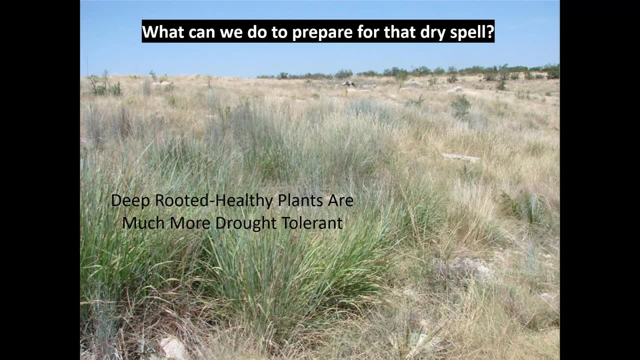 that has received better rainfall. Now you look at this picture over on the deep-rooted healthy plants. they're much more drought-tolerant. The green growing plant- or they're probably not growing, but they're green If you see your big blue stem- Indian grass. 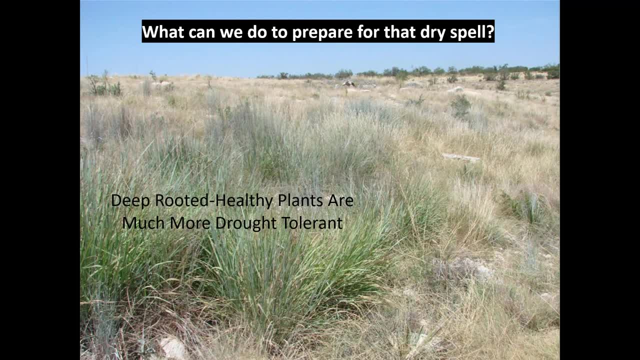 little blue stem and look at the brown other perennial grasses, High grasses or short grasses that are browned out due to the dry weather. Those deep-rooted plants still have that green. That is exciting to see. Now then warm season and cool season. 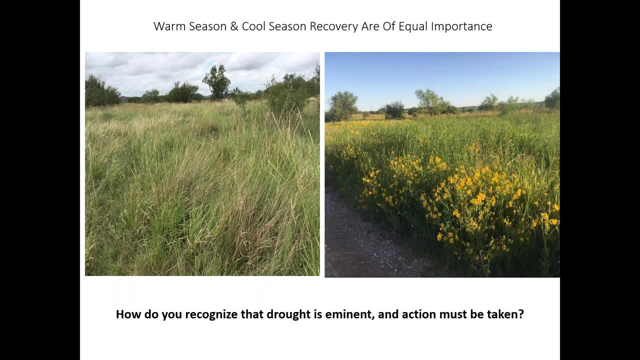 we hear about season-long deferment or deferment during the growing season. My first question is: what growing season are we talking about? We're very fortunate in the area that our ranch, my son and I have warm season and cool season growth. 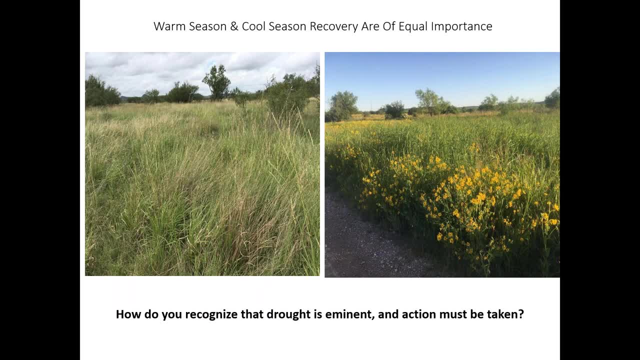 Over on the left you've got side-oast grama, Texas cupgrass, really dense coverage, None of the tall grasses, but it's really good, excellent condition. Over on the right we've got Engelmann daisy. 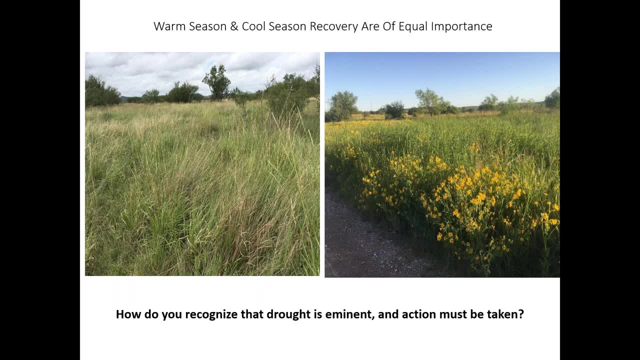 which is a perennial thorn, very palatable, a large reef system and Canada wild rye. I'm beginning to think Canada wild rye, with our grazed-rest program, may be the most profitable. It's one of the most valuable cool season grass we have. 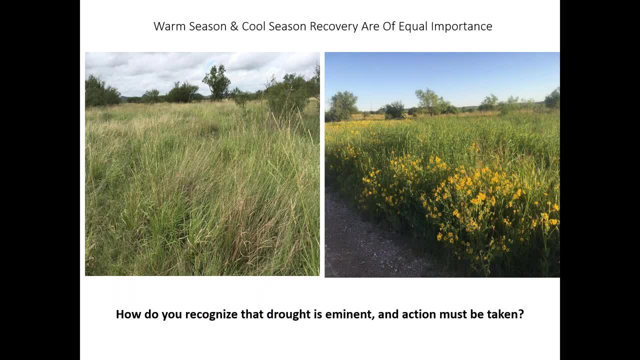 Now our grazing program is built around a single herd long rest 250 to 300 days regimen, utilizing traditional, already in-place pastures. No wagon wheels, just take the pastures that are on the place when we take it on and make them work in our grazing program. 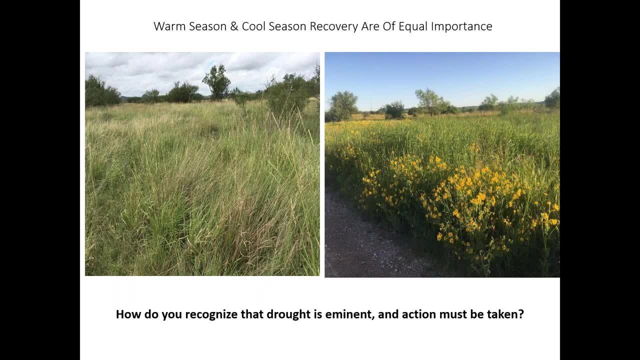 More pastures can be added at a later time. Finances dictate Going full bore, in my opinion, moving to a multi-paddock, high-intensity, low-frequency mob grazing program- and some producers are extremely successful at that, but I don't believe that the new grazer 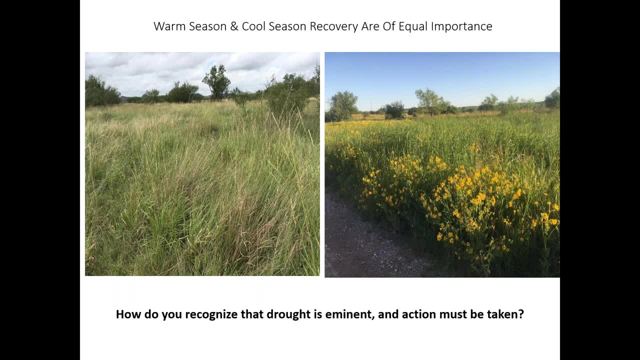 that's interested in moving to a single herd program. he'd better stay away from that until he has the experience to deal with the issues that it can create. The main thing is get started in some sort of rest program, Initiating a simpler, effective program. then you can expand. 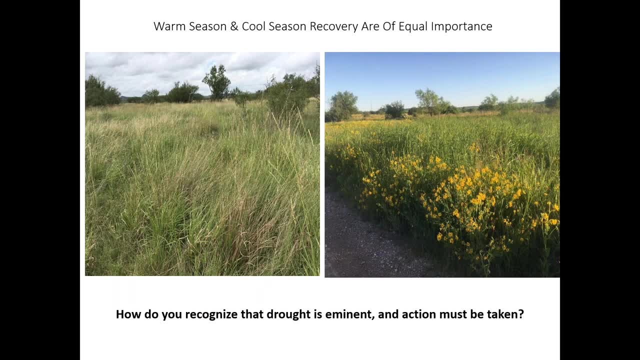 as you become more comfortable in the process. Duration of time spent in a grazing pasture depends on the number of pastures, size of the pasture and condition of each individual pasture, But of great importance, upon moving out of a pasture, everything's being rested. 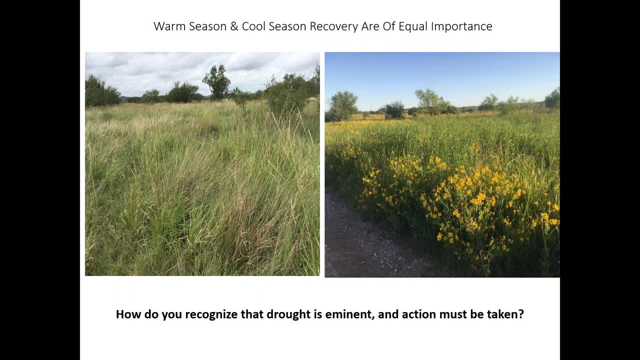 but that one pasture we moved out of. we ask ourselves a question: If it does not come, appreciate we'll run. But if there's no rain and growth of our grass before our next time grazing of that pasture, are there enough quality grazeable plants? 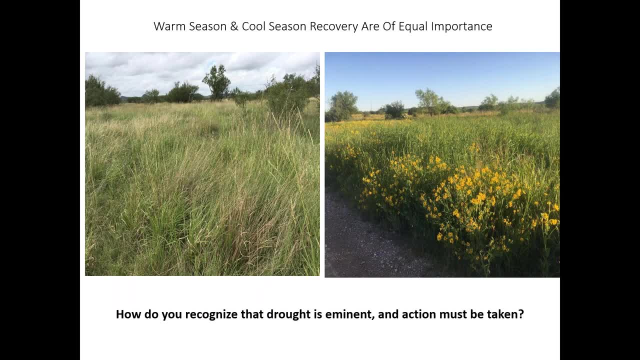 to graze that pasture again? Very important question. If the answer is no, the caution flag goes up When we move from the next grazed pasture. if the same answer is no time to move into our drought management plant, It may be a long time before we come back. 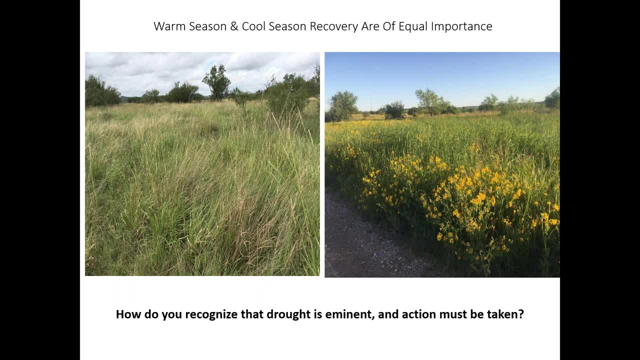 but we need to start taking the possibilities, the availability of drought, very seriously. We've never been able to use rainfall as a consistent indicator of an approaching drought. Yeah, you get the feel, but observing those pastures is the most important thing I feel that we can do. 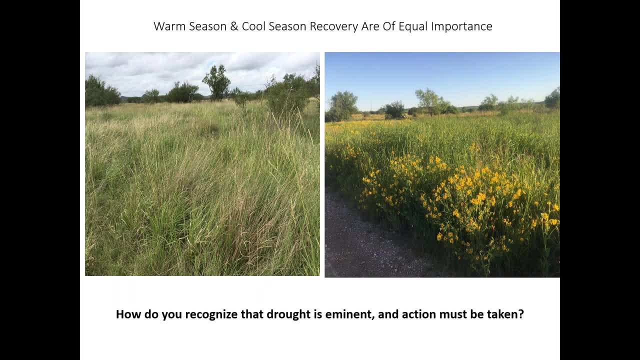 After initiating the grazing program we've chosen, which is that single herd program each preceding year, the rangeland is known to be more resilient to dry spells. In other words, the better it gets, the faster it gets better, And that's since we went to that long rest period. 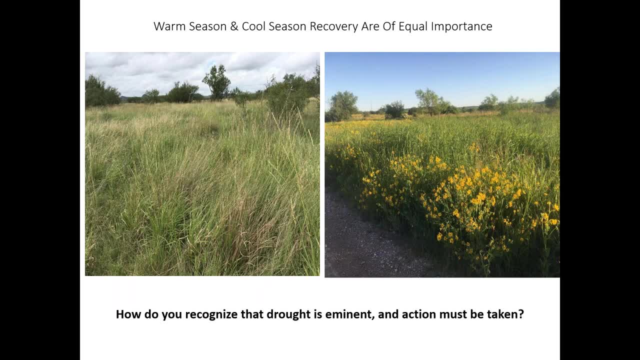 we were seeing that every year it's getting better. We're finding those smaller rain amounts are more effective than in the past and that those deeper rooted grasses, including Indian grass, big blue switchgrass, are among the last to brown out. 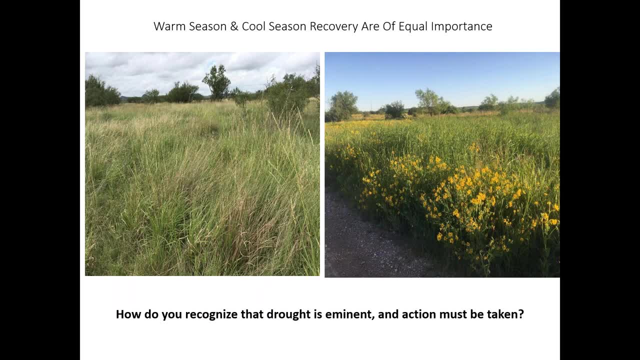 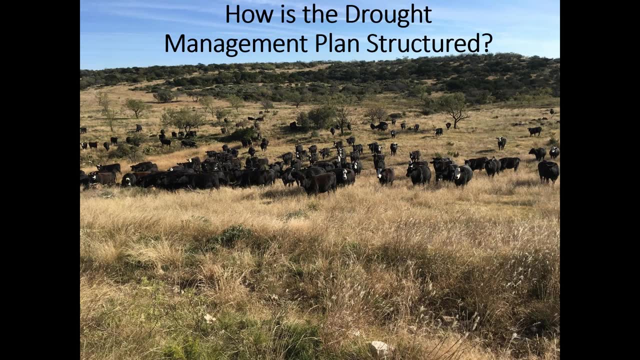 as that prior picture showed us. Now then, how is the drought management plan structured? Hopefully the plan will be initiated well enough in advance that we will not be in a panic mode. That's one reason for the observation of the pastures that we do. 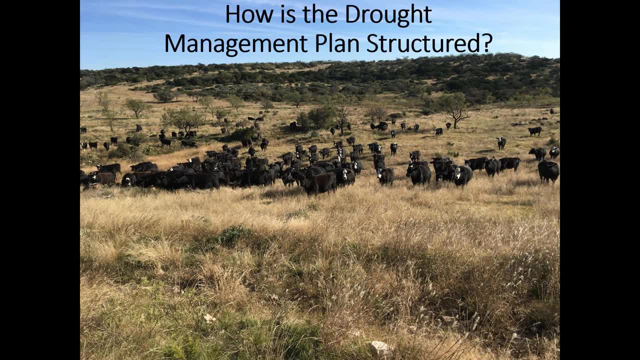 A slow progression is important. If it does come appreciable effective rainfall, the plan can be reversed without jeopardizing the factory. and the factory is the cow You sell. all the cows being a cow-calf operation, we're no longer in production. 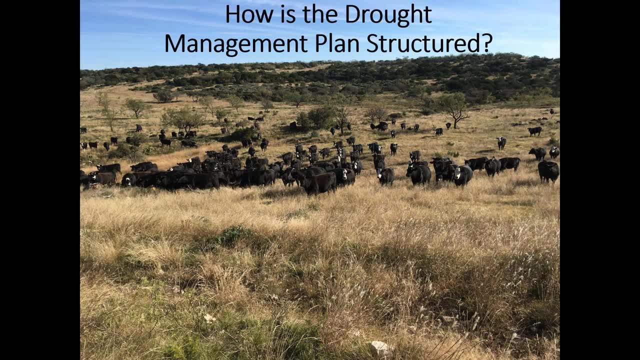 Each individual producer needs to develop his own plan, as there are so many variables depending on the location, goals of the operation, labor availability, numerous other influences on each particular ranching operation. Listed below are some of the options that we utilize. 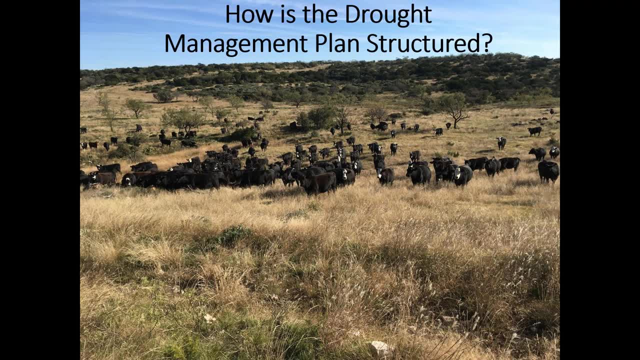 and some we prefer not to use. Once again, it's up to the individual which ones will work for him. Many options are available. Don't limit your operation to what I've listed here. First, early weaning calves. Second, reducing cow numbers. 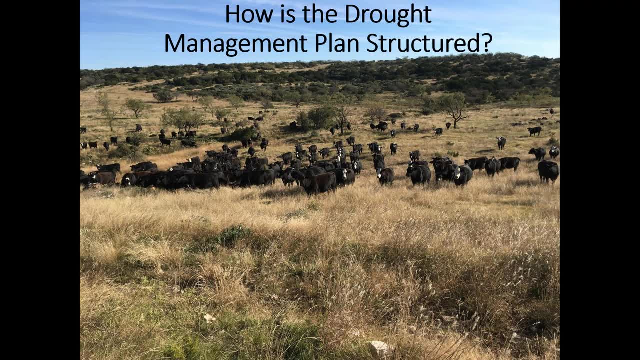 Open cows first, Perhaps using sonograms. Do your pregnancy testing at an earlier stage. Late bred cows come next. older cows next, Though we always try to keep our younger cows, as they will be the ones that are productive, well into the next of the good times. 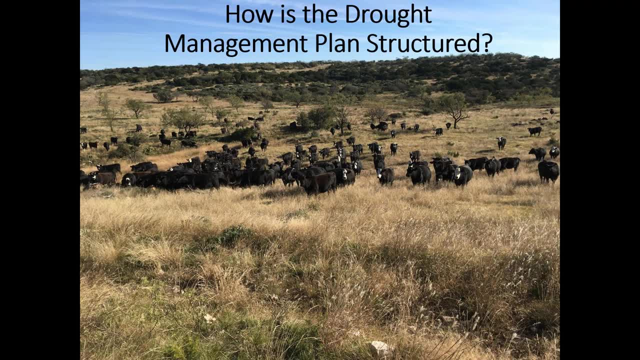 We generally try to raise our own replacements as they, as they grow, are acclimated to our operation, both environmentally and socially. By socially I mean they're adapted to how we handle them, moving from pasture to pasture. We can, you can, bring in outside stock, but our cattle are adapted to our program and I like 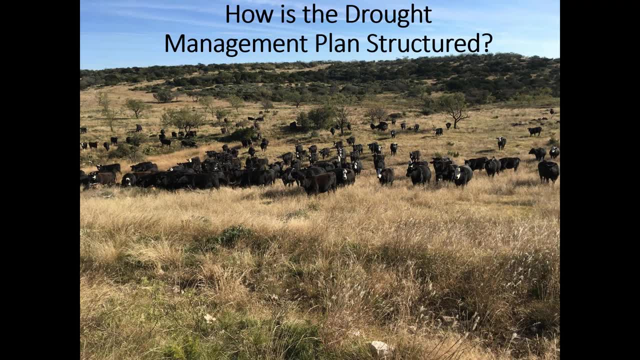 staying with them. For producers, next first, last- there's always room for improvement in the cow herd During the expansion of the herd, which is generally the case. since we implemented our single herd graze rest program, culling tends to be limited as we would rather own. 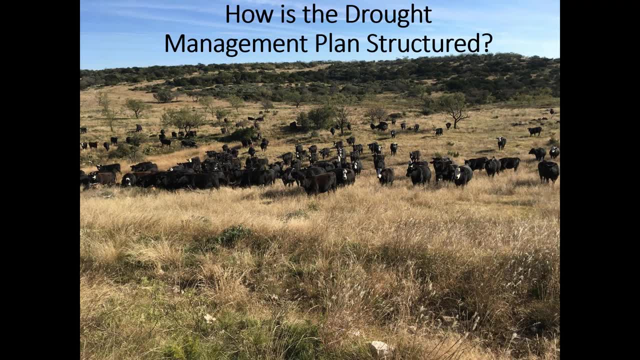 some of our own culls than buying someone else's culls. Limited supplementing supplemental feeding can be productive for the short term, in particular, approaching breeding season. Now we have built into our operation around never feeding mature calves winter or warm season. This has been a very positive and 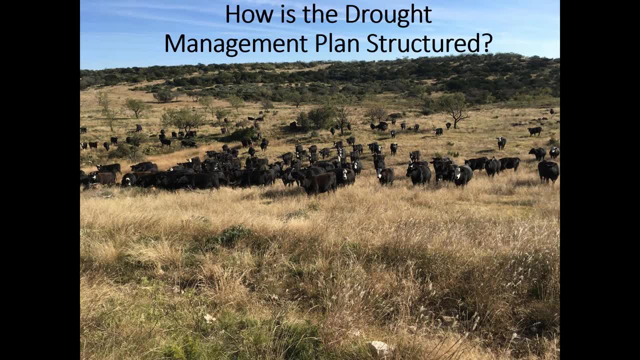 consistently profitable for our operation. Heavy supplemental feeding is not an option for our operation, perhaps on a very short-term basis, until marketing can be initiated. However, if you have to go to this heavy feeding, even for marketing, it can be a good idea to buy cereals during tax break, in the winter or in the cold week. 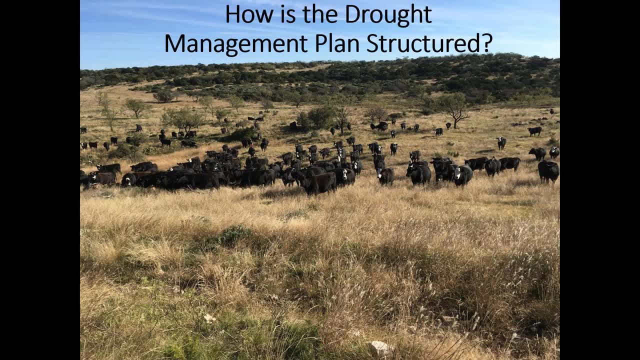 There are also ошибcance- nutritional Cut-off and manufacturer-acc 분들은 mind, and we've also collect the personnel during that time. However, at that time, the care care secret is to consider Titus At another stage. each and everyルクings can demand or more than can be. 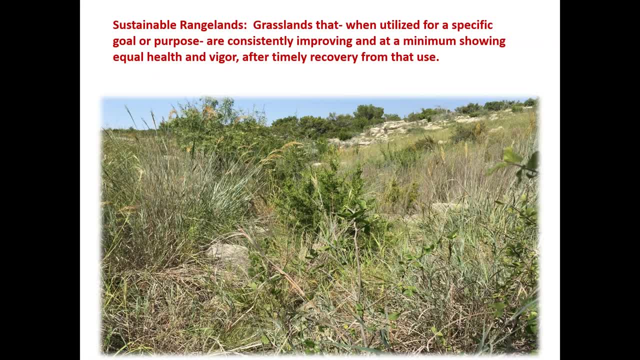 different food crops, leading to pollution and severeaktuings of the crops themselves. The first and last option of any producer that is wanting to create and maintain a consistently profitable operation, even in drought situations, should be a grazing management program that utilizes sustainable rangelands. 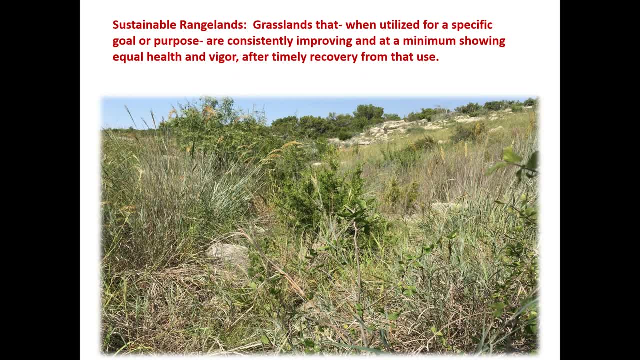 My definition of sustainable rangelands. first I want- the picture is in some very rocky, not really steep but good elevation change. Here we have Indian grass, big blue, little blue white honeysuckle. that just appeared after we initiated that grazing program. 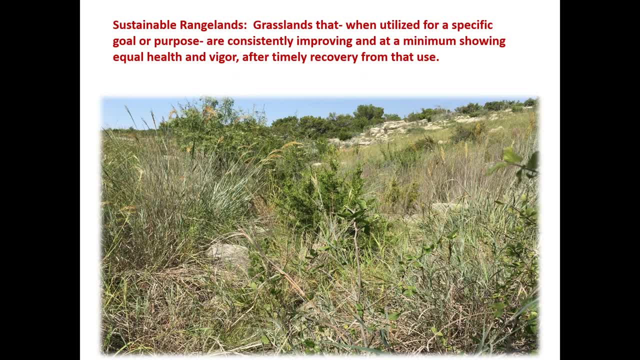 Very important: Sustainable rangelands, grasslands that, when utilized for a specific goal or purpose- ranching in our case- are consistently improving and, at a minimum, showing equal health and vigor after timely recovery from that use. We have to give it that recovery time. 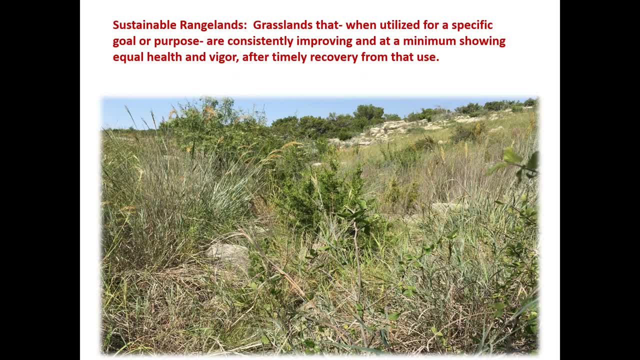 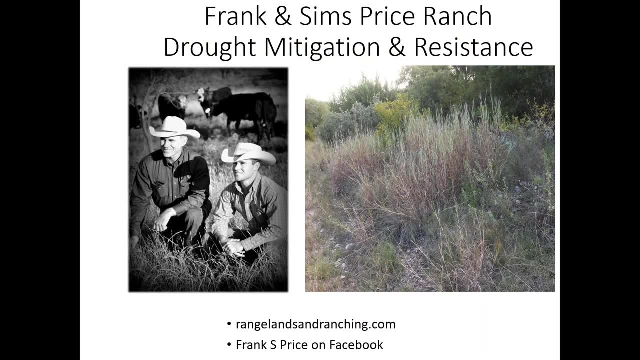 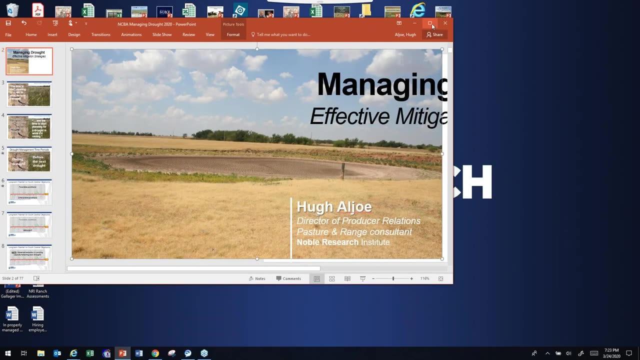 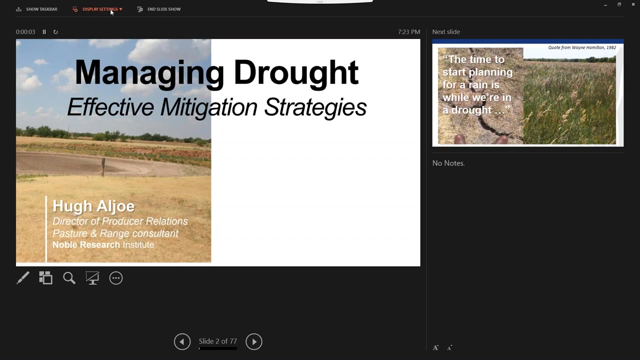 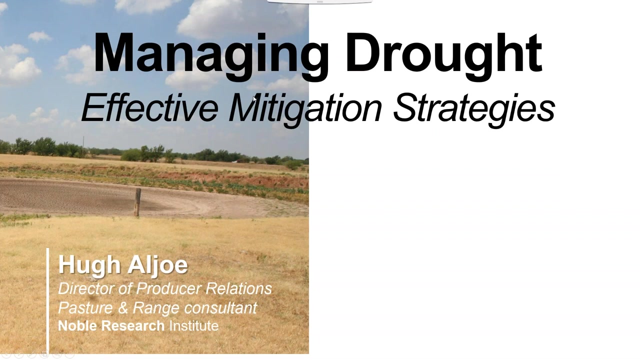 Thank you very much for hearing me and, Hugh, I'm going to hand it over to you, All right. Well, thank you, Frank, And I appreciate being a part of the program today. I also appreciate Joe's introduction and can really appreciate the words of both these. 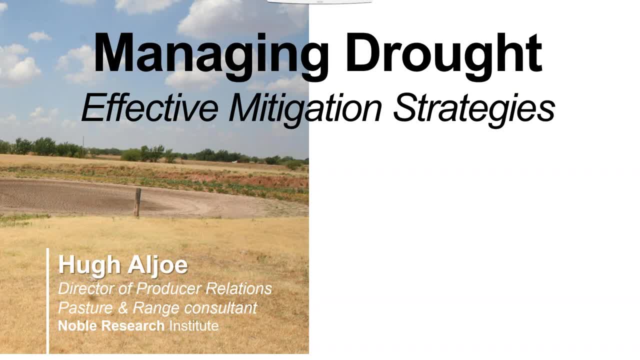 producers that are in part of the western part of the US And most of what I've experienced here in the Southern Great Plains at Noble Research Institute as director of producer relations and a pasture and range consultant is not quite as arid, not quite as risky of management as the other producers. 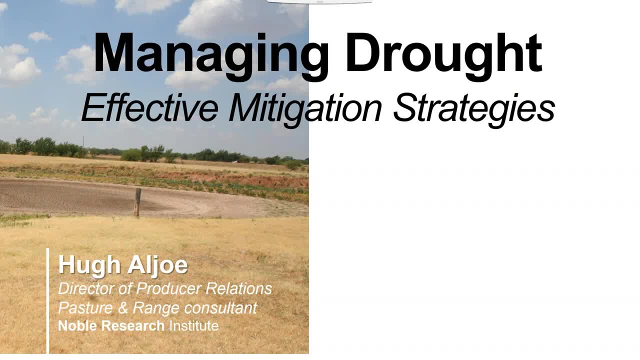 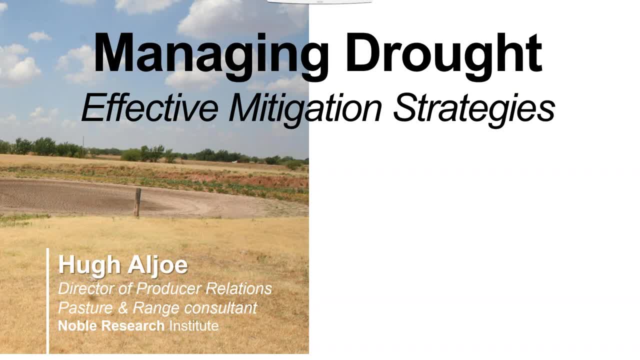 Thank you, Thank you, And so we're going to finish up with a quick, quick presentation, And I'll have Frank submit it as these two gentlemen face, or the next gentleman here in just a few minutes, Scott Stone. But what I will share with some of the some of the highlights is we work with producers. 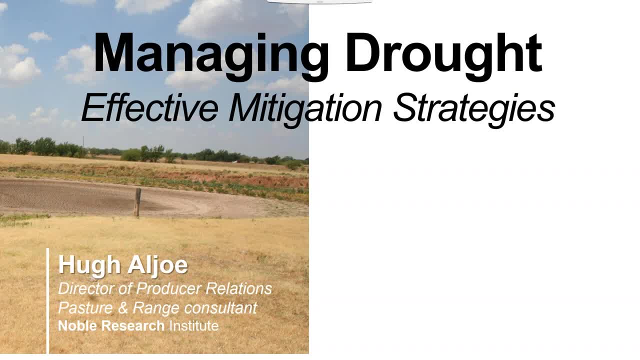 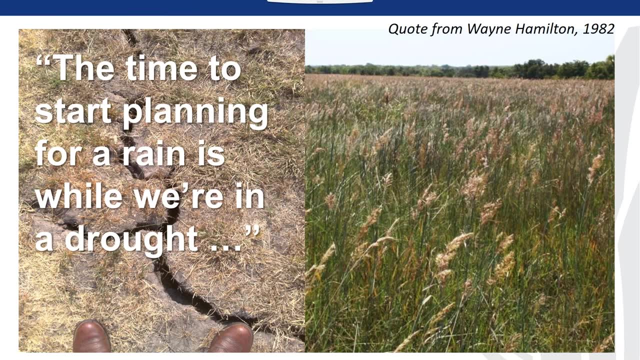 here in this part of the world in managing effective strategies toward managing the drought. You know, back in college one of the wisest sayings that I accumulated from Mr Wayne Hamilton, who was one of one of our range professors, is the time to start planning. 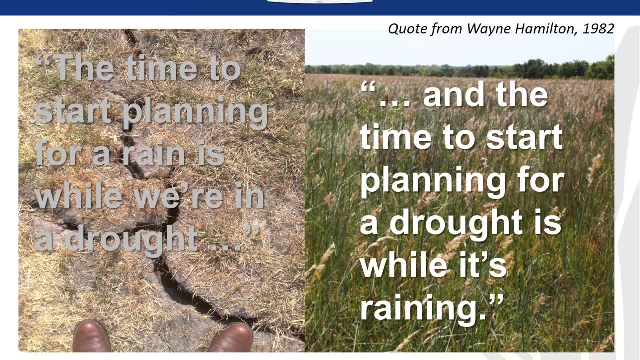 rain is while we're in a drought, and the time to start planning for a drought is in is while it's raining, and we think about that, you know. the take-home message is is that we're always need to be planning for the seasons ahead and if 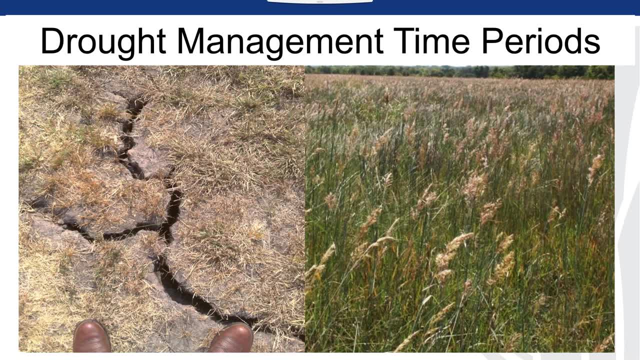 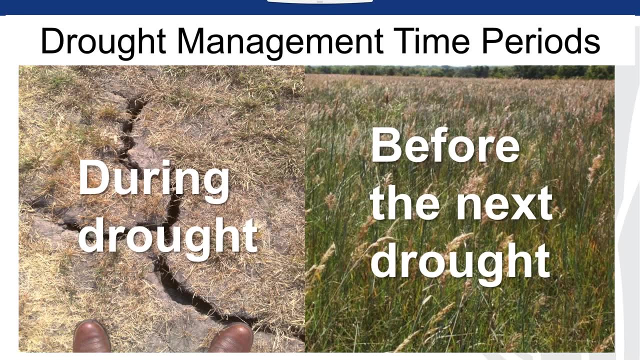 we look at drought management, there's two time periods that we're always operating within the period: the period during drought as well as the period before the next drought. you know, we have always got to be thinking ahead and knowing that even in favorable, favorable conditions, there is a drought. 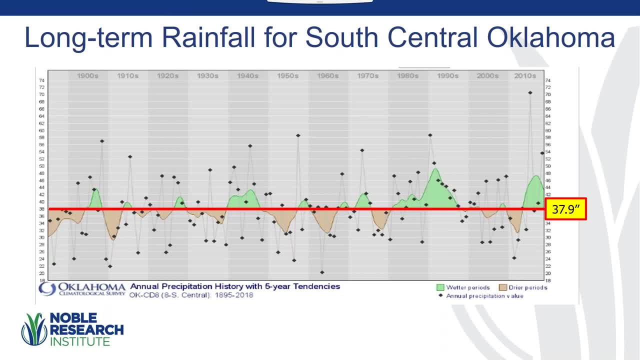 that's going to be looming ahead. if we just look at the long-term rainfall for South Central Oklahoma, where Ardmore is located, in NOVA Research Institute is located, we can see that over 125 years we've got a rainfall patterns that tends to show that we've got periods- excuse me, periods- of favorable conditions as well. 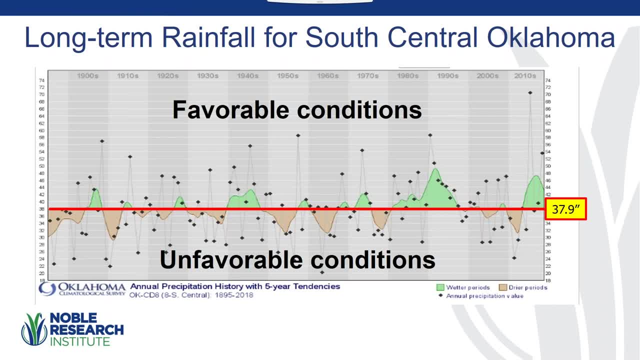 as periods of unfavorable conditions, and we note that these tend to last longer than normal, and we know that we're going to have a drought that's going to be last for a period of time once, followed by, followed by another. you know, the favorable conditions are going to be followed by unfavorable. where are we at? 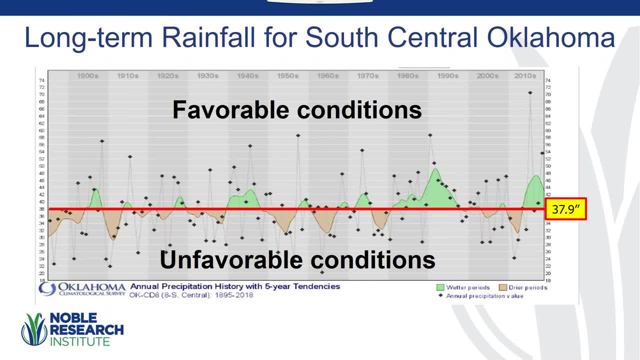 any given time, and as you move to the arid western part of the United States, we see that these conditions may be even more extreme as we look at at these of these periods of time. but where do you begin to operate? how do we begin to stock? how do we manage our pastures if we're really trying to provide for drought? 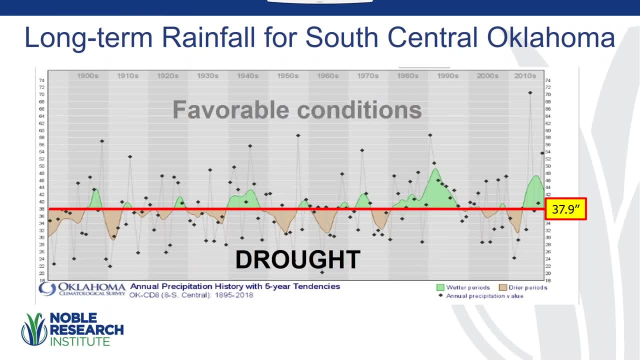 and the drought is real and one of the things that we've got to realize that, similar to what Frank was talking about, is that after every drought, there's been an observed reduction in carrying capacity through, you know, through those periods following, and we've also go back and you note the age of trees and 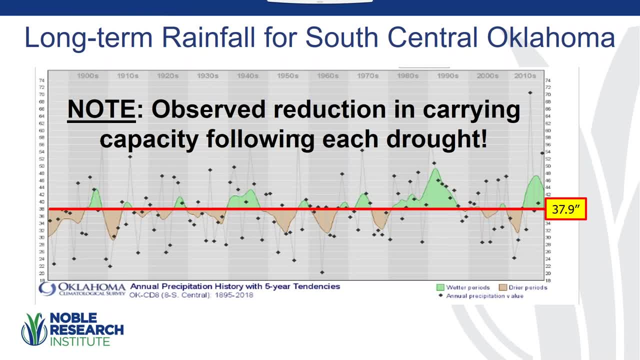 some of the shrubs that have appeared in areas that historically were never part of the natural floor, at least in these open space- and we're going to have to spaces, and we'll see that they have all appeared or begin growing sometime following one of these drought periods. so we have changed the flora through our 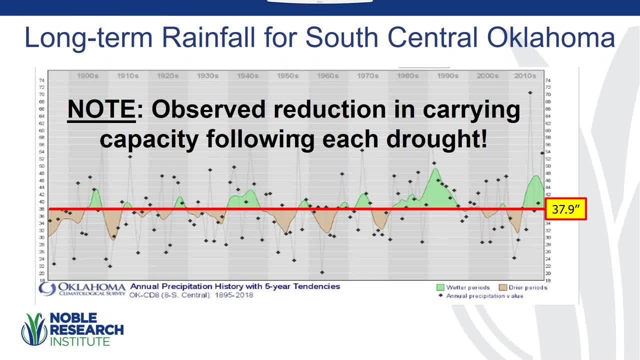 grazing management, or, in this case, the lack thereof, during these drought periods. so what can we do in managing our own ranches in order to secure greater resiliency within these pastures, so that, when drought does come, we're more likely to successfully manage through it and mitigate the effects of? 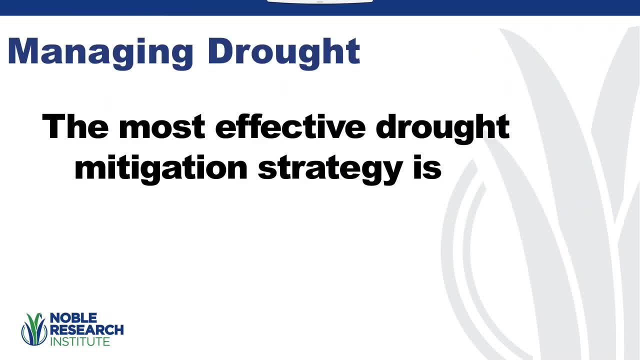 the resource itself. so we want to really begin talking about drought or managing drought, looking at what's the most effective mitigation strategy for drought- and really it is pre-emptive management, similar what Frank was just talking about: some of the planning that he does and the producers that we've worked with. 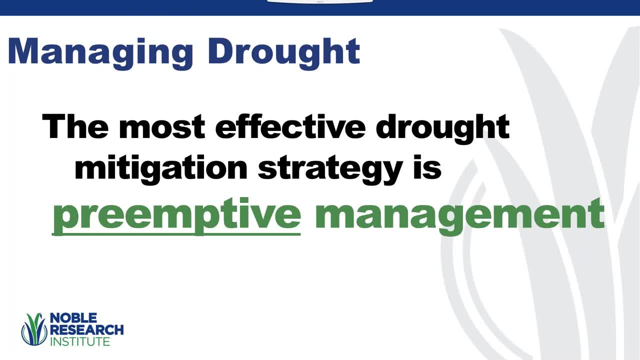 it have been most successfully. what they've done is they've done a lot of planning, and they've done a lot of planning for a long time now, and so what they do prior to the drought is lend themselves to the opportunity to successfully navigate through these drought conditions, and they're usually falling into a couple of three areas. 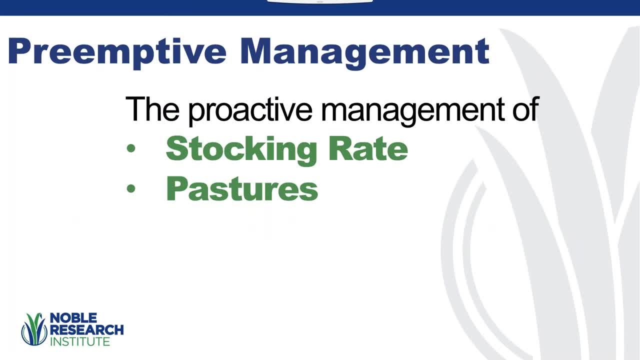 that they're always prepared for: the first, they proactively manage stocking rate and second, at any given time, there's always a plan in place. and in order to prepare for the drought, they're also developing contingency plans, or drought plans as we would know them. so that's what we're going to talk about. 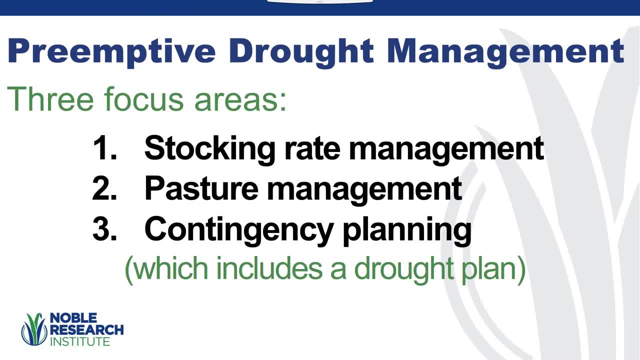 pasture management and contingency planning and show you what a prescribed drought plan might look like for a producer which, as Frank pointed out, you have to adapt these things to your own operation and situation, but this will give you a template at least to step through and consider as you begin. 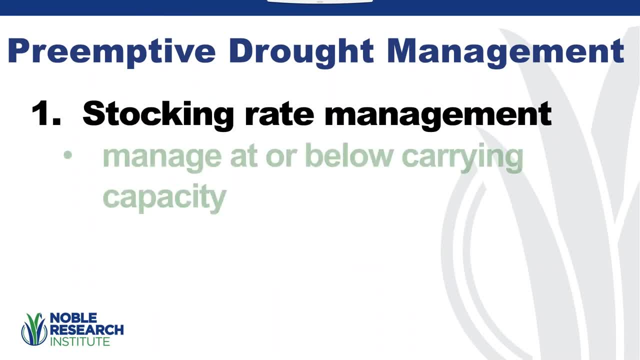 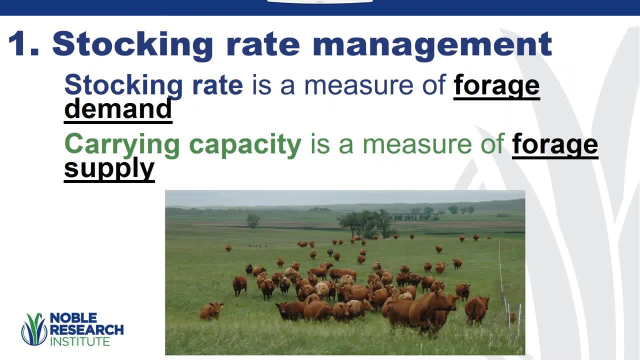 planning in the into the future. so stocking rate management. now what we really would like to do is manage at or below and below carrying capacity. we understand this producer stocking rate just the measure of forage demand. it's the number of animals that are out there at any given time and carrying 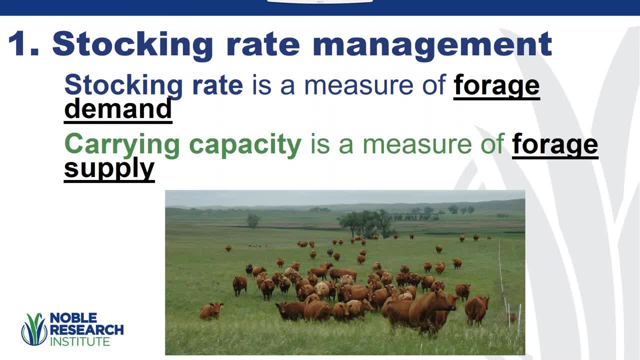 capacity is a measure of forage supply. that's the amount of forage that's been actually being produced and it changes and we know that it does. you, as a manager, have influenced directly over stocking rate at any given time. now, carrying capacity, that's a function of what you know, primarily whether moisture 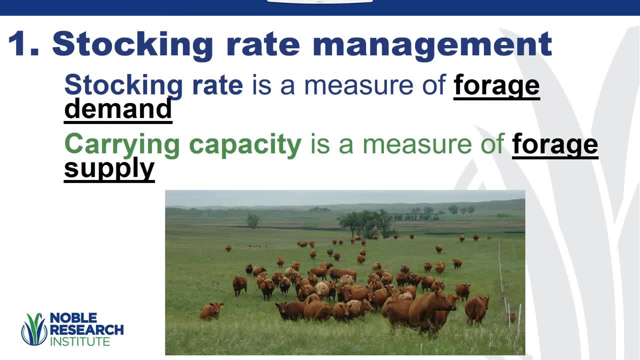 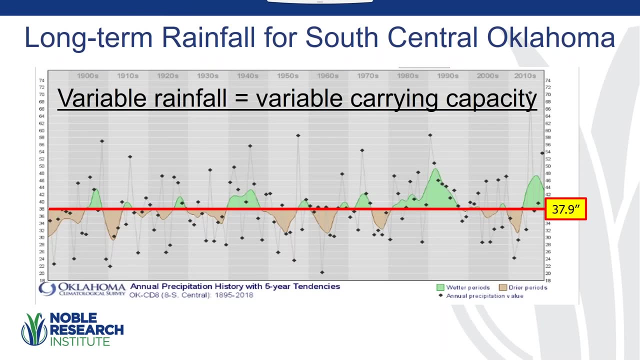 conditions and not to leave managers unfocused on our previous management, how well we've managed in the past. it's going to influence the amount of carrying capacity going forward. so if we look at just that long-term history of annual precipitation, we can easily see that variable rainfall is going to equate to variable carrying capacity and 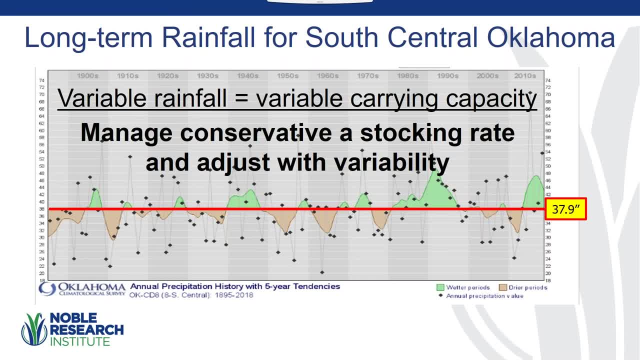 what we've really got to do as managers is always understand that we're trying to manage at a conservative, conservative stocking rate and adjust with this variability that we see, but in order to be able to, just we've got to manage somewhat below what we would consider. 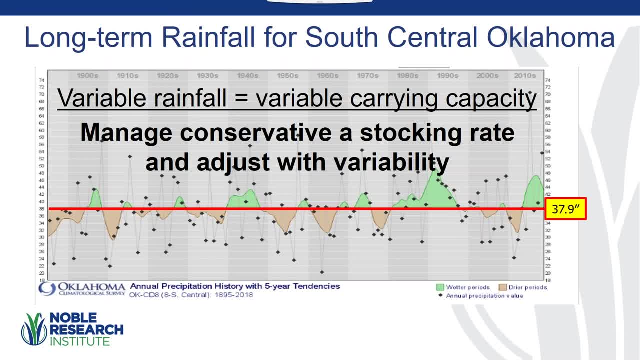 consider normal or average type of precipitation- and we all know there's no such thing as is average precipitation- but what type of safety net should we even be planning for so that gives us the resiliency necessary in order to be better managers of the land resources? that were accountable for the next part. 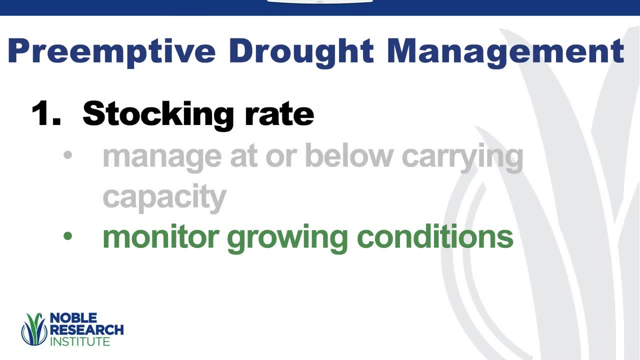 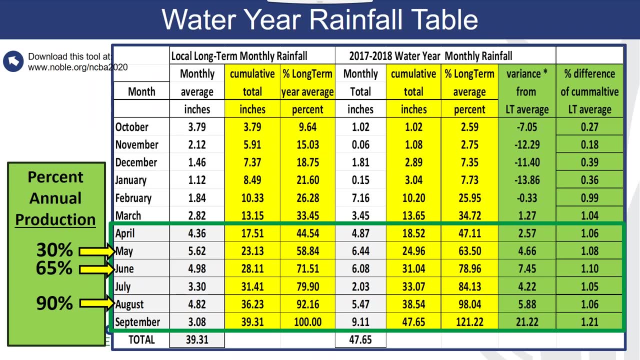 of it. we need to look at it, just monitoring growing conditions in order to to manage that carry capacity or the stocking rate with the carrying capacity, we need to understand what the growing conditions look like. where are you at at your property? one of the tools that we like to recommend here at noble is is: 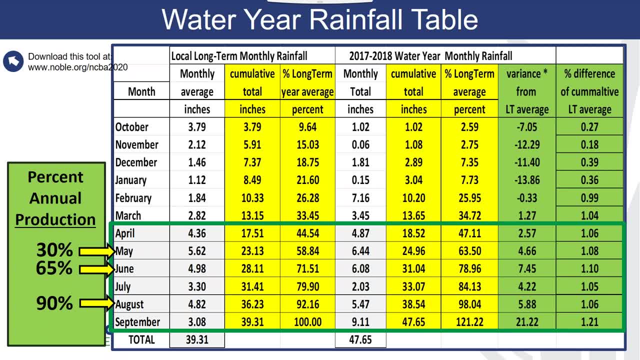 water your table. you know, typically in most part of the United States, when we get to our about October, most of the growing season is complete and, with that being the case, most of the water recharge into the soil is going to begin sometime in the cool season months as we move toward spring, as indicated by 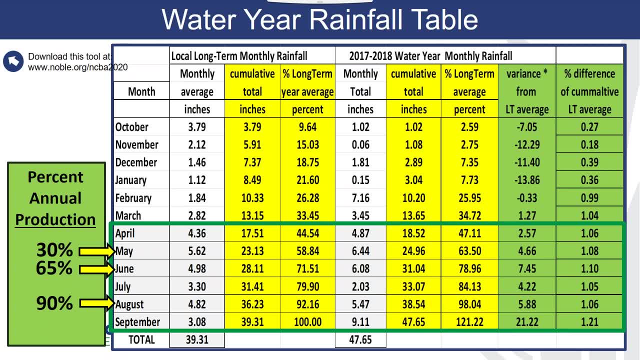 that green box, we begin to want to build up a certain amount of precipitation or moisture within the soil and if we relate it to precipitation itself. but we should expect somewhere, at least in this southern Great Plains, about a third of our annual rainfall to occur on a water. 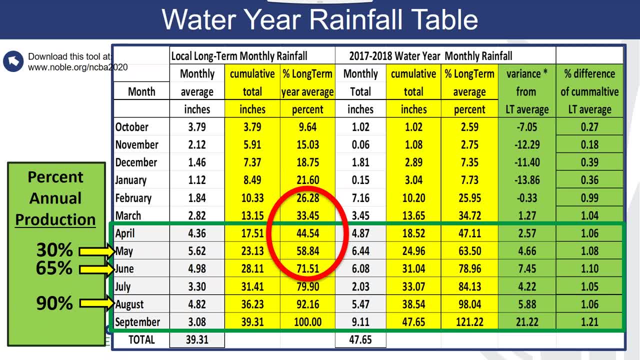 year by the 1st of April. if we don't have that at that point time, spring may be slow to get started. if we don't have about 45 to 50 percent of our water- your expect about 45 percent of our water, your weight- with some precipitation, by the first of May, we may not have much of a spring and certainly by the end of end of my. if we're not well on our way toward normal precipitation pattern or a favorable precipitation pattern, we will never acquire the potential of what we consider an average carrying capacity for for our land resource. so what we've really got to be looking at is over here on the right side of the screen: is that variance from the long-term average? we were you. where are you at any given time? it's 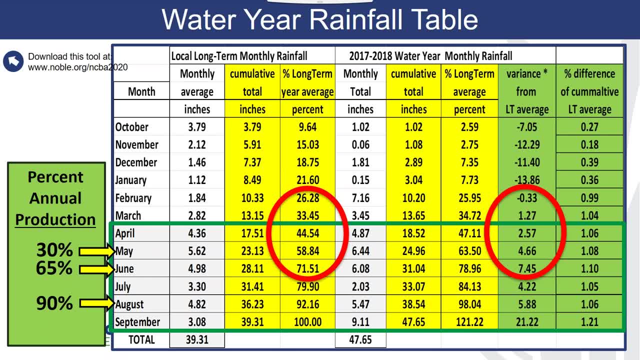 especially as we begin to enter the growing season and those early months in the growing season, Because with forages there's rarely what I call compensatory gain. There could be the unusual typhoon or hurricane that may saturate an area and we get a big boost. 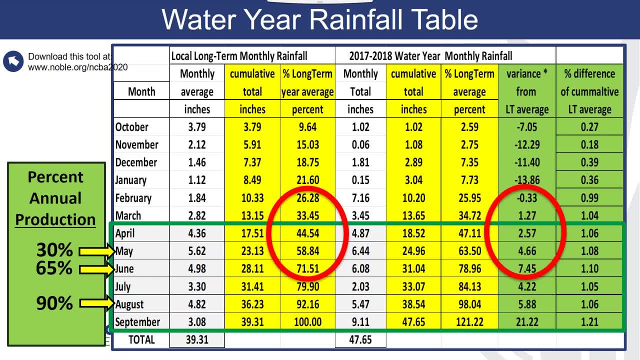 but typically what occurs early in the spring is what we've got to manage for through to the next growing season. So we've got to understand where we are. As just an indication, if your variance is a negative, 10 on this type of chart. 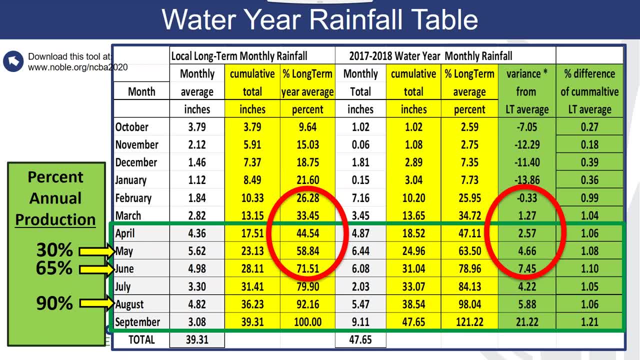 you'd probably ought to be implementing drought strategy sometime. if that's the case there in May, At 20%, it should already be in effect if it's a negative 20.. If you like this chart, you know there up on the left, 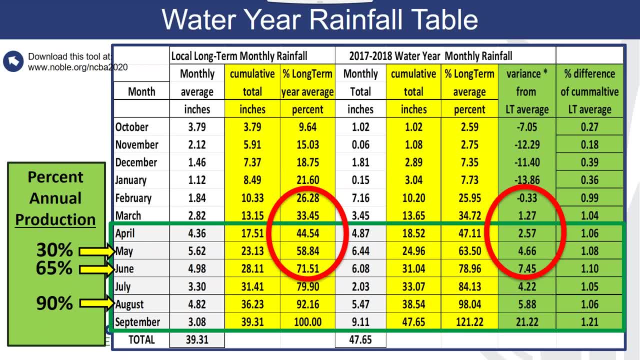 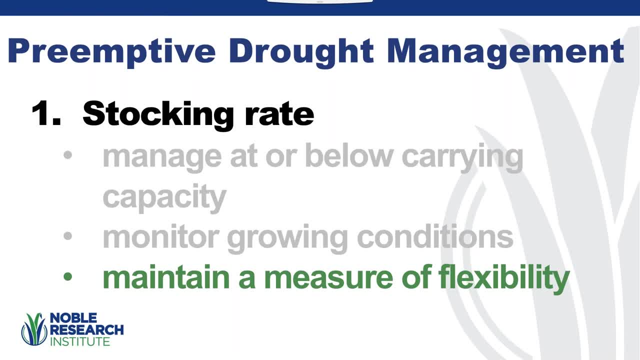 we can certainly be able to supply it to you just to look at what your ranch precipitation looks like against the long term for your region. The next part would just be maintain a measure of flexibility, You know, within the stocking rate. you know we can look at if we're conservatively stocked. 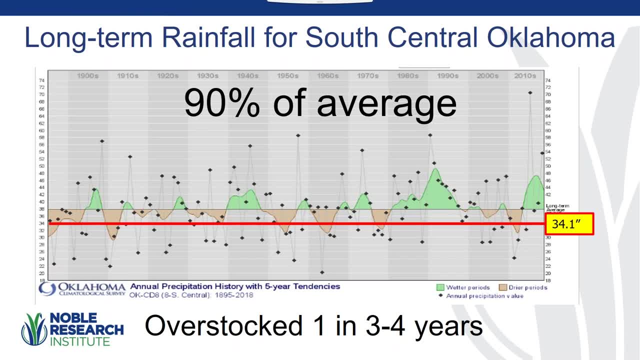 if we're about 10% below what we consider an average year, we'd only be stocked one in three to four years in this part of the country. If you're 20% below, it may be seven to eight years. You know, you lend yourself the opportunity. 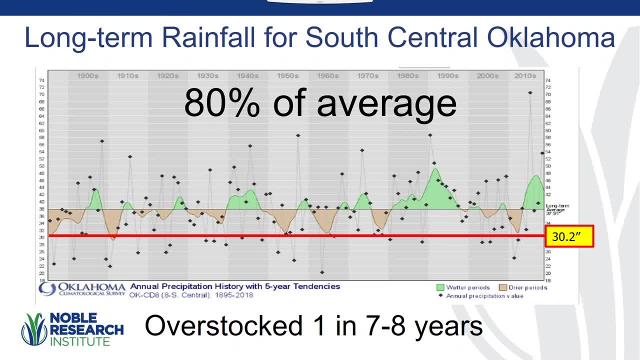 to get through a whole lot easier if we are conservatively stocked, And as you move more to the arid west that number may be on. your long-term fixed stocking rate may be considerably less than that. What you'd like to be able to do is be able to cover yourself. 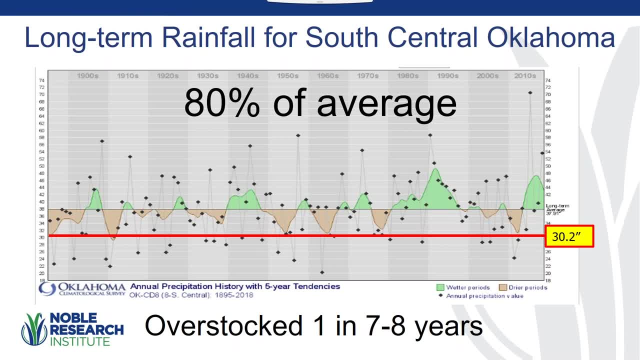 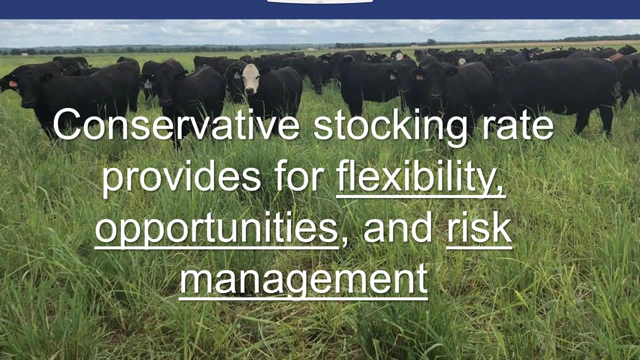 adequately 80% of the years, And then you just have to adjust your stocking rate accordingly And, in the good years, provide yourself opportunities for capturing some of the resources that might be made available. In short, conservative stocking rate provides for flexibility opportunities. 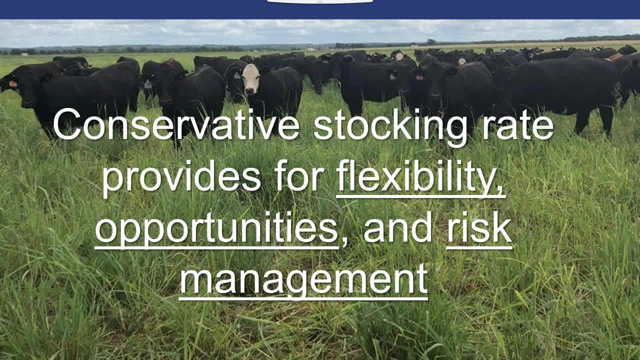 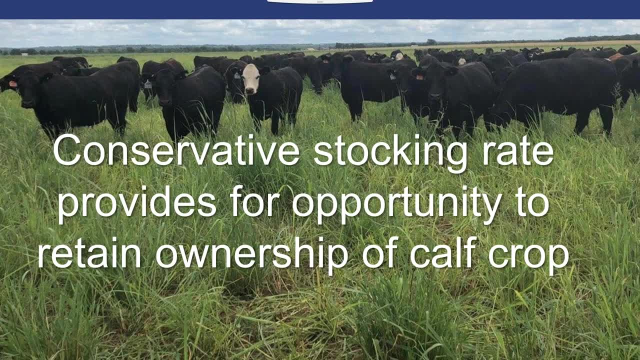 and additional risk management, As Frank had said. you know, the more he can store up and grow through the growing season, the greater the risk that he's going to have And that creates that risk when the drought actually occurs. Just as an example, a conservative stocking rate provides. 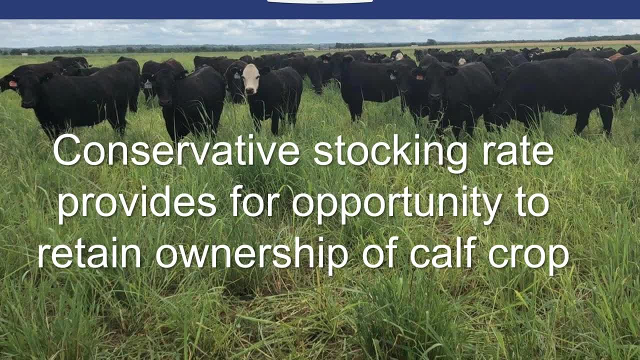 for opportunity to retain ownership of his calf crop. You know it may be all or a part, Depending on the conditions, you may be able to carry a portion of your calf crop into later in the season In this part of the world. typically what we see is 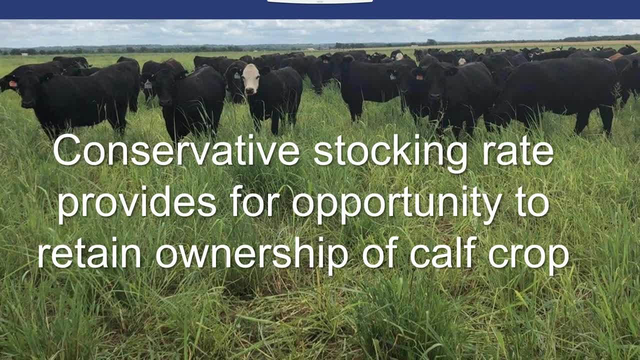 that if you're able to do that, you can actually increase income off of one calf crop over what you would have had at the beginning of the year. So that's a unique opportunity to not only manage your land resources, it also mitigates the risk of drought. 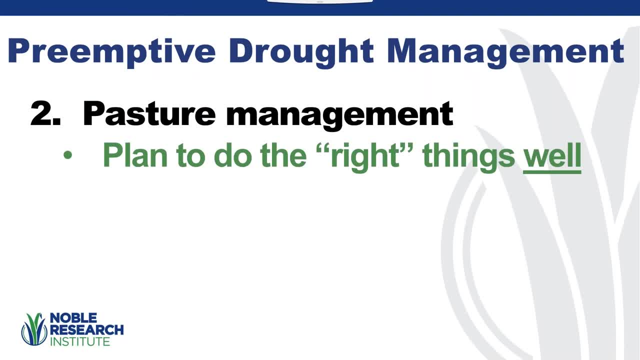 Next point we wanted to look at in preemptive drought management is the pasture management itself. You plan to do the right things. well, You know Frank's got a plan. I'm sure Scott's going to talk about his plan here in a minute. 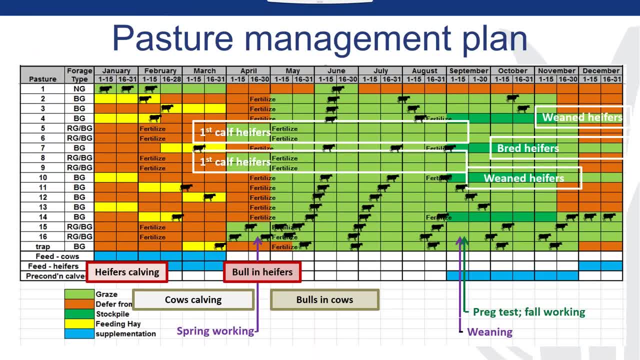 But what we've got to do is do the right things well, starting with the pastures You know. have a pasture management plan. Identify the key things that you need to do in order to manage the grazing resource first, and then overlay your livestock needs second. 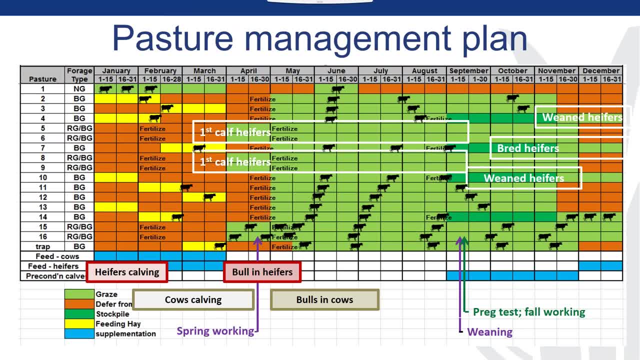 That's where a lot of producers probably fail to achieve is they're always trying to make their stocking rate or their pasture plan fit their livestock production. It should be just the opposite. We need to be managing our livestock to fit the grazing resource. 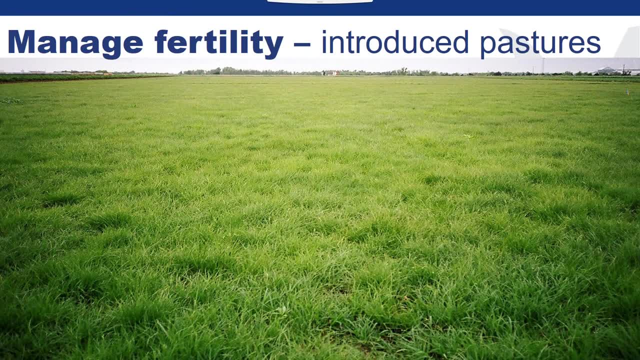 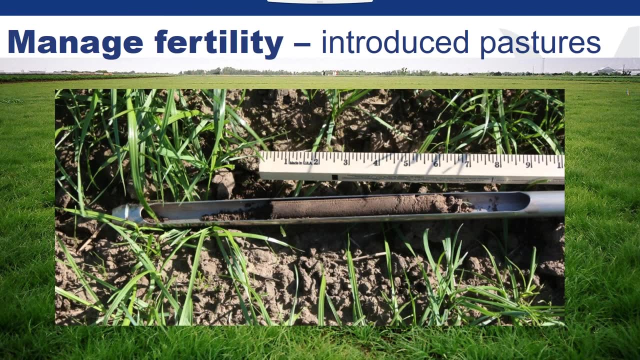 always trying to build up our pasture systems. If you have introduced pastures, as you get further into the eastern United States, you need to manage your fertility. You know be able to take the soil samples and actively manage those pastures that are contributing most to your stocking rates. 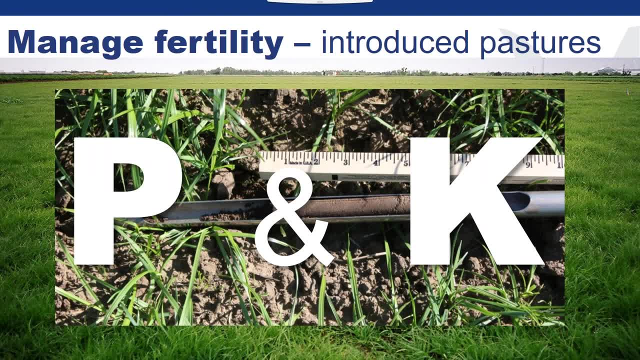 and pay particular attention to the phosphorus and potassium. These are the nutrients that supply the health to the entire plant system, the root structure, that benefit the roots themselves. So if we're not taking care of the roots below the ground, there's no way that we can be able to take proper care. 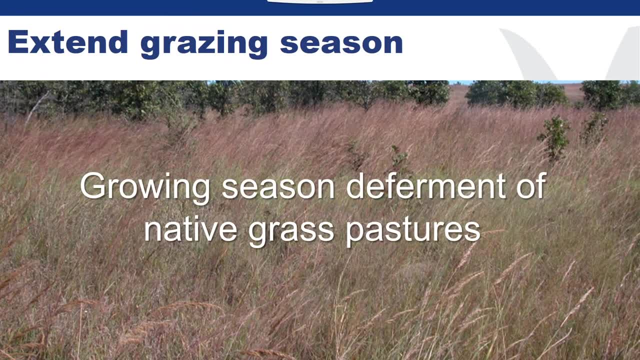 of the plants above ground In our native rain systems. we need to be trying to extend our grazing season. We want to make sure that we have growing season deferment of our native pastures At some point in time. Managing our rest and recovery periods are critical. 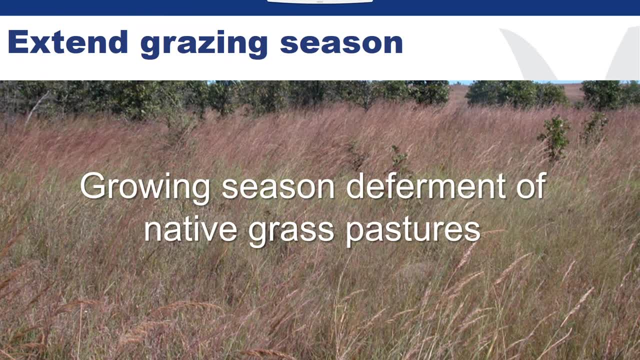 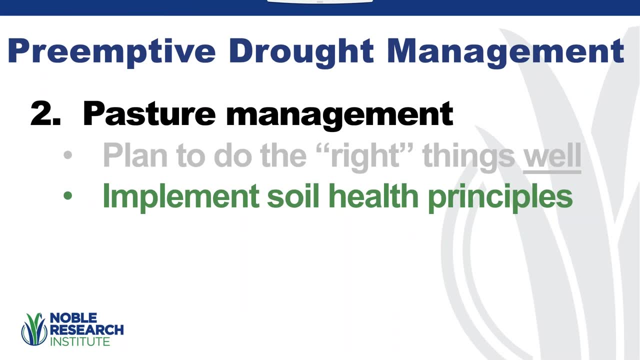 especially with these native systems that we expect to build resiliency in preparation for drought. Next point on pasture management is to implement our soil health principles. We know what they are, We've heard them over the years, But are we actually managing and applying those? 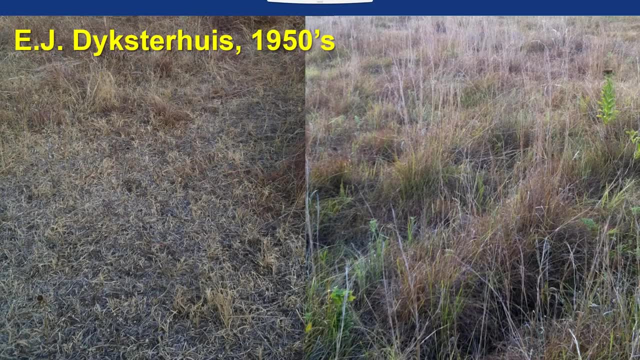 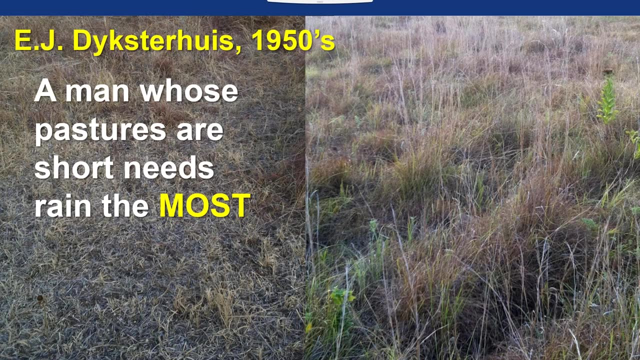 to our pasture systems, EJ Docksterhouse, back in the 50s. he's one of the fathers of range management. He made a statement: A man whose pastures are short needs the rain the most. A man whose pastures are in good shape makes the most. 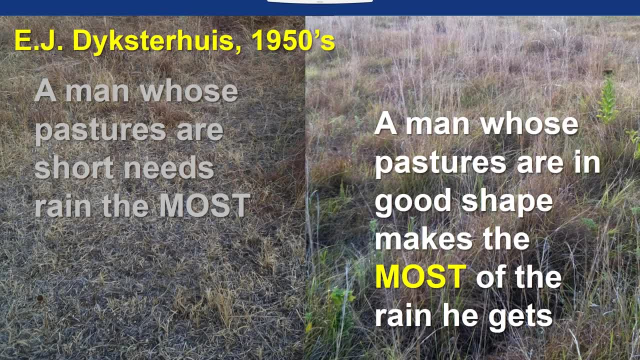 of the rain he gets. Just as Frank was saying, even a small amount of rain when you've got good conditioned pastures can absorb water and provide growth that pastures that are not in good shape can't do it. This is not only critical when you're during what I'd call. 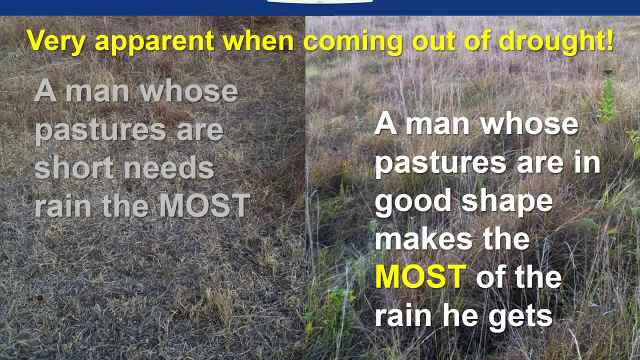 favorable conditions. it's extremely apparent when you're coming out of a drought. If you've managed your residuals properly, what occurs is that you'll have little or no lack of recovery and we may begin to rebuild the carrying capacities that we've lost following drought. 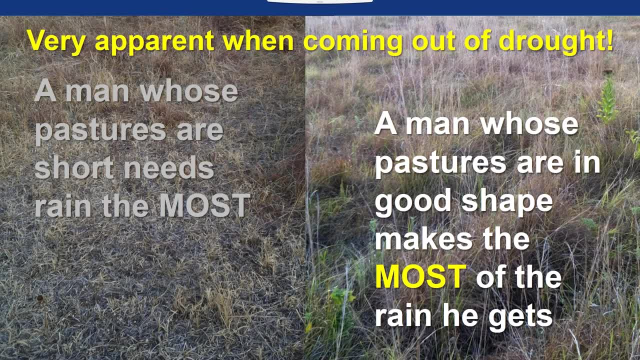 some of the droughts in the past. Just in the 2011 to 2012 drought, individuals that I know that actively managed their pastures, reduced their stocking rate and implemented drought plans early. once the drought was over, they actually saw a benefit: an increase in their preferred. 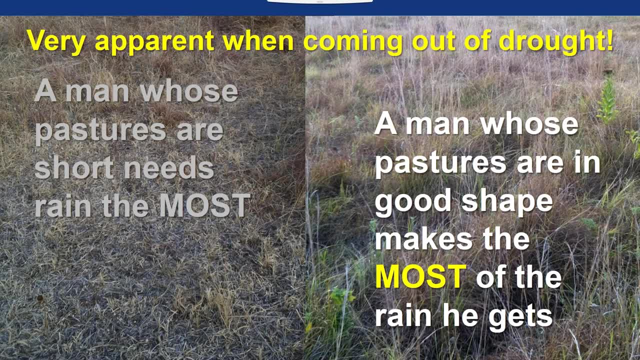 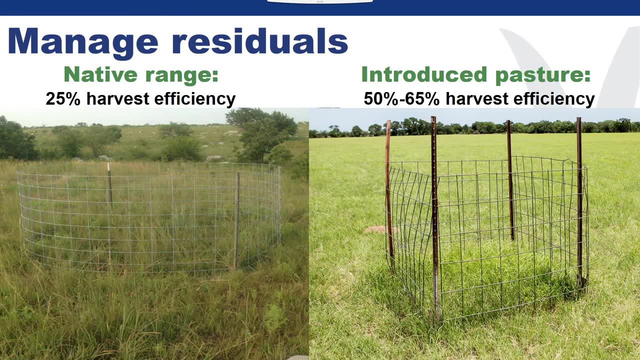 desirable tall grasses that they're actually trying to manage, for It's pretty exciting to see some of the recovery that can occur if your pastures are in good shape. So we've really got to be managing our residuals following what we know are recommended harvest efficiencies. 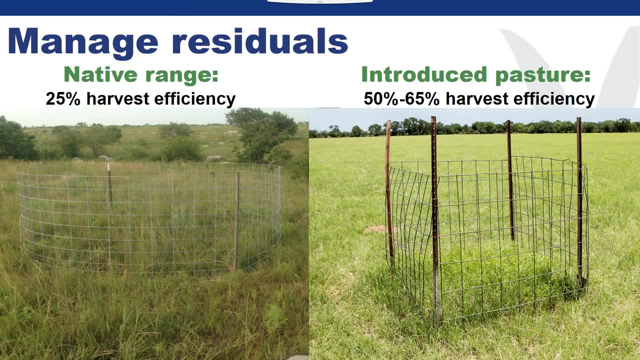 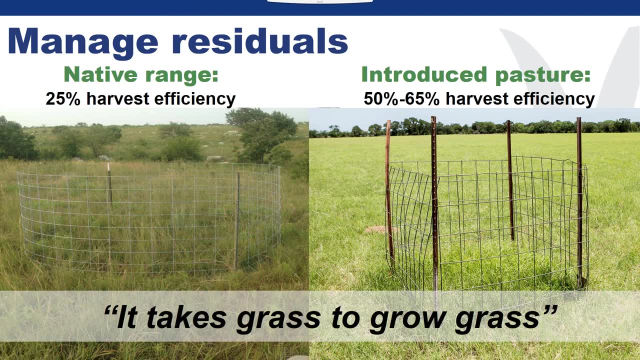 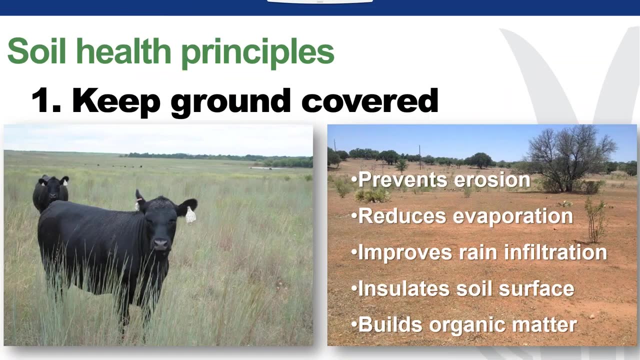 at all times, regardless of whether we're in drought or in favorable conditions. We've got to keep in mind it takes grass to grow grass. We need that grass there so when the moisture occurs, we can have the regrowth that's necessary in order to sustain our land and our systems. 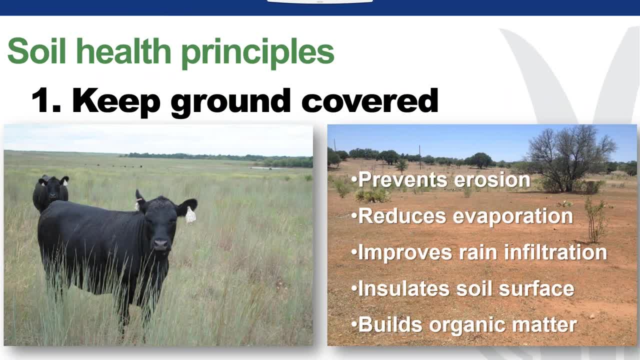 Just quickly, the soil health principle, just keeping the ground covered, Preventing the erosion, reducing evaporation, improving rain infiltration, insulating surface, The things that we know that are going to build the organic matter within the soil, which is the water holding capacity. 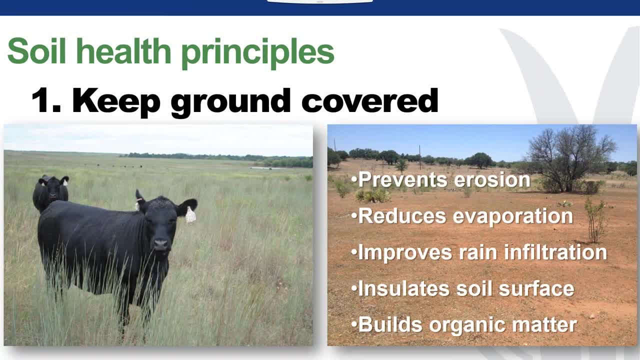 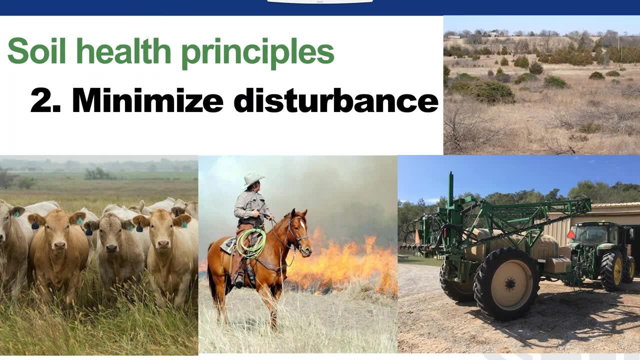 to a large degree in most soils is what we need to be focused for, and keeping the ground covered contributes to that. We need to minimize disturbance As much as possible, But in our grazing systems we're going to have some sort of disturbance. 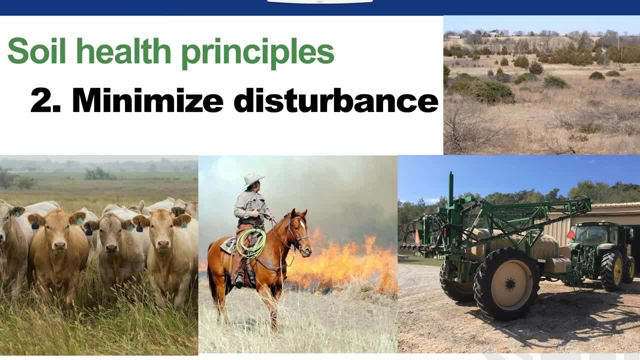 At least we're going to be grazing across these properties, hopefully in an intentional, managed focus, But we also may need to fire in our native rangeland systems in some locations, as well as periodic brushing and pasture control, So optimized disturbance may be a more accurate term. 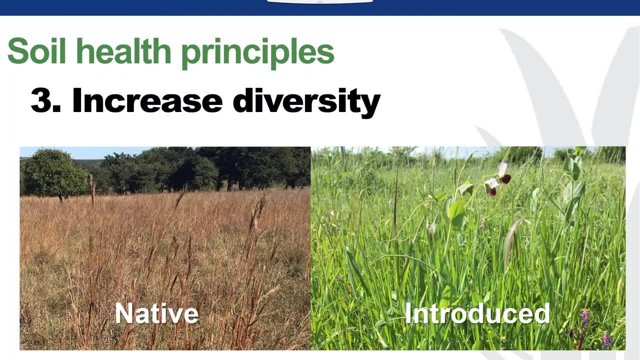 or a phrase when we begin to apply it to our grazing systems as it applies to soil health. With three, we need to increase diversity. In native country it ought to be relatively easy, but we need to make sure that we're getting the right type of forages throughout the seasons. 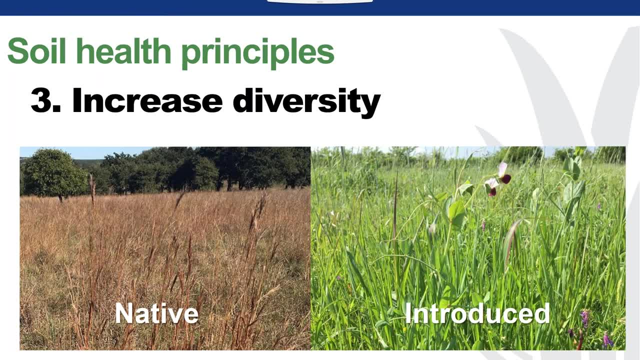 As Frank pointed out, sometimes the cool season grasses are just as important as the warm season grasses. depending on the season, Depending on our management, we can manipulate it, but we've got to be paying attention In the introduced systems. 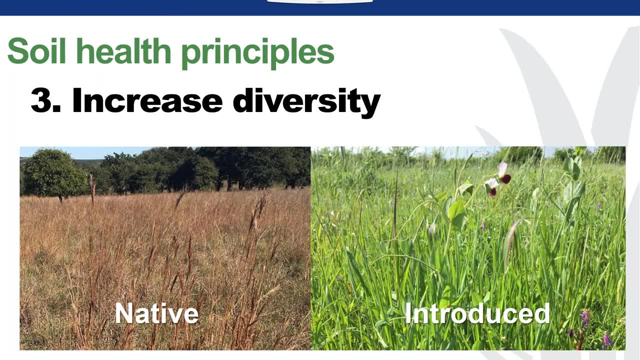 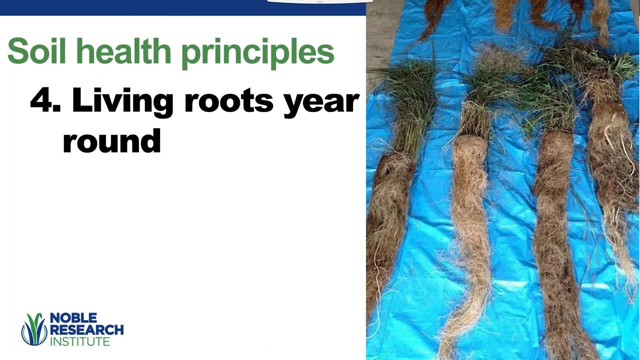 it's a little more difficult because we typically operate those in monocultures, But introductions of other forages into these systems can actually build our soil health. Keeping living roots in the soil primarily means we need to be managing our perennials. 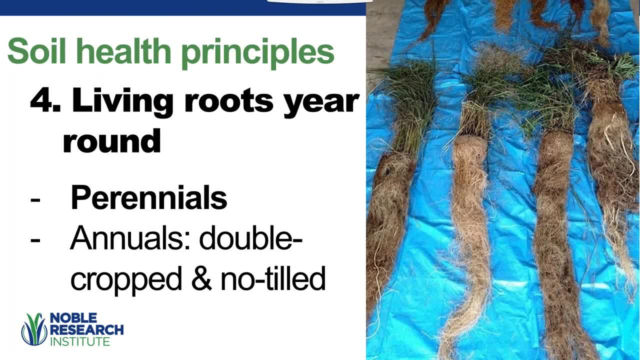 and managing them properly. If we're using annuals, they can add to our systems and we need to make sure that we're doing and managing those appropriately. that will be in complement to our perennial systems. Five: integrate grazing livestock And following what. 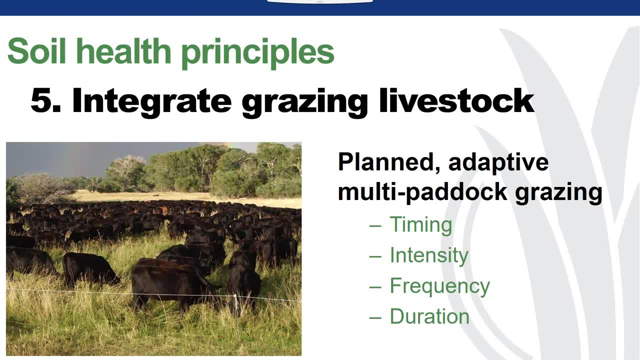 as Frank communicated, a planned, maybe an adaptive multi-pasture or paddock system where you, as a manager, have influence over timing, frequency, intensity and duration of grazing Timing, making sure that we're grazing at the right time and not before. 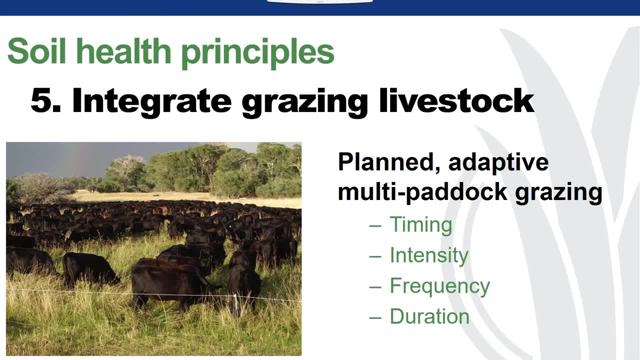 Being sure that we're have the right intensity during the times, the periods of time when the cattle are in the pastures, making sure that we're managing for adequate residuals and the frequency not coming back too soon, too frequently, and then looking at the duration. 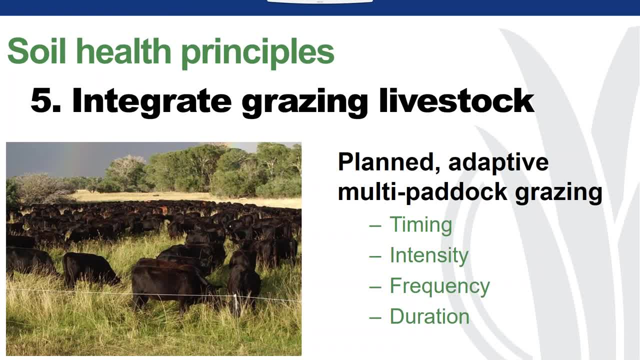 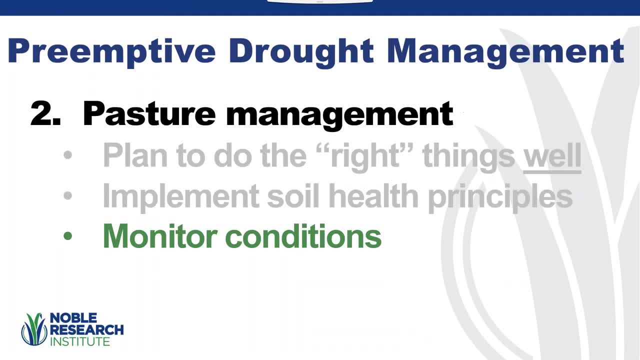 How long do we need to be in there, and all that depends on the different factors we're actually managing. But we as producers can be intentional about our grazing and have the positive outcomes. And then three just monitoring overall conditions Regionally and nationally. 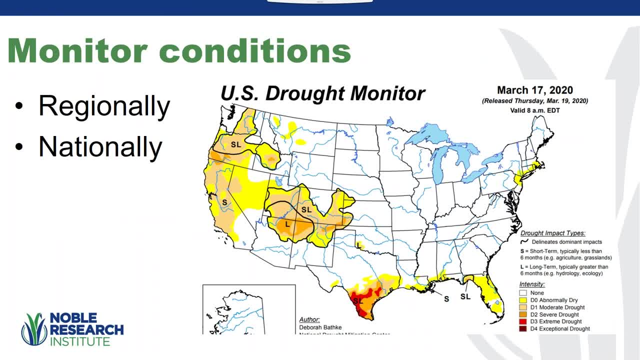 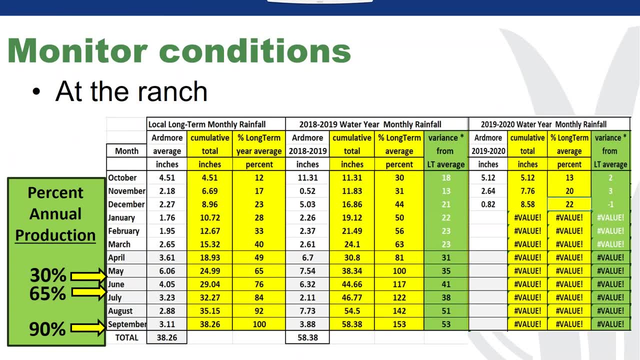 using tools like the drought monitor, knowing what's going around around the country and what's occurring near you. Using the tool, like you know, this water your table to better understand what the rainfall patterns are at your ranch over the long term. 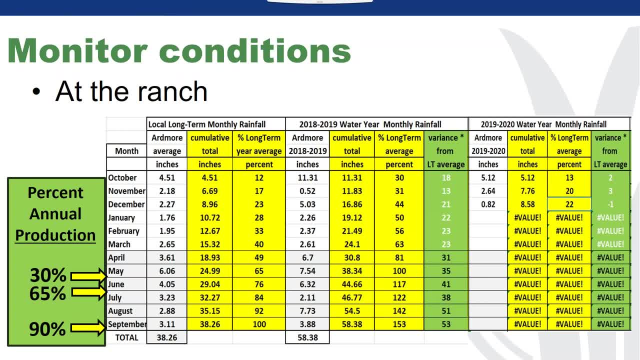 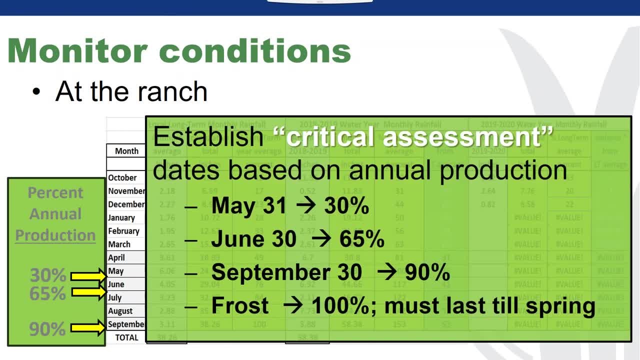 and how does that reflect to the growing conditions or your expected production each season And knowing what your critical assessment dates may need to be When you get into drought conditions, set timelines in front of you so that you know relative to your growing conditions. 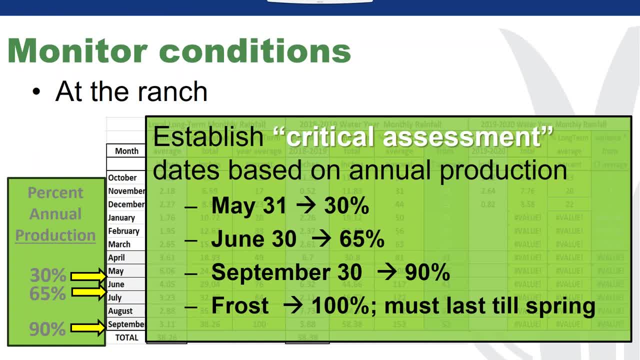 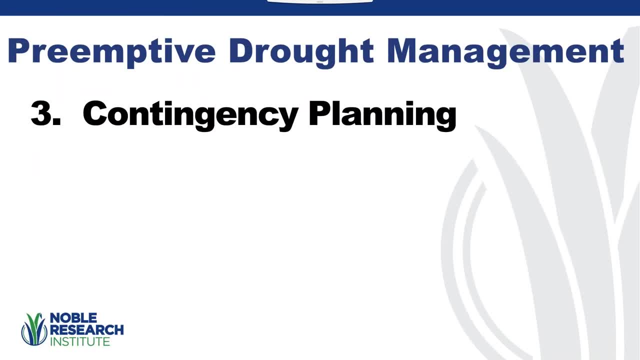 or expectations how you need to manage or adjust stocking should drought conditions prevail. Three: as we move into this, look again at preemptive drought management. we've got to focus on contingency planning, Doing the things that are going to make a difference. 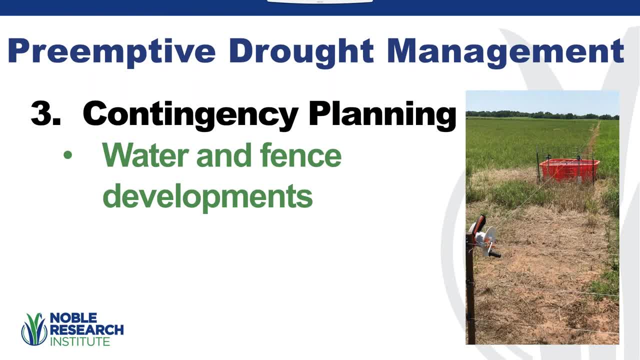 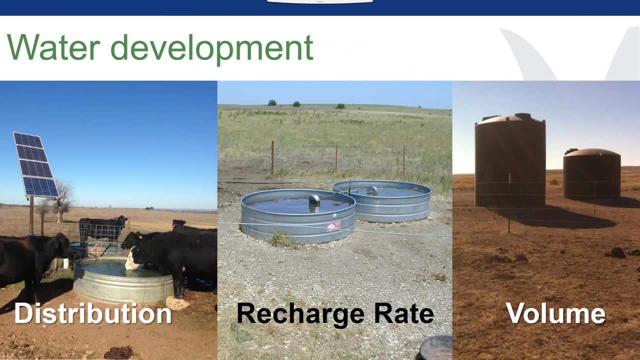 in the long term. One of the- probably one of the easiest or most justifiable capital expenditures is your water and fence developments, so that you can more efficiently and effectively apply grazing management to your ranches, You know, making sure that you have adequate distribution. 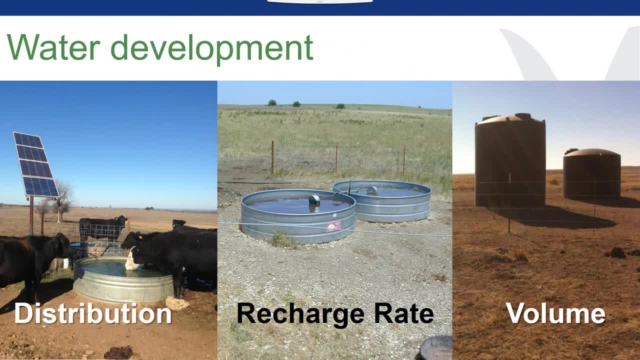 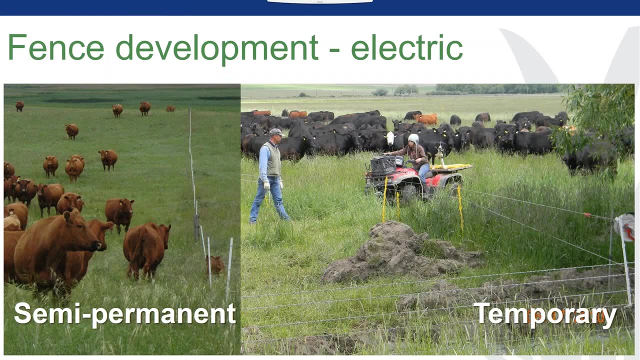 where you need it. Adequate recharge rates and volumes for the periods of time that you know that the cattle will be in certain pastures. Making sure that you have proper fence developments to where you can carry cattle where you want them at the time when you want them. 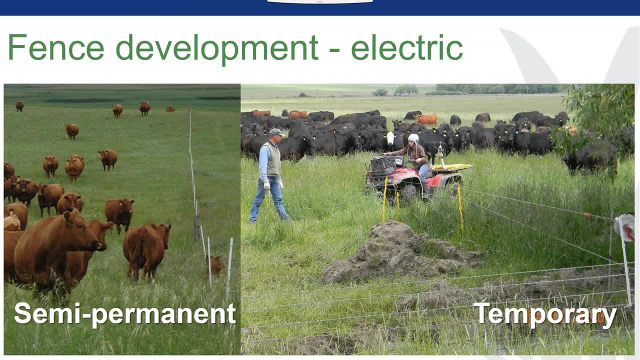 So that you can manage the rest and recovery, your graze periods And managing the different rain sites, soil types, the terrain that your ranch actually has. You know, we've got to be adaptive, We've got to be sure that we are managing 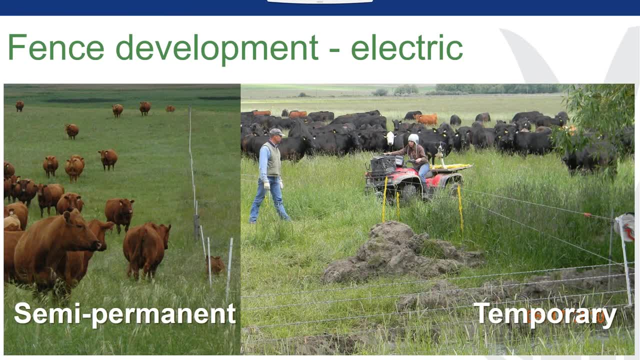 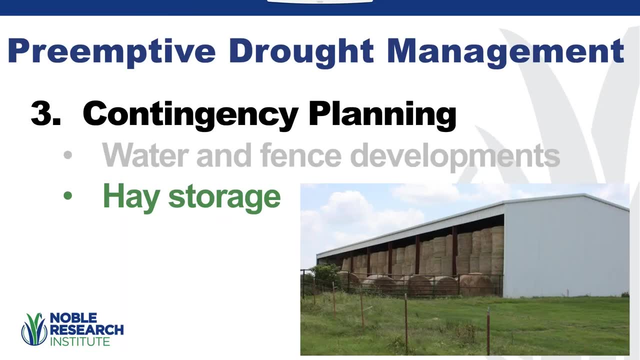 the entire resources as effectively as we can, And sometimes putting in these permanent electric or temporary type fences will allow us to do that more effectively. And then hay storage, especially as you go east where you have higher rainfall, just be able to protect the hay. 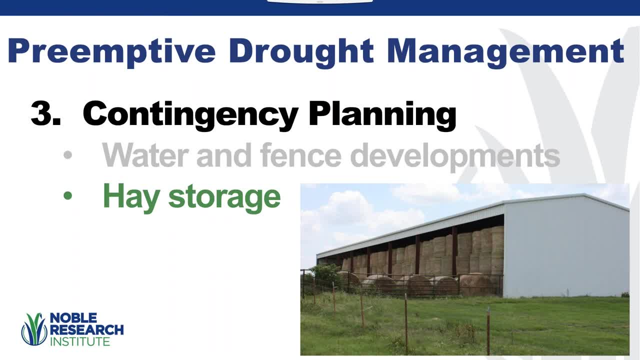 from weathering or other losses, Probably another one of those expenses that you can justify relatively easy if you get enough rainfall and if you're an introduced pasture system where you can warn itself. But no regard. but in no regards am I saying that you should ever try to feed through a drought. 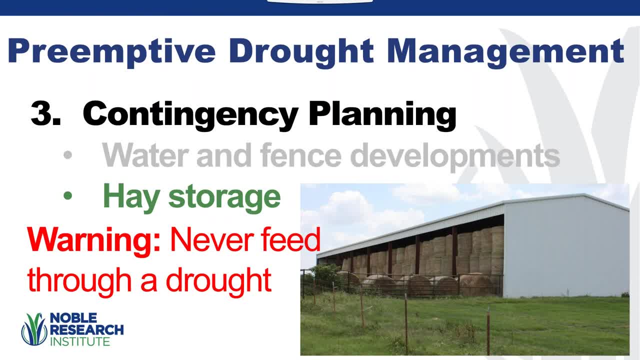 You know, typically in every case I've ever seen, it's never going to pay for itself and it would never be justifiable. So just a warning: never attempt to feed through a drought. That's not the purpose of this, you know. 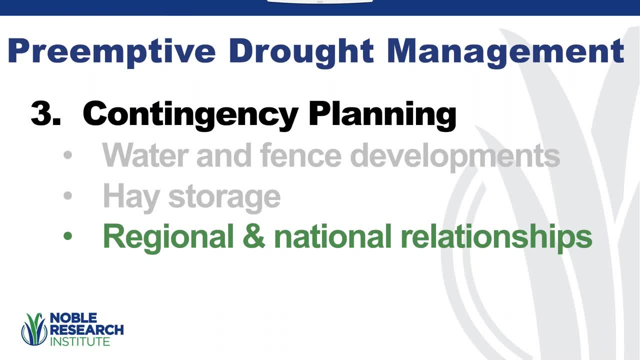 at this point And also develop relationships regionally and nationally. You know, especially if you're considering relocating cattle, It's those relationships that you can build with people that you can trust where you may have an opportunity to move cattle to an area. 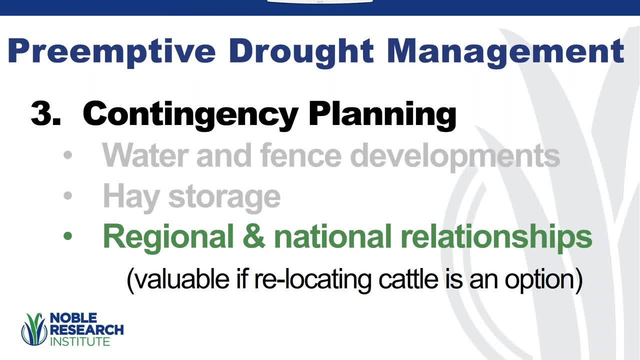 that may not be as droughty as you may be at a given time, But you got to have a relationship with these individuals in order to make those connections oftentimes. And then we get into the drought plan, The key thing that we want to talk about. 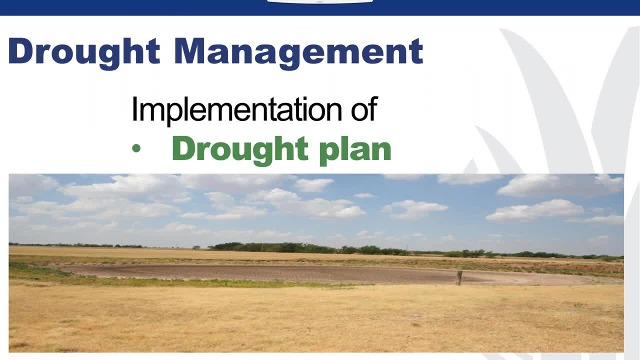 on the drought plan is the implementation of it, Even though we have developed it as a contingency plan well ahead of time. what does it look like as we get into it? And that's where we're going to focus now, Because even in a drought plan, 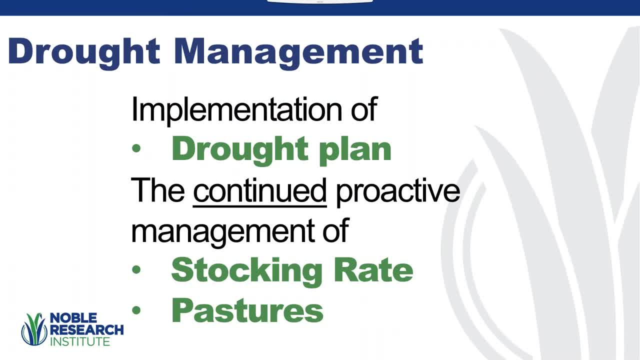 we've still got to continue to proactively manage both the stocking rate and the pastures, And that's one of the key points that I need to make: You never throw open all the gates. You've got to continue to manage throughout the drought. 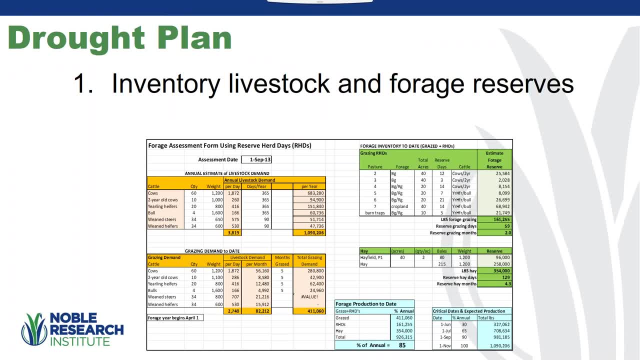 Just as a drought plan. some of the points that you need to be able to do is inventory your livestock and your forage reserves. You know, with a table, something like this, you can monitor your reserve herd days that are ahead of you against the livestock demand. 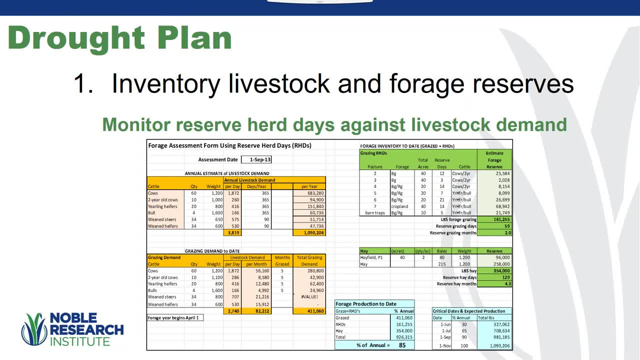 How long is it going to take you to get to the next spring, And do you have too many cattle? Do you have enough forage reserves at any given time, Or you expect to accrue between now and the next spring? That's what you're trying. 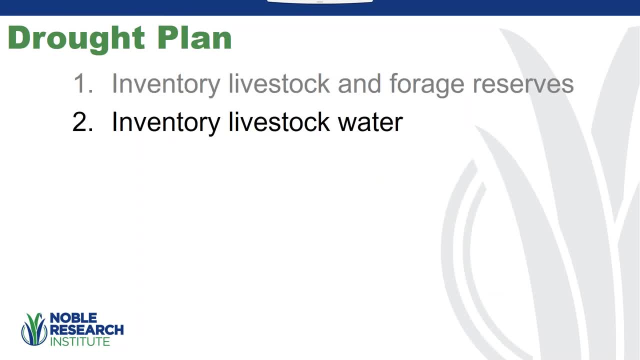 to manage for- And you need to be managed proactively for that Inventory livestock water. You want to make use of forage of the pastures that typically have lack of water during drought conditions, If they're going to be going out, if they're going to run out of water. 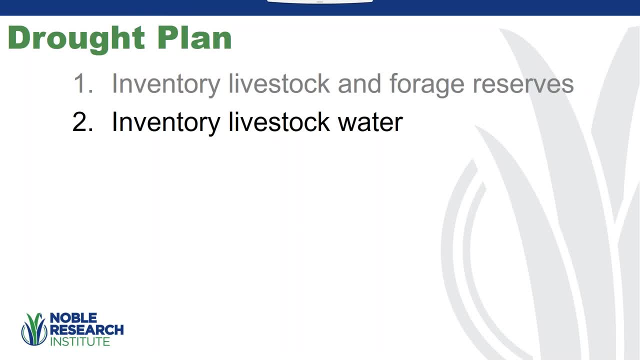 before you can use it. typically, you want to make sure that you graze those forage, that you graze those first, Being able to identify those areas early on and inventory what capacity of water can you adequately meet should you get into a drought? 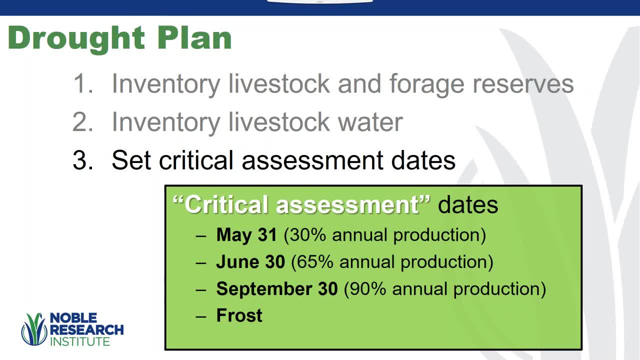 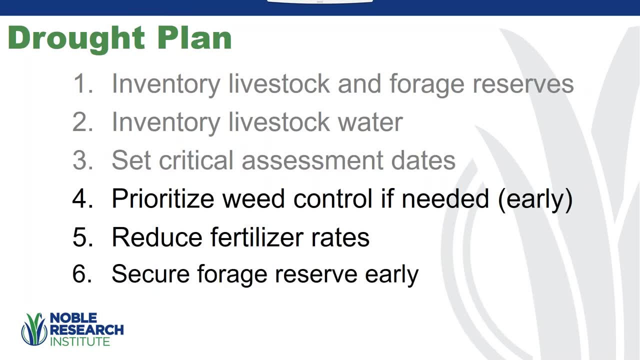 And then set critical assessment dates. Always be able to monitor, knowing where you're at, so that you make stocking or destocking decisions at different times. Prioritize your management, such as weed control, fertilizer rates, securing forage reserves early, if you're going to be doing that. 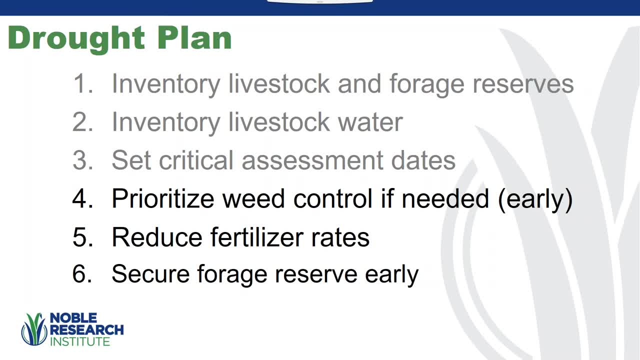 You want to make sure that you do that well ahead of drought, typically during times when you have, when you have cheaper prices on your forage reserves and at a time when they're most abundant. Seven: We get into the active part of the drought plan. 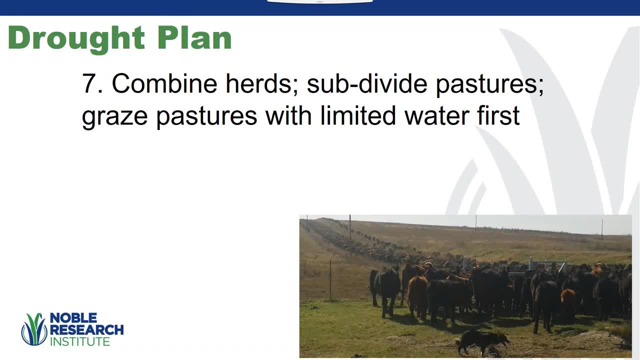 Combine herds, subdivide pastures, graze pastures with limited water first. You know we really want to get down to one herd, just as Frank described. Get down to one herd, subdivide those pastures. The drier it gets. 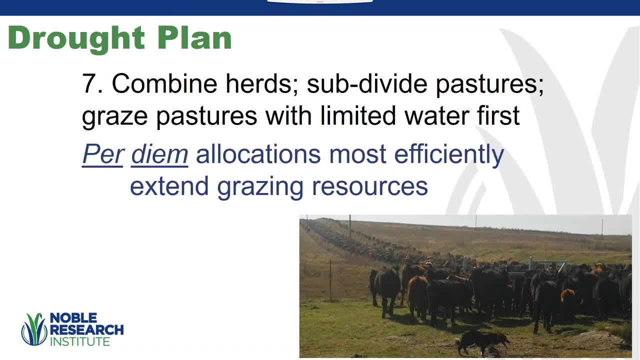 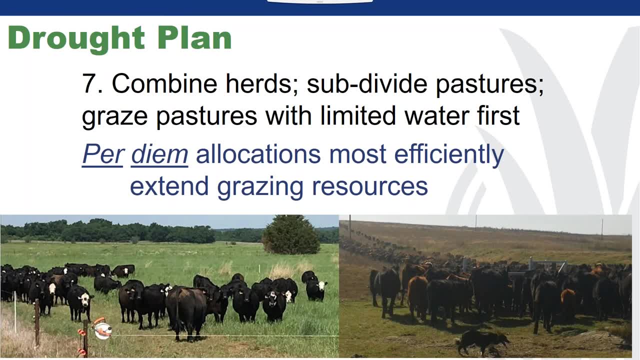 we need to have more control over the herd so you can actually continue to be able to manage the aufgabe of the other pastures at any given time and have these daily allocations so that we can more efficiently graze the resources in the extreme case or where you can actually. 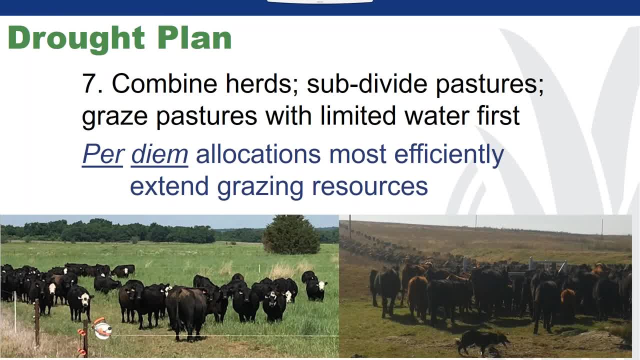 go in, allocate the amount so that you can still manage the residue heights and the reserve that you want to have going as you move from one pasture to the next- Very efficient way of doing it. It does take some time and effort and then continue. 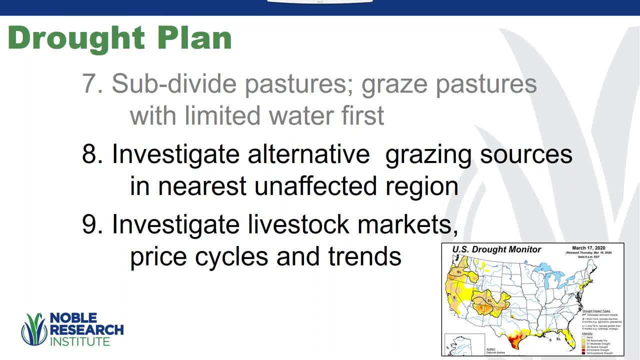 investigating alternative grazing sources in the nearest unaffected areas might be. should you consider relocating some of the some of your livestock? investigate the livestock markets and price cycles and trends and this drought of 2011- 2012: just the early diagnosis of drought: save producers lots of money. 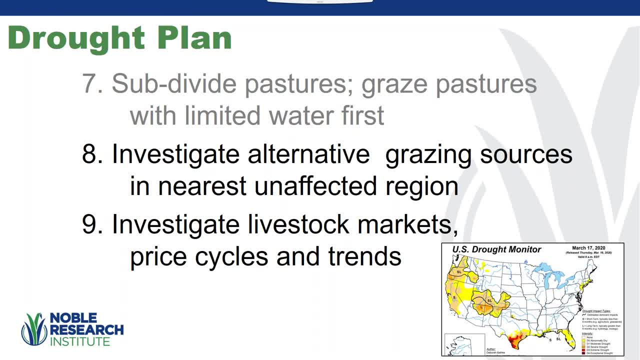 they D stocked in the spring, when at the early onset of that drought, and maintained prices for cattle that were never achieved again till we got into 2013- 2014 time period. so being able to market cattle successfully, knowing what those price cycles look like, in trends and strategically markets, cattle make a 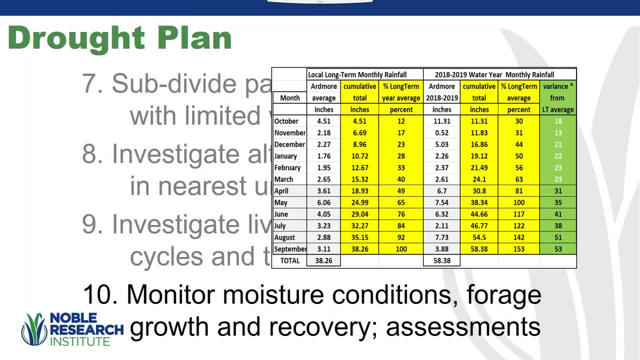 lot of sense and then continue to monitor your moisture, your moisture conditions, forgery, cook, growth and recovery. you know, as Frank said, if you can identify your pastures and know the key forages that are out there and understand what that looks like and how you need to adjust your grazing. that's 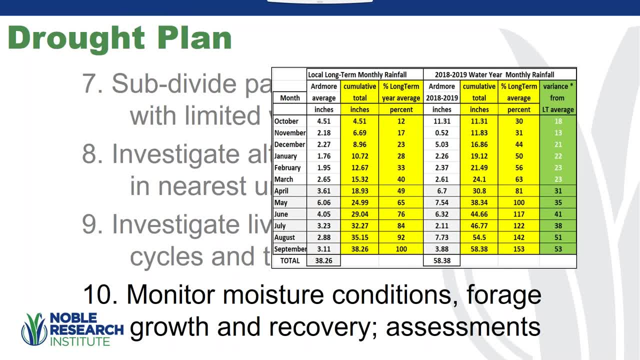 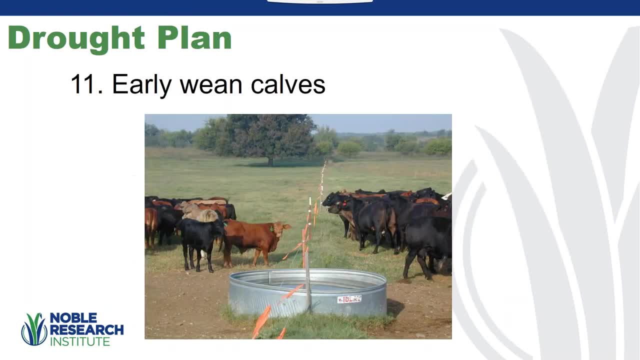 probably a much better method than trying to use a chart like like we have right here. but as you get into more predictable rainfall patterns, as you find in the central part of the US and East, some tool like this could be effective. 11 early weaned calves. we can least we can. 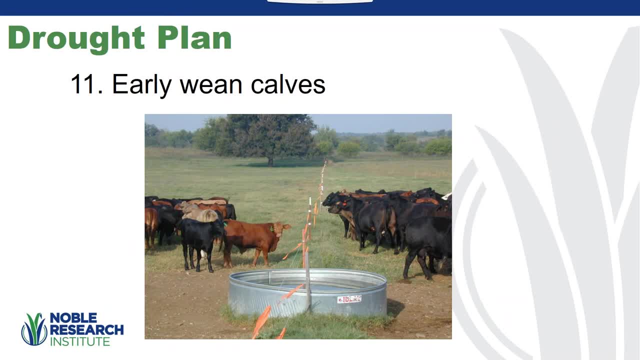 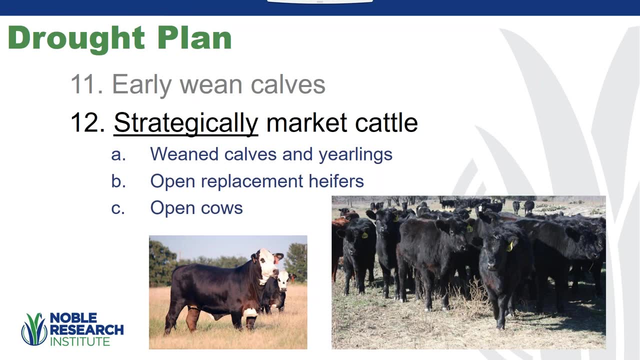 reduce our forage demand by almost 20% by early weaning our calves. so that's always a consideration. then, strategically marketing the cattle, just as Frank diagnosed. you know you, we want to wean these calves that are. you know that we market our weaned calves, our weaned calves that are, weaned calves that are. 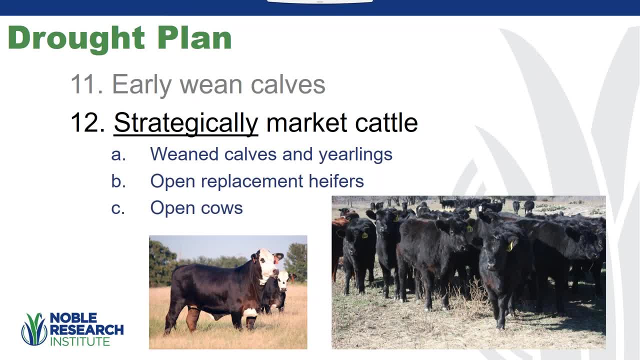 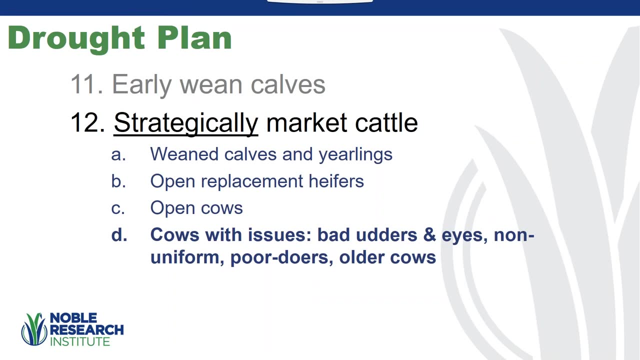 open replacement heifers, open cows, anything that is your, maybe months or years away from from actually producing. these are the most expendable and you're still maintaining the factory with on the operation. then you begin to look at your cows. you know, first getting rid of cows that that they have issues, the bad. 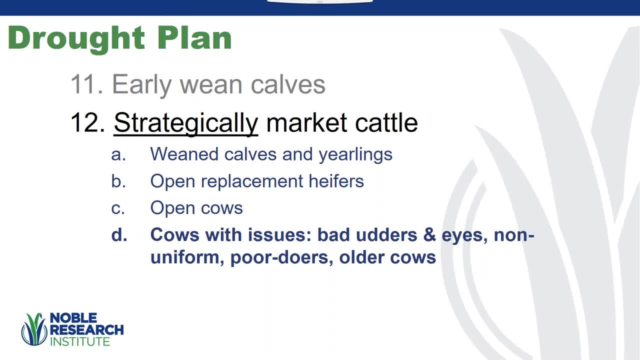 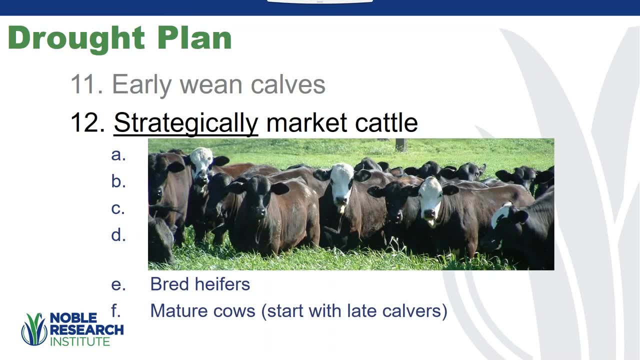 others and non-uniform- poor doers, older cows- you try to get down to the point where you have the core of your herd still left to take place and then, if it ends to become even more drastic, then begin to look at your bred heifers and 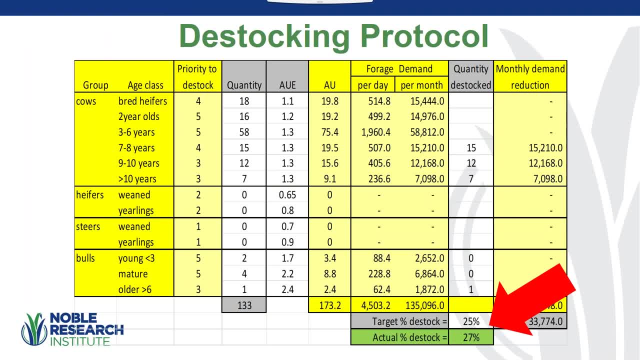 mature cows. so as we begin to get toward the end of this right here, you know this would be just an example of a destocking protocol, where it's when you're looking at the impact of destocking would have against your forage demand and your expected forage production could be, as you're beginning to manage both of those. 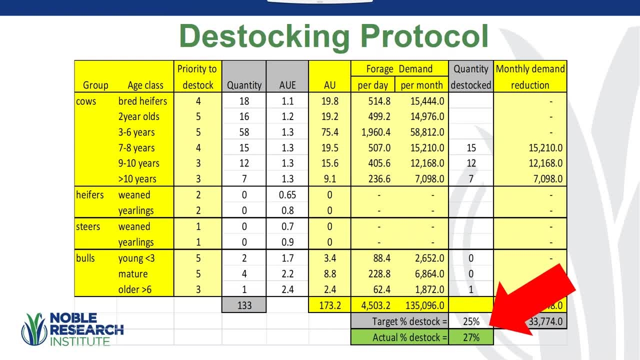 where you've got a target about how much you think you need to be destocked, based on your experiences and or indications that you have used through your monitoring, then begin to look at the animals that are younger animals or open animals, and then begin to get to the point where you see how many groups of animals or how 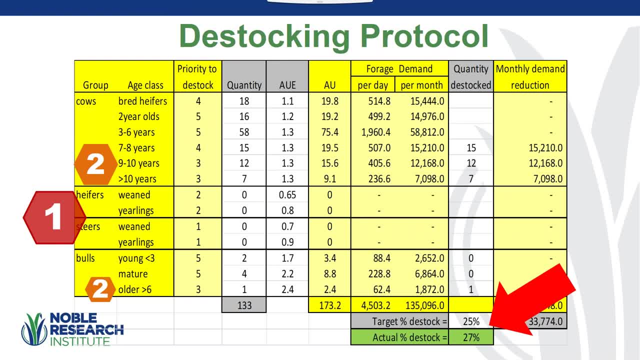 many animals within these different classes that you need to destock in order to meet your destocking target, and you know. thirdly, this would be the area that you'd be looking in X's we talked about earlier. so just having a destocking protocol, that where you systematically understand how you want. 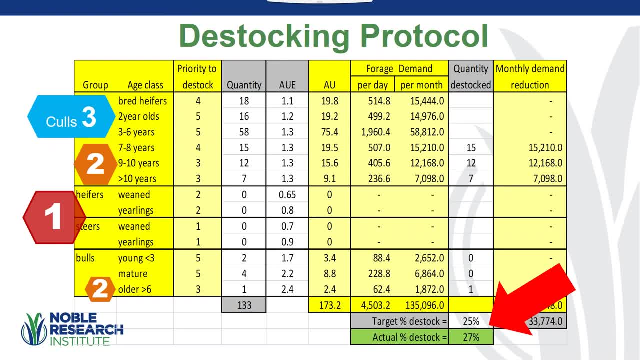 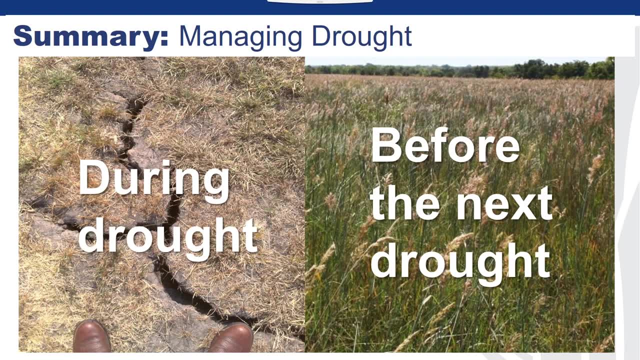 to step through reducing your stocking rate and still maintain the factory into the future. so, in summary, you know, managing drought. we've got two time periods that we've got to be focused on, the area that we call the drought itself and the time period before the next drought. we've got to constantly be. 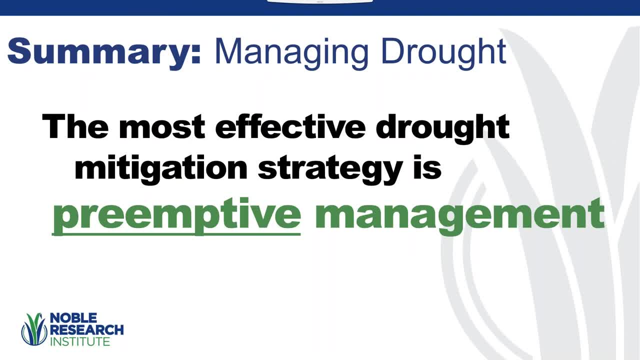 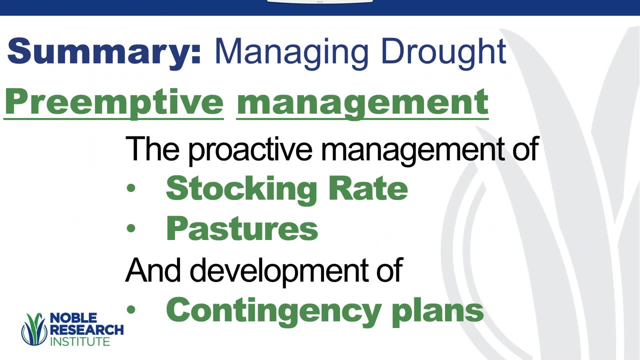 managing some of the key areas that we have the most influence over. as a result, we look at drought mitigation as being being a preemptive management plan- are part of our preemptive management plan, so therefore, stocking rate and pastures and developing contingents plans are critically important, no matter whether you're in a drought or you're preparing. 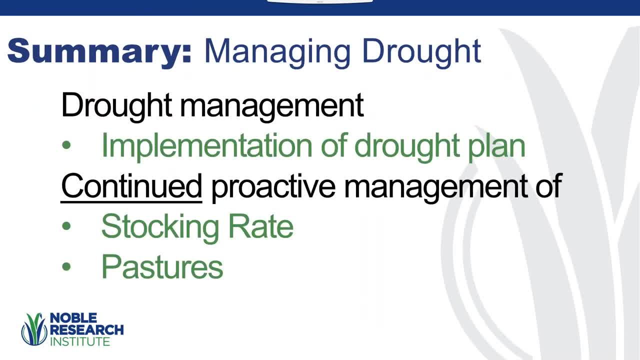 for the next drought, and when you're in a drought, we want to be sure that that we have a drought plan already in place, and then we're walking through this the way we should and then remember, continue to proactively manage stocking rate and pastures throughout, because as we come out of the drought, we want to make sure that our 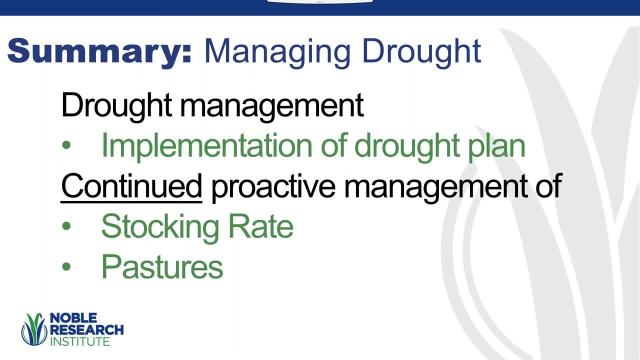 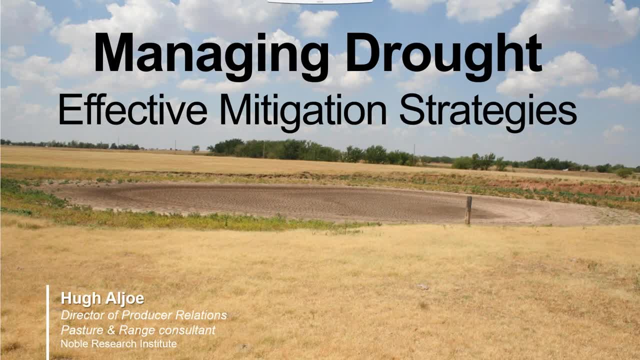 are prepared to take that first rain and recover rapidly. So with that I'm going to turn it over to Scott with Yolo Ranch. Scott Stone is a rancher there in California and I'm interested to see what he has to say as he manages drought. 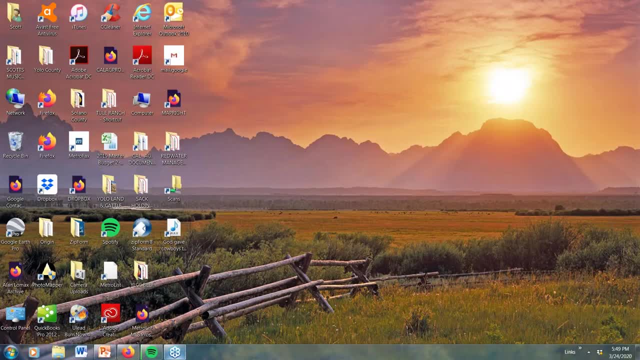 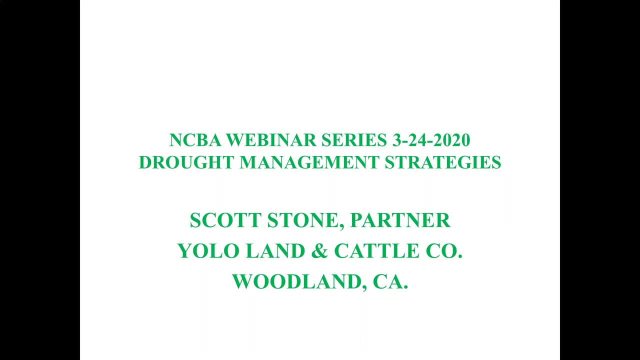 himself, Scott. Thank you, Hugo. Our company is Yolo Land and Cattle Company. We're based in Woodland, California. My brother, Casey, and I operate a cow cap and stalker operation. We also farm hay on our ranches, which are located on the west side of. 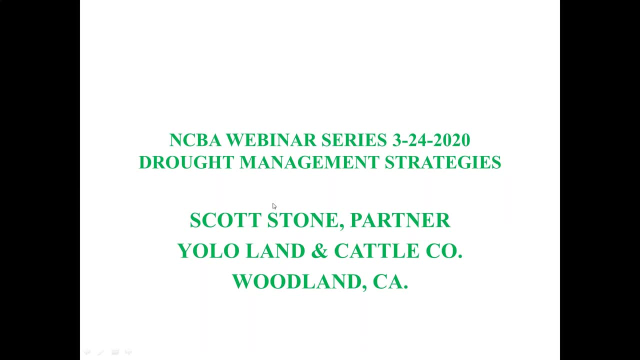 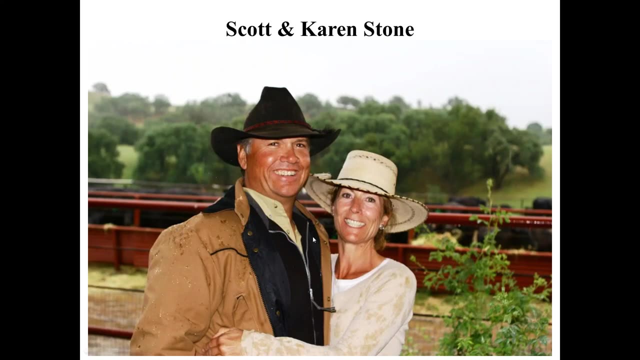 the Sacramento Valley. My father, Henry, started the ranch back in 1976.. This is our 44th year in the business. This is one of my favorite pictures of my lovely wife, Karen, and what I like so much about this picture: not only is she in it, but it's also. 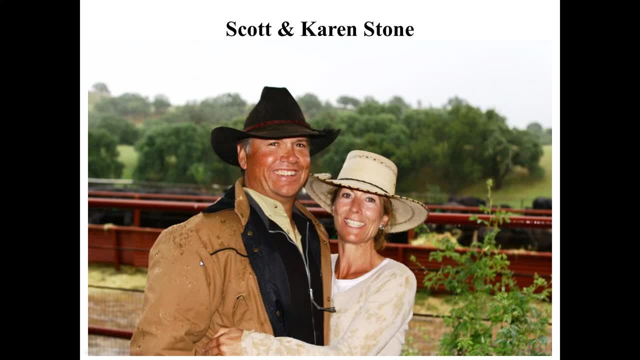 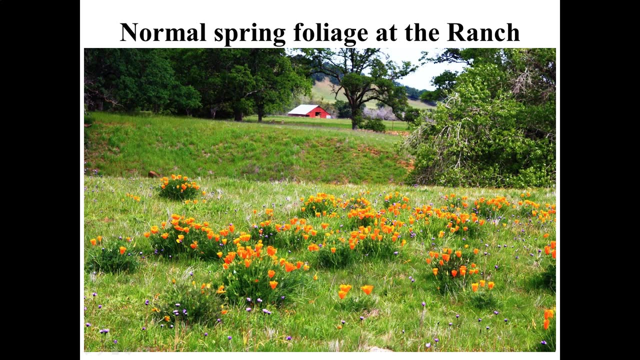 the last time it was raining out in our country. So our home ranch consists of 7,500 acres that run from about 300 foot elevation on the valley floor up to about 2,300 foot elevation at the top of the mountains. We have all our cattle in. 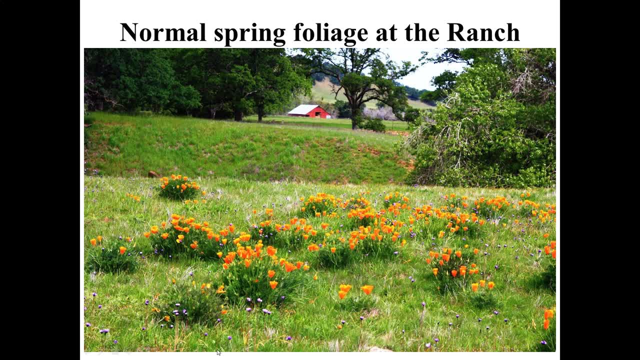 the mountain ranches from the end of October until the middle to the end of May. In May we gather and ship all our cattle off our hill ranches and ship them down to irrigated pasture ranches about 30 miles from our hill ranches. 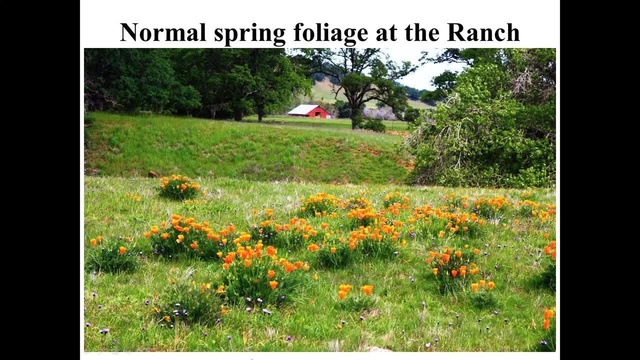 In our part of California during the summer months. the annual and perennial grasses are not nutritional enough to provide good feed for the spring pears year-round, so we have to ship everything to irrigated pastures for the summer and the fall. In our part of the state the normal average rainfall is 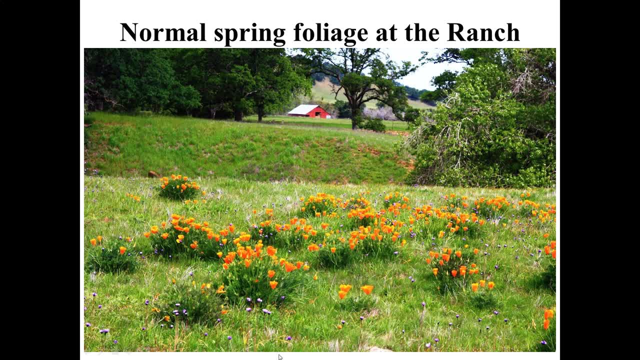 between 18 and 22 inches, and the one thing you can consistently say about our state is that there is no more normal and every year is different than adventure: fires, floods, earthquakes. we have it all out here In 2018, we have two. 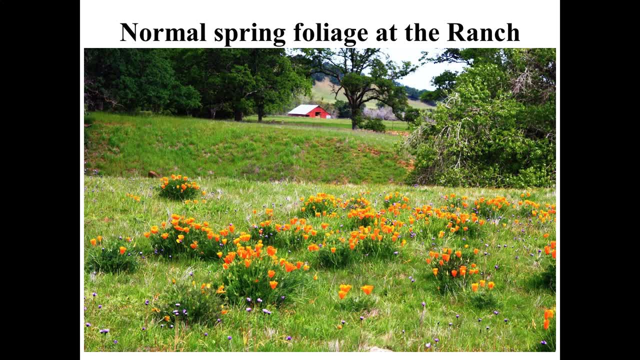 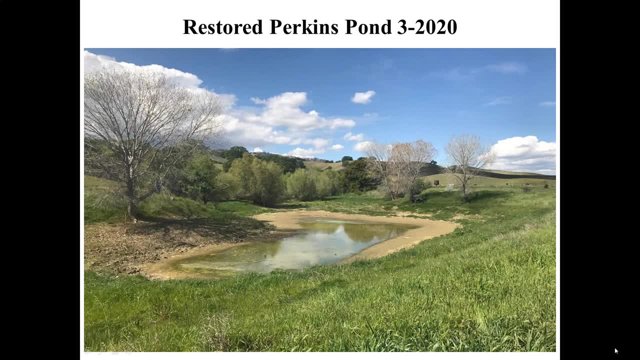 different fires that burn a total of 7,000 acres of our 7,500 acre home ranch. The fall rains historically used to start around the middle of October. It would rain few inches and then the winter grasses would start. then it would start. 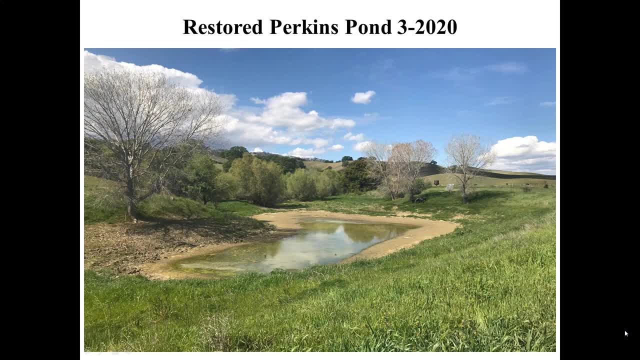 turning cold in November, maybe to begin into December 2018. after the Fire on the Pond Ranch started, That was the beginning of the fall the ranch. we got the very first rain November 30th of that year. then the weather turned very cold about a week after, so that grass did not start. 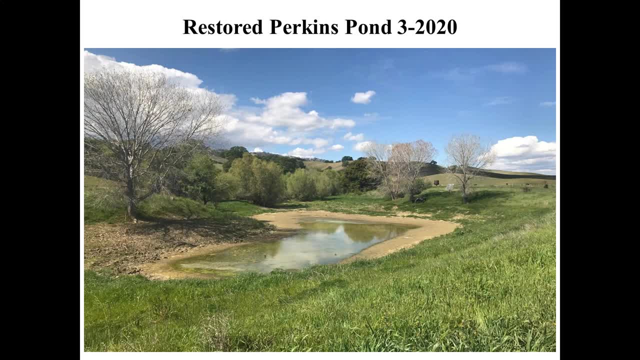 growing into the middle of February in 2019, which is also the time we stopped feeding hay to our cattle. the latest we fed that winter, we received 36 and a half inches of rain and we had a lot of flooding and erosion due to the lack of 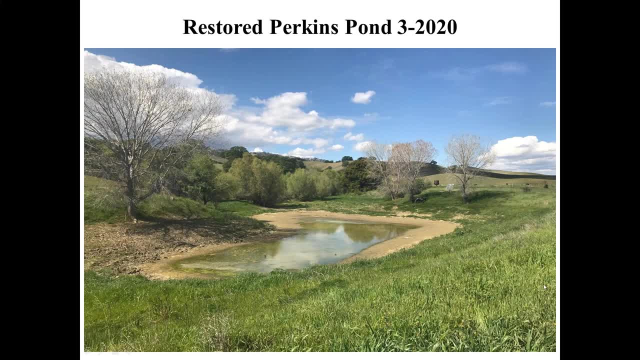 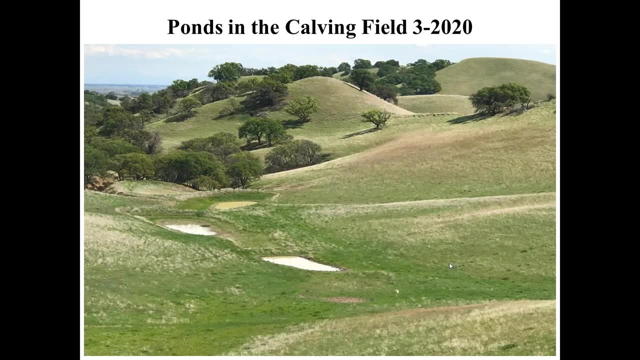 vegetation to hold the water back in the hills during the big storm events. and this slide I'm showing you. in the next one I'm going to show you are some of our pond- bigger ponds on the ranch. this is what they look like at this time of year. so now we're knocking on spring's door. the last week of March 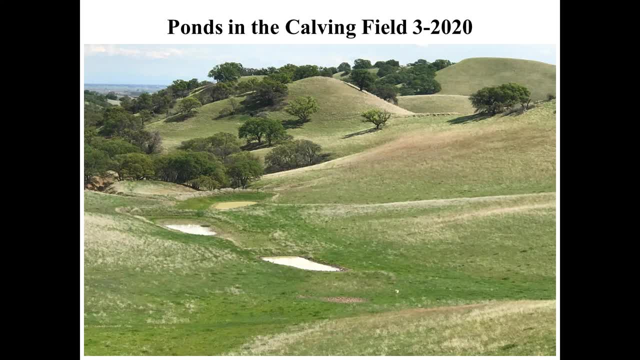 of this year and we've had a whopping ten and a half inches of rain. in the last 11 weeks we've had only a half inch of rain. so here we are again, going down from one extreme to the other. the interesting thing about that- trying to prepare for drought out here- is that we usually are trying to recover. 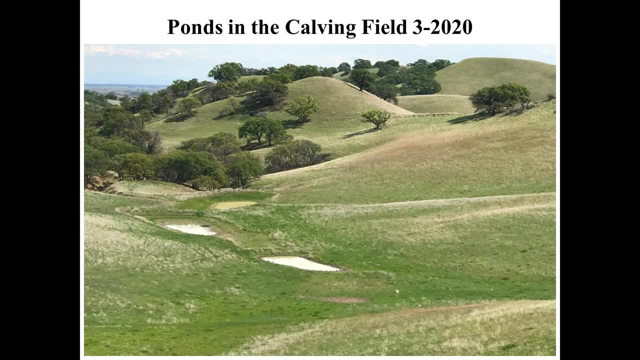 from something else prior to dealing with the drought. thank God, we cattlemen are extreme optimists, so today I'd like to discuss with some of the strategies we've been using to try and deal with drought as we settle into another one. out here in California, I do not have a lot of scientific charts and 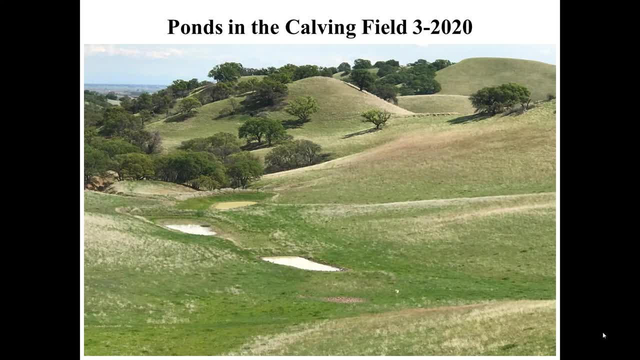 graphs to detail how we've dealt with droughts. just some pictures and a little common sense. just some pictures and a little common sense. every livestock operation in every state is completely different and you just have to try and manage your own resources that you have at hand on your 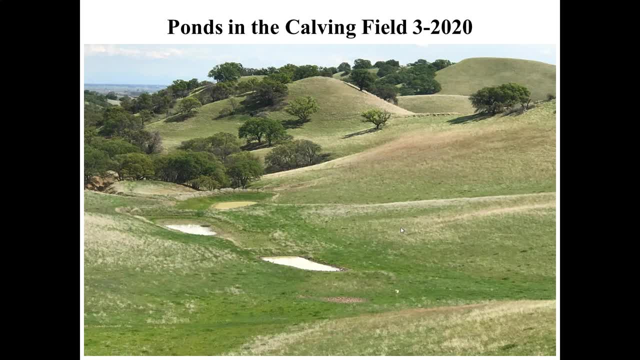 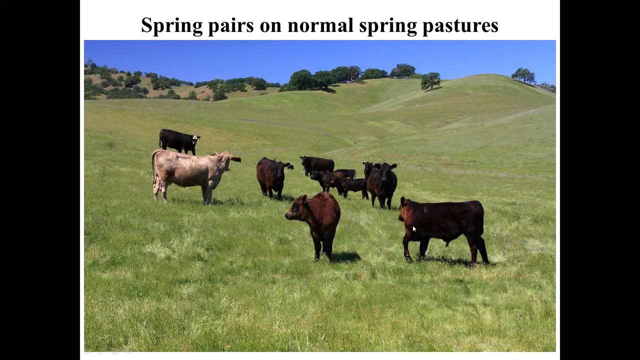 operation to deal with droughts. most of the things that we've been doing have been occurring over time and have multiple goals when we tackle them. managing for drought is always part of these decisions and goals. well, so some of these droughts start going through the strategies over the last 13 years. 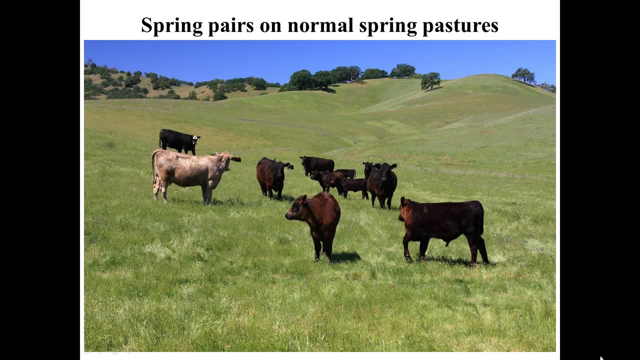 we've been switching our herd from 100% fall calving herd to 100% spring calving herd and last summer we took the final step of selling off all our older bred fall cows. we did keep 50 of the youngest and best fall cows and held them over to. 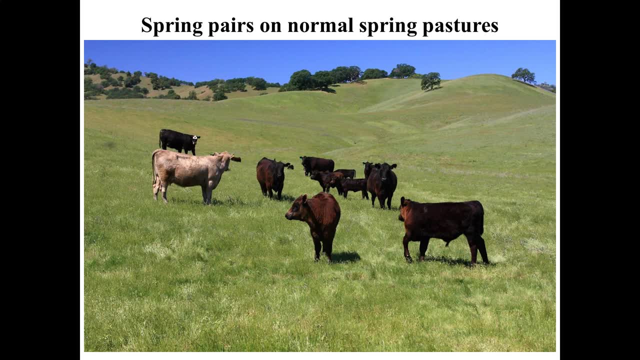 breed this spring with all our other spring cows, and we did this for the following reasons. first of all, we do not need to feed spring cows any hay, like we used to do to the fall cows. this frees up labor and resources to do other things, saves us money. now we sell. 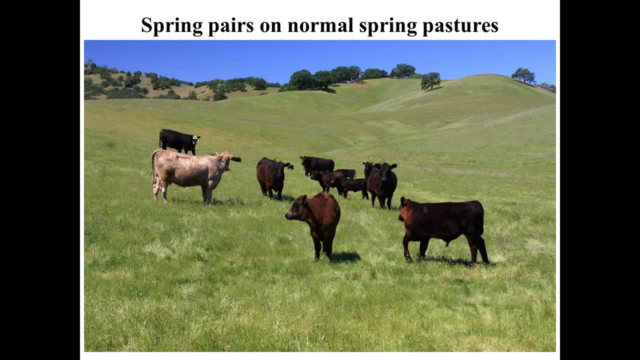 the hay, which increases that revenue stream, is much faster to calve out. the cows brand the calves in the spring rather than November or December, when it usually reads: cows are calving in sync with nature, not against it. after we wean the calves in the fall, we wish to retain them as stalkers. they are ready. 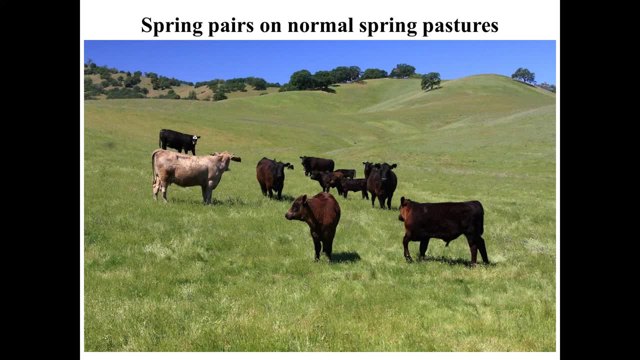 to go out in the hills for the winter. we already own them, they have all our cost into them and they are locally raised. another thing we try to do on all our owned and leased ranches is: rotationally grazed the ranches and it looks there's different. 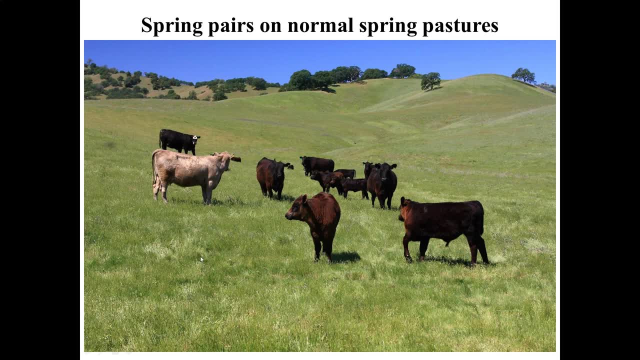 systems for different ranches depending on size, water availability and everything else. in order to graze cattle in a successful rotational system, the most important thing is to have good water for structure and good fences. you can get by even if your fences are not in great shape, but you 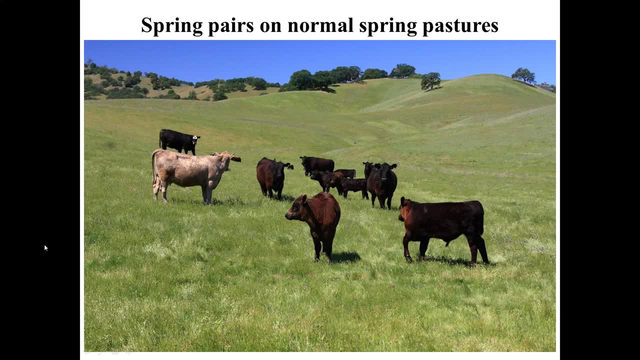 cannot get by about good water resources. ideally, we like to see two sources of drinking water in each field. one is the dirt tanks or stock ponds that we have multiples of in each field. the others development of springs or domestic wells that are solar-powered. good well can provide water to cattle in more than one. 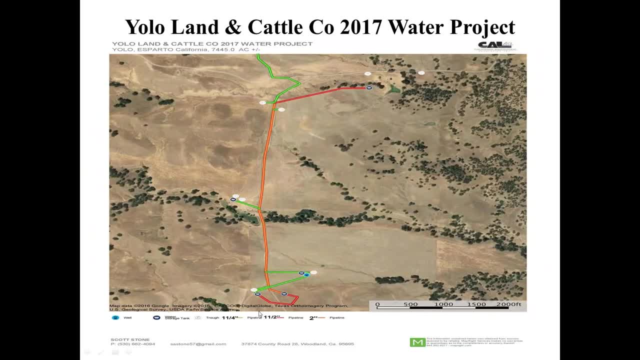 field. three years ago we partnered with our local NRCS office in Woodland to develop a water system that would provide water year-round, with some of the fields in the middle and south end of the ranch that were consistently short of water when the ponds would dry up in the spring, we were not able to. 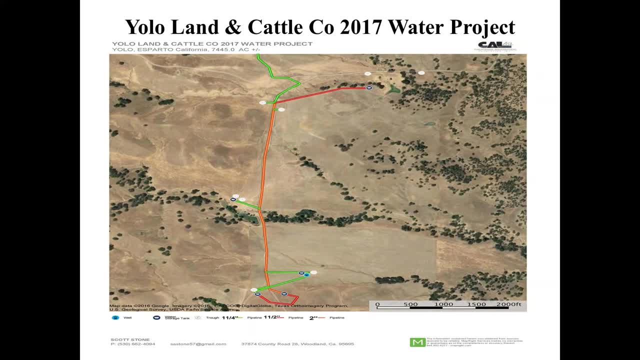 take advantage of grazing some of these fields in the fall until we got winter rains to replenish water in the ponds in a drought situation that is exacerbated because we don't have the water for the ponds. so we drilled some test holes around the ranch with hopes of installing. 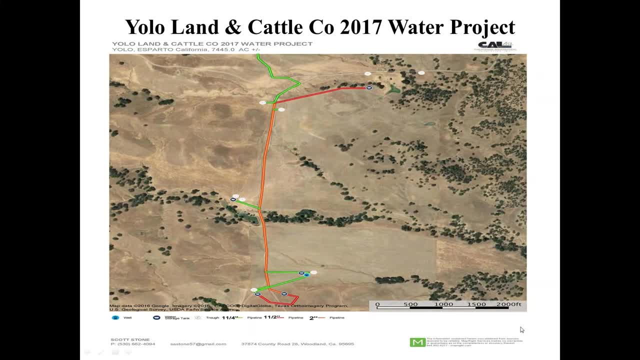 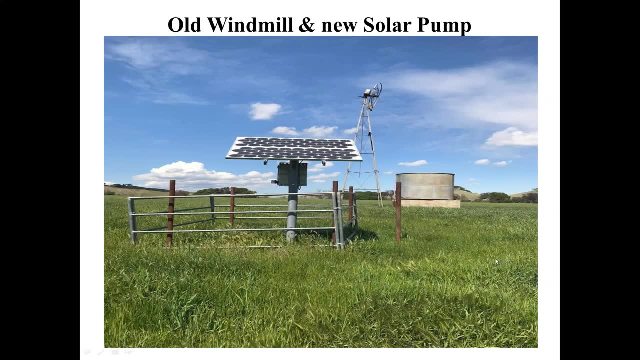 solar-powered domestic well and drilled a small domestic well at the south end of the ranch. we then installed two 5400 gallon water storage tanks and connected them to a new domestic well and an existing natural spring on the ranch. in this picture you'll see the windmill. it's been out there on the ranch for. 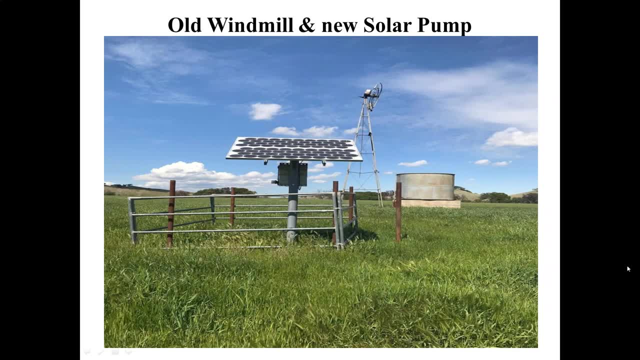 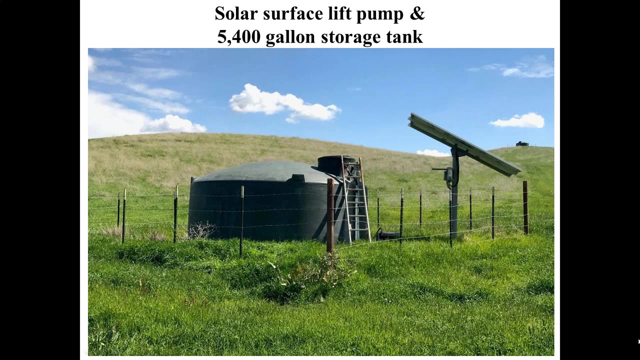 probably 70 years, and it's been in use for about three years now. we're going to put a new tank next to it and then you'll see the new solar pumping. well, one storage tank that we put in is located at the bottom of the hill and it has a surface solar pump. 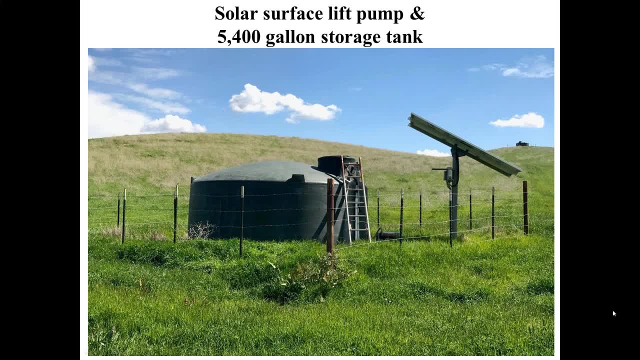 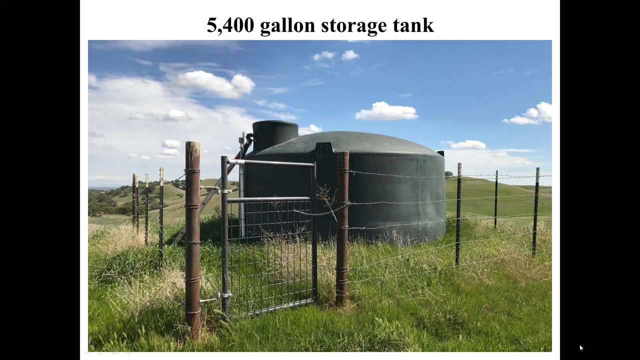 which pumps it up to the other storage tank which is on the top of that hill to the right. you can just barely see the top of the storage tank- picture of the tank on top of the hill- And that tank has a two-inch PVC line that we installed. 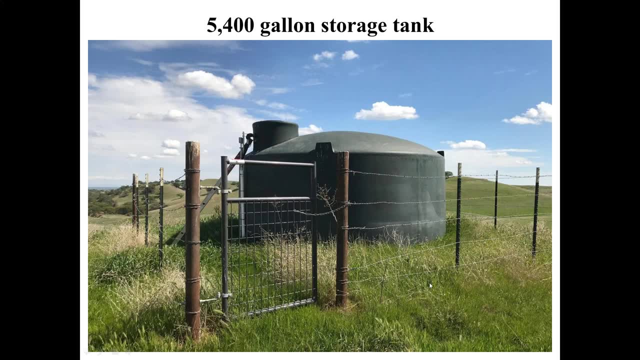 It runs for two miles across the ranch And we tied that line into three other storage tanks in different fields, which increased the storage capacity of the total system to about 26,000 gallons. The new system also provided us with water troughs at 14 different locations. 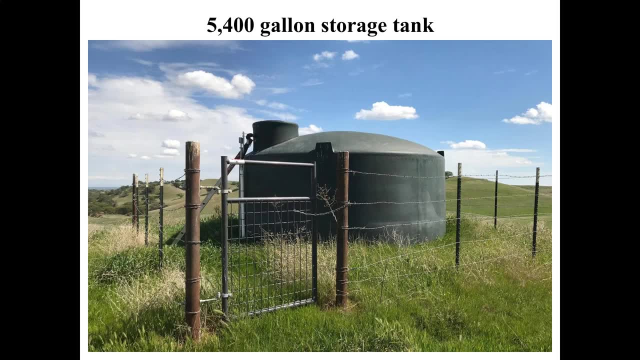 And it has allowed us to utilize the lower fields in the fall, with or without any rain. One of the critical points of the water system is the type of water trough and flows they're using in the system For any new construction on the ranch. 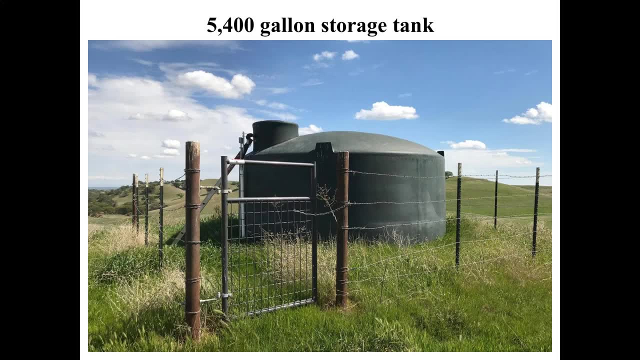 on the water systems. we only installed 4x10 concrete troughs. We also only installed floats which have proven to be the most maintenance-free and reliable stock tank floats that we have ever used During the drought, when we only have one water source in a field we cannot afford. 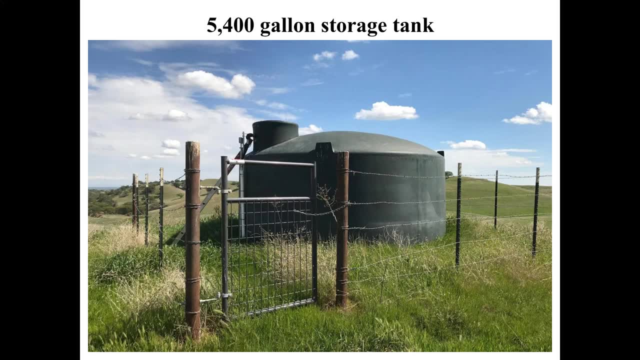 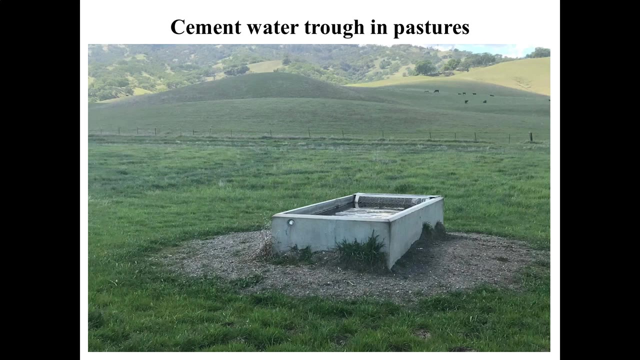 to have the system get drained of the available water because of a faulty float or a leaking tank. Over the last few years we have replaced almost all the metal and plastic troughs on the ranch with concrete troughs and Watson floats. It costs more to do it, but they rarely have any issues. 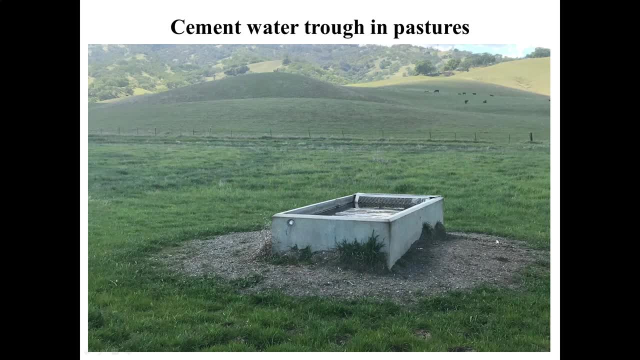 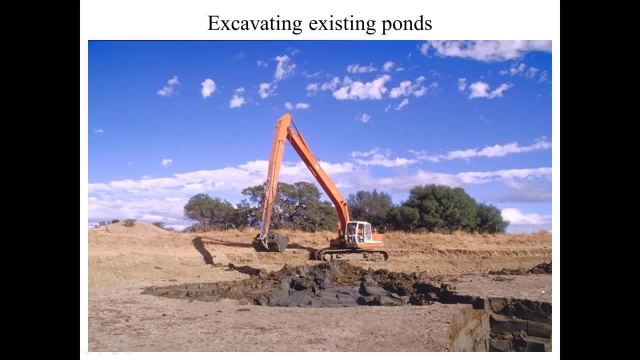 We are constantly cleaning and repairing existing reservoirs on all the ranches so that when it does rain, we're in a position to maximize the capture of winter runoff. We are a proponent of composting on rangelands and have been trying to do so for the last. 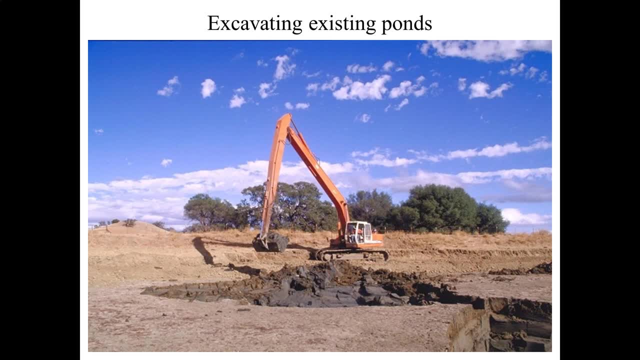 few years. When possible, we make our own compost on the ranch with old hay or source some shavings for horse manure. We have partnered up with our local resource conservation district and the California Department of Food and Agriculture for a three-year demonstration grant for the Statewide Healthy. 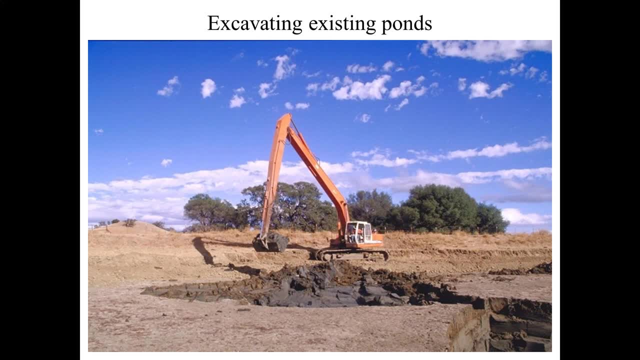 Soils Program. The demonstration grant provides funding for an application of five tons of compost applied to 50 acres of rangeland each year for three years. The soil is then closely monitored and measured for the amount of carbon from the air, the plants and roots that seep into the soil. 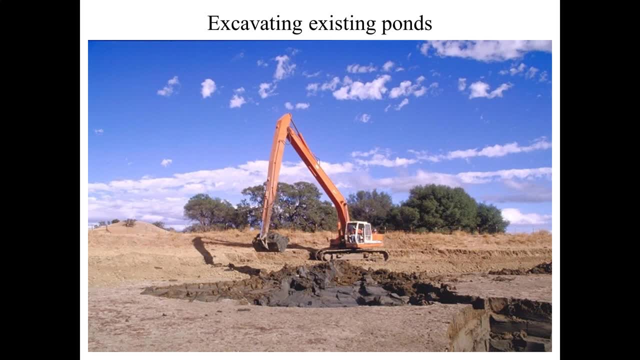 The soil is then sequestered, also the amount of additional plant growth produced and the amount of additional water infiltration capacity, ie groundwater recharge, that the soils can achieve due to the compost applications. The scientific studies being generated by these programs are proving what we ranchers 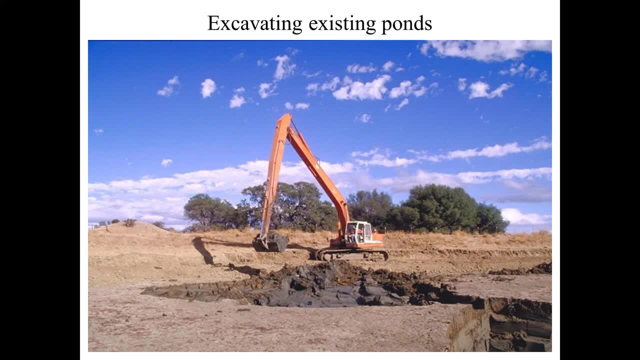 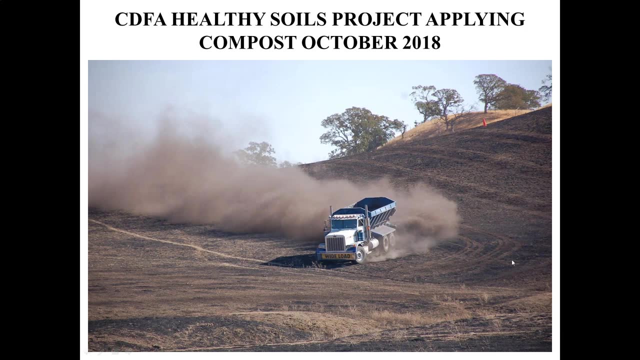 have known all along, Raising on rangelands is good for the environment, So we're fortunate enough to be here. Thank you, I'm very happy to be here, So this is a little bit of a side note. We're working with the City of Washington to have some improved irrigated pastures down. 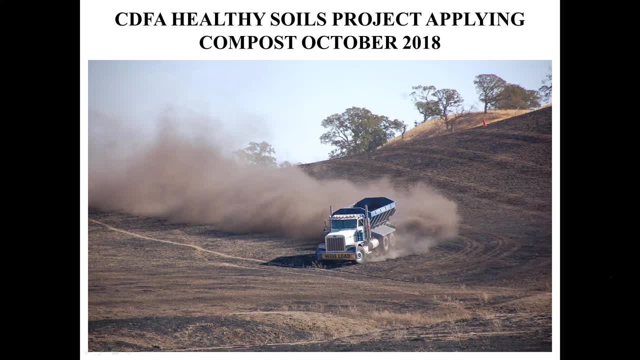 in the Valley, about 30 miles from the ranches And on these irrigated pastures, over the last few years we installed a concrete weir and sump pump to reuse the drain water that's generated from the flood irrigation of 600. 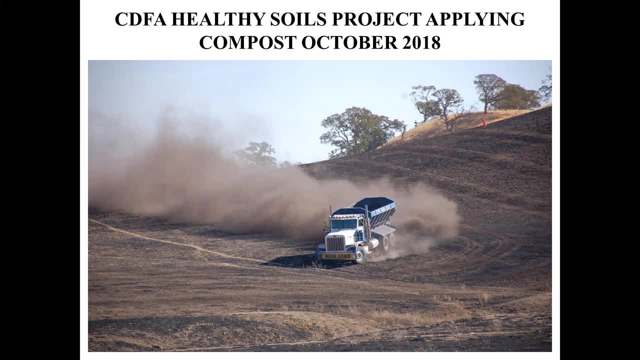 acres of the pastures. Once the water is applied to the irrigated pastures, it is captured in the system and reused over and over again Again. this is our first time doing this, But this is just a little bit of a summary. 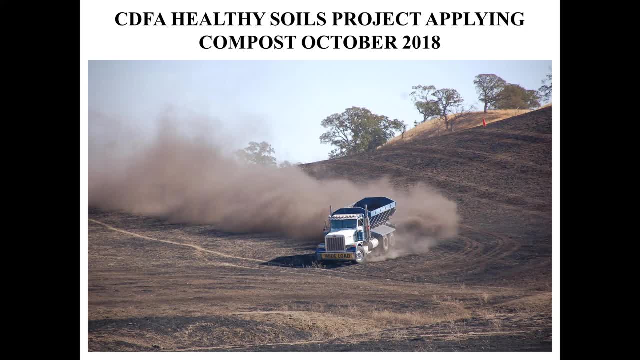 It's a little bit of a summary- irrigate the pastures. We've also installed a 24-inch drain pipe under a county road to bring drain water from an existing Reclamation District drainage ditch into our return water system. This provides us with additionally. 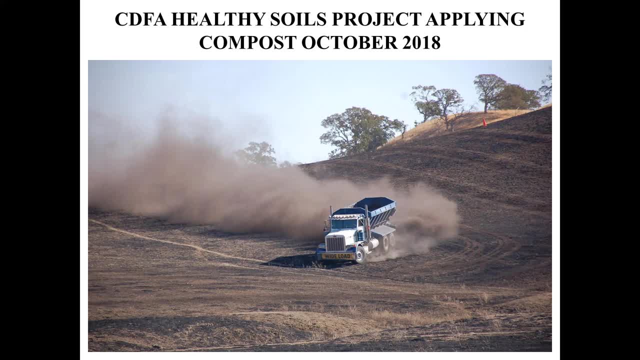 economically priced irrigation water for the pastures. Thanks for your time this evening. I will be happy to answer questions at the end of the program. Thank you to all of our presenters, Frank Hugh and Scott NCBA's Cattlemen's. 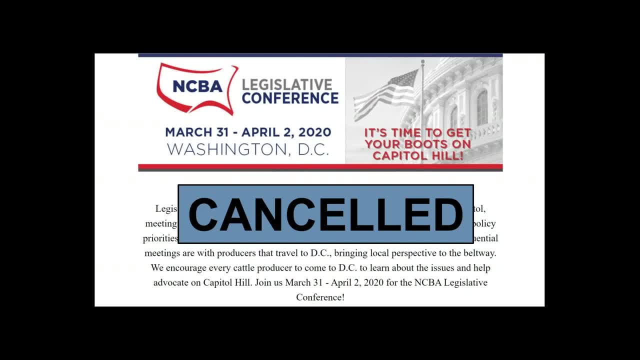 Webinar Series has the goal of bringing you the latest information that's relevant to any producer in this country, and our presenters tonight have sure helped us to achieve that goal. As we move into the question and answer session, I want to remind everybody that while our spring legislative conference was, 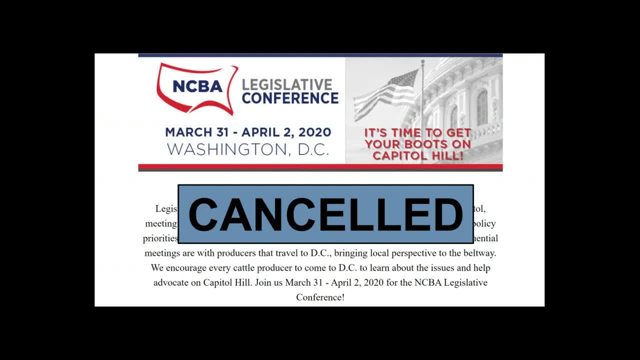 cancelled in Washington DC. the Washington DC team continues to work on your behalf with regulatory agencies, including lobbying for support of programs like EQIP, which help cost share many of the management practices discussed in this series. Your officers, NCBA officers and the leadership in Denver and Washington DC are continually engaged on a daily 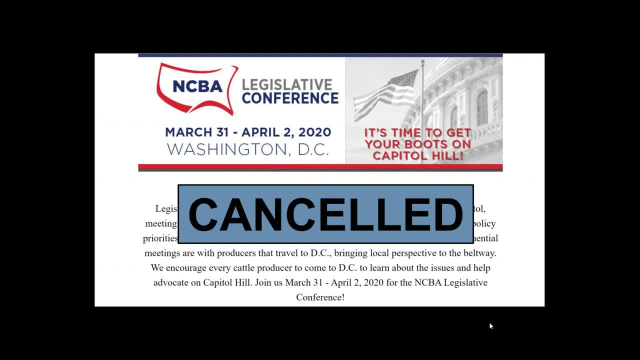 basis to address these challenges that we now face with this COVID-19 invasion. So be assured that we're working as hard as we possibly can to make sure that we can optimize benefits, even if we can't. Thank you, Thank you. Thank you so much. 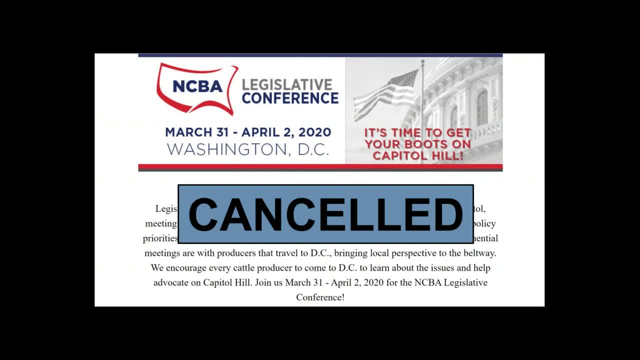 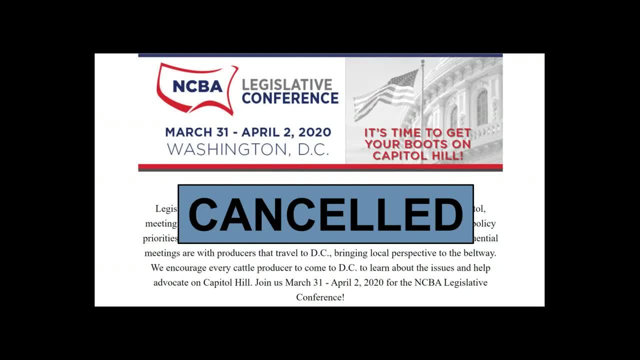 If you are a member of NCBA, really appreciate your as a treasurer of NCBA. I really appreciate your support And I know that your fellow members appreciate that too. If not, please consider joining, and you can do that by going to ncbaorg. 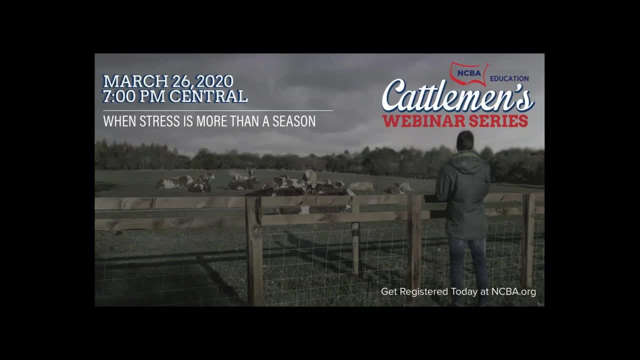 Two more webinars are coming up, One this Thursday night with two professional counselors, So I encourage you to go back and take a look at those All right, who will discuss how to manage stress and how we can support each other during these. 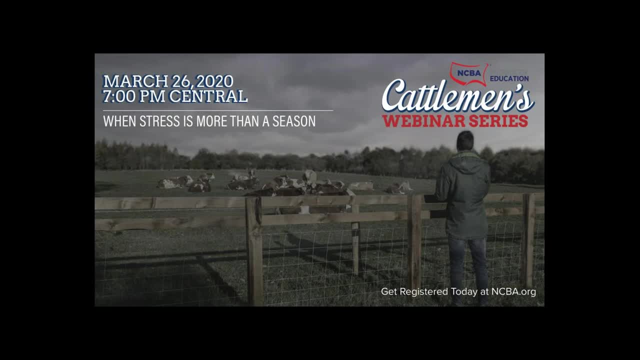 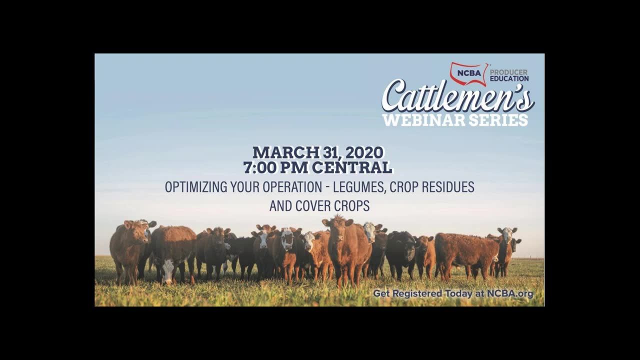 trying times. The final webinar is entitled Optimizing Your Operation – Legumes, Crop Residues and Cover Crops, And registration for both of those webinars is open under the Producer tab at ncbaorg. I was interested that both – that two of the presenters mentioned, Hugh and Frank, mentioned. 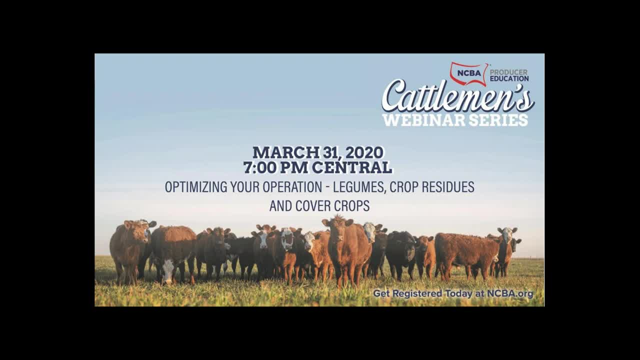 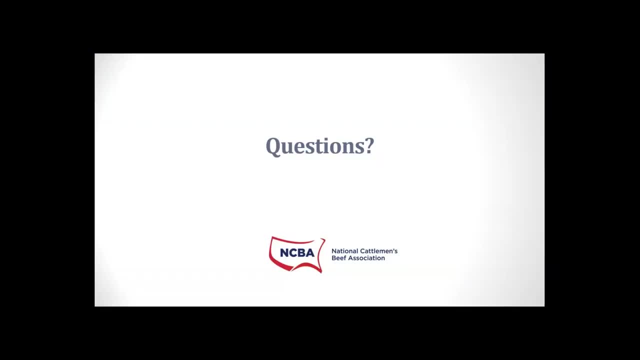 animal management, and I think it was Hugh who called it preemptive management as one of the tools we use to mitigate the problems with drought. I'll just give you a quick anecdote: The ranch I'm associated with has – several thousand mother cows, but we also run 6,000 – up to 6,000 range sheep when we have the ability to do so. Normally we wouldn't be coming out of winter range and hauling the ewes back to the headquarters ranch for lambing until about the middle of April, And two weeks ago we made the decision because of forage –. Forage: Lack of forage To haul 5,000 of those ewes. we left 1,000 replacement ewes on the range but we hauled the rest of them back, So we had to move off that range about four weeks early. 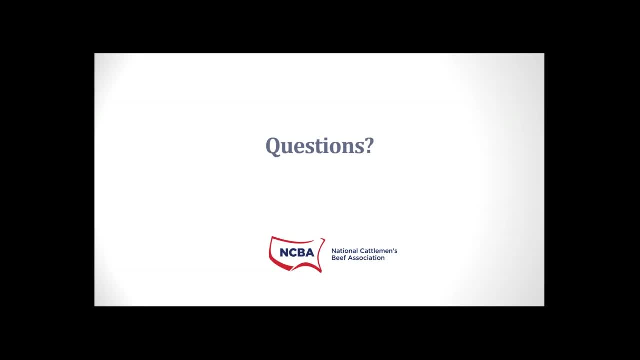 With that, let's get to some questions. Josh, I think you've got those that have been delivered via email. I'm sorry. I'm sorry. I'll turn it over to you. Sure, And just to remind everyone that's still on, you can chat in questions in the question. 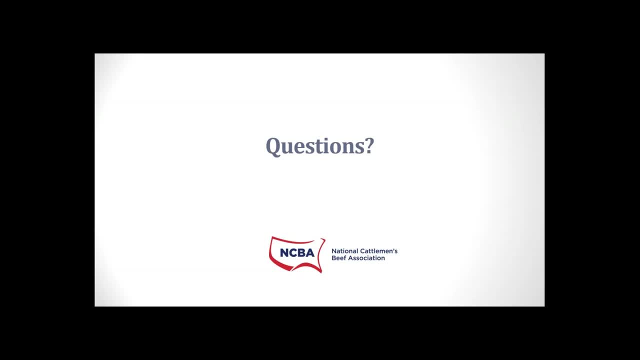 box on your screen. Just click on that and type in any questions you have. I'll start with one, I think probably geared towards you, but everybody may be able to chime in based on your experience. How do you go about assessing long-term rainfall data if you haven't collected it yourself? 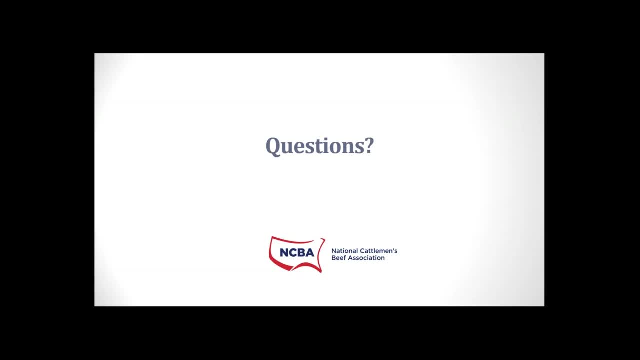 Do you know if you've collected it yourself? Do you know of any sources, Hugh, that folks could go to, or any of the panelists any recommendations on how to get that data from years gone by? Well, it is difficult. That's one of the challenges that we all face. Some states, like Oklahoma, where you've got a Mesonet system, you've got a long-term rainfall records that go back a number of years and you don't have to have 125 years' worth of rainfall data. But when you do that, it's a lot. You develop it like a water year table. You just need to go back to the last 20, 25 years. Your county that you reside in maintains monthly rainfall records and that's where I've found the most reliable source to get that, at least for individual ranchers that I work. 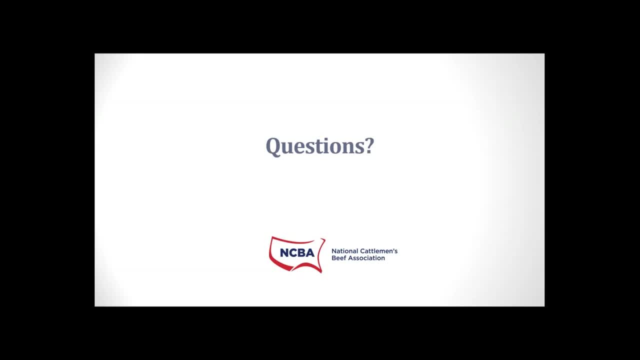 with Those charts that I've showed you. most of those will come from the Southern Georgia. Some of them are from the Crescent Coast. Southern Climatic- I'm trying to remember what the abbreviation but the Southern Climate SCIPPS is. what is the abbreviation? 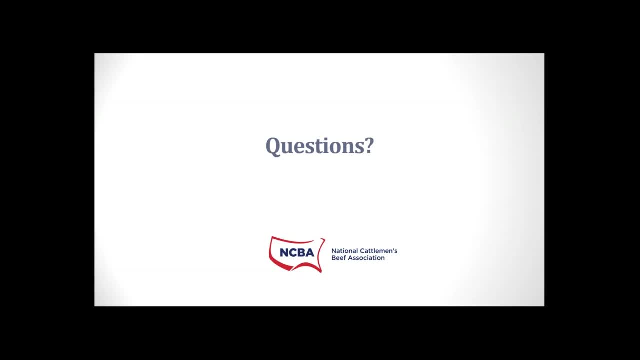 But the Southern Climate Hub is where a lot of that information would be coming out of And if you have questions, contact me there at Noble. I don't mind trying to help Frank or Scott. either one of you look to any outside sources for any of that historical data, or do you rely on your own data? I rely on my own. I started, for whatever reason, in 1984 and keep pretty detailed records, And I've always tried to establish trends with that rainfall and I can't find one. So anyway, that's what I work with. Yeah, we use kind of the old-fashioned way. We have rain gauges and we just write down from every storm and we tabulate it at the end of the season and then store it away and compare it against the previous years. We're probably doing that a little over 20 years. 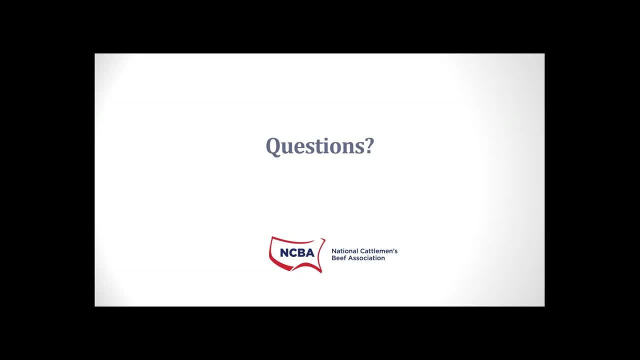 Hugh, I think I've got a follow-up question to that. I think folks were maybe having a little bit of trouble understanding- I know you were flying through that information but understanding some of your tables and how you assess the reduced rate, you know what those triggers are. 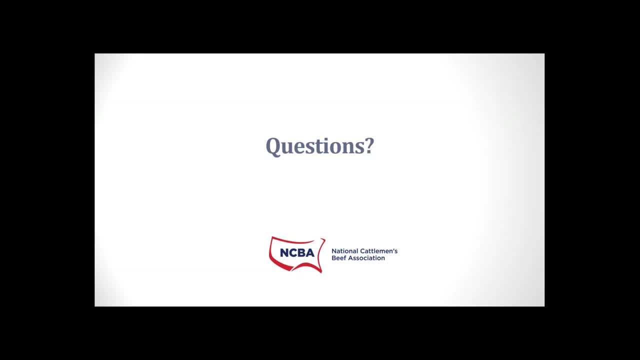 I can hand the controls back to you. if you want to go back to that rainfall table, Let me pull it back up. Just tell me when you're ready and I'm happy to kick it back over to you. And it seems like that's what a whole lot of the questions are being generated around. 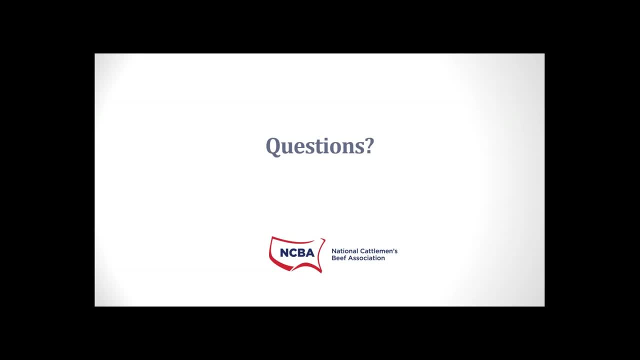 Okay, shift it back And I'm going to make a suggestion. I have another question about supplementation strategies on deferred pastures And I just want to refer you back to the webinar we did. I believe it was the one last week Where Jason Sawyer from King Ranch Institute spoke and he spoke extensively on supplementation. 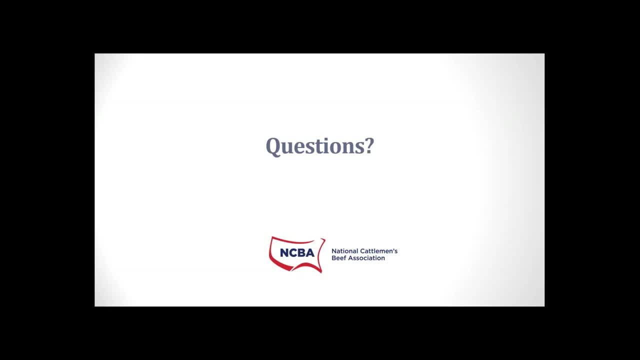 That was a big focus of his presentation, So you might check that out And if you have a follow-up question, feel free to email me, jwhite at beeforg And I can get that question to Jason or some of the folks at Noble if you want to get a little more specific on that. 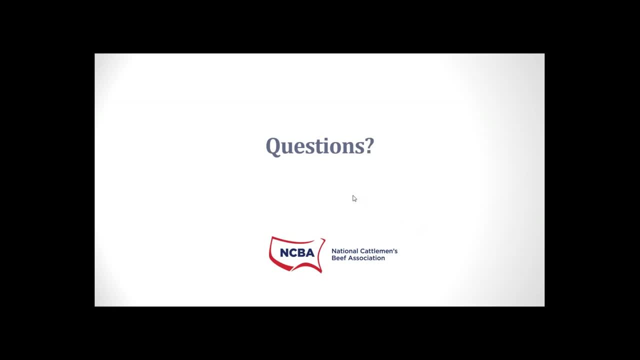 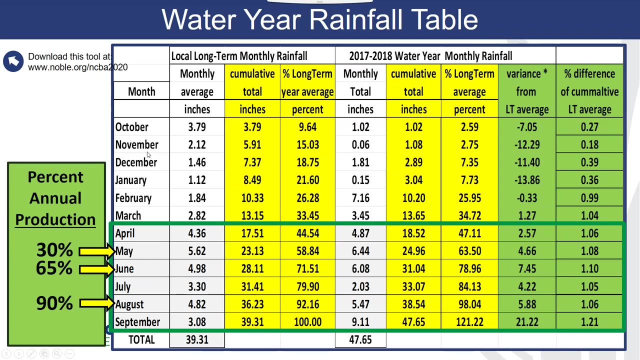 Hugh, I'm going to hand it to you if you're ready. I'm ready, Go ahead, Okay. All right, Are you seeing the water at your table there, Josh? Yeah, it's up, Okay. In particular, if you look over here on this left side, can you see my arrow being moved? 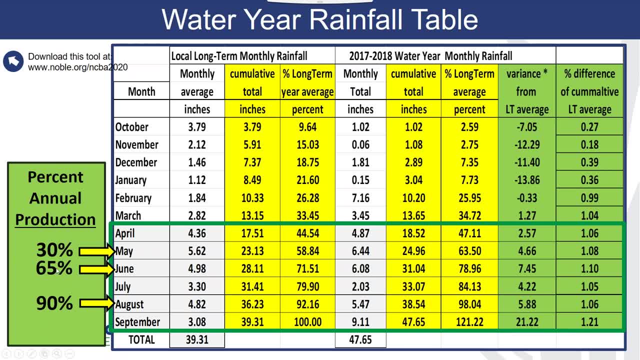 Yes, Okay, That percent annual production where there's 30%, 65%, 90%. your NRCS- local NRCS- can give you an idea about what annual production curves would look like. It's going to be a little bit different than any general area. 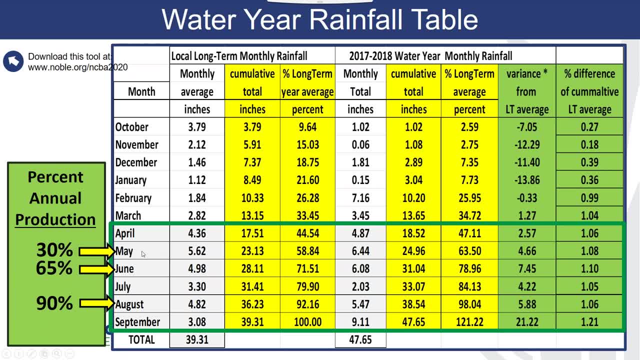 And then, for you know, here in the Southern Great Plains, and really as you go up to the Northern Great Plains, by the time we get to the end of May we expect about 30% of annual production. That may be 25 in some areas. 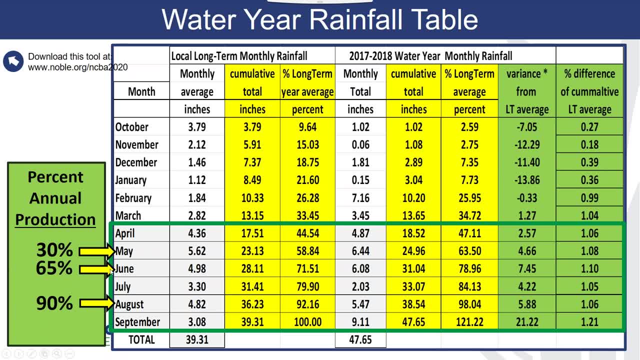 It may be a little more than that as you get further south, And then 65% about the first of June and 90% by the end of August. So we've got some parameters to where we typically know that there's a certain amount of production that's going to start slow in the spring and then it's going to start slowing down in the fall. 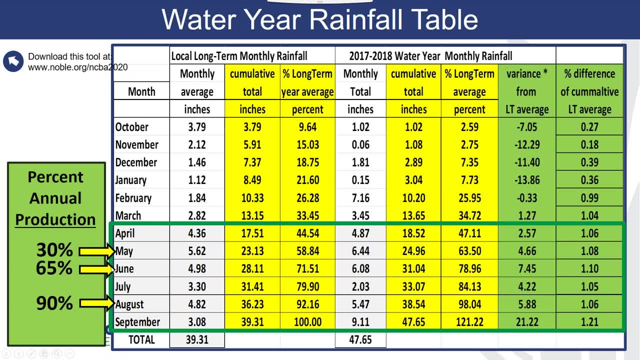 And then it's going to really take off as we get to that early part of the summer And then, when the rain begins to slow down- at least in our part of the country- we usually see a slump in July and August And at that point most of the moisture that we're going to have accrued to grow most of our forage is going to have already occurred. 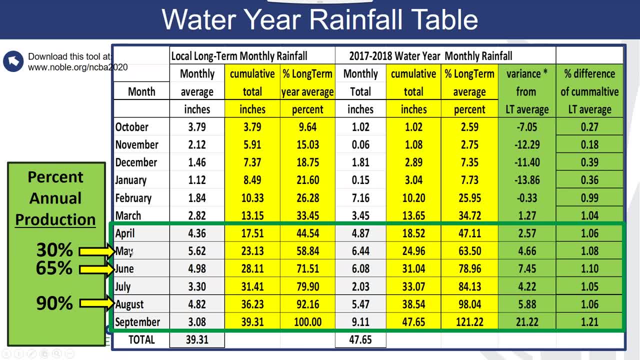 So that's where I'm looking at those critical dates. Knowing that I've got about 30% at the end of May- end of May is easy to remember- I'm looking at about what I need to trigger that And if I look down over here, where I've got this about 60%, 55% to 60% of the long-term average, these numbers here are just the long-term average compared to what is the annual average based off of each one of these months. 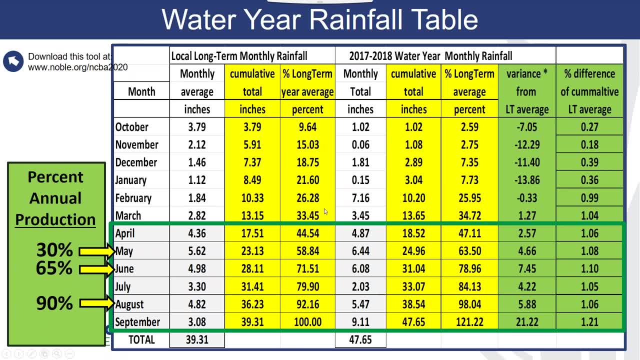 So here's the cumulative, Here's the long-term average. So, as you go down through here, you've got some trigger points And then, as I pointed, over to this variance, When you're going through and with this table- if you wanted it, I could provide it to you. 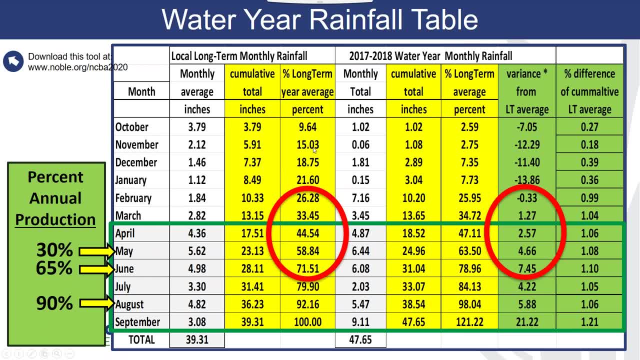 All you have to enter is this white column. The rest of it's already pre-calculated for you, So you'd have your long-term average conditions. Then you get into your actual- you know, the records that both Scott and Frank were talking about. 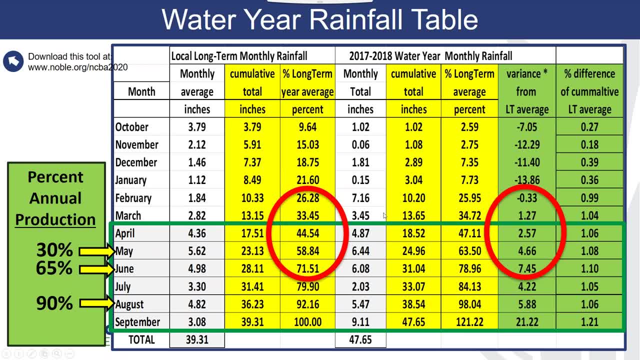 Plug that in for the growing season that's occurring going back to the beginning of October of the year before, And just see where you're at. And there's here where I look at the triggers When I get down to March, if I'm in a negative number or close to zero. 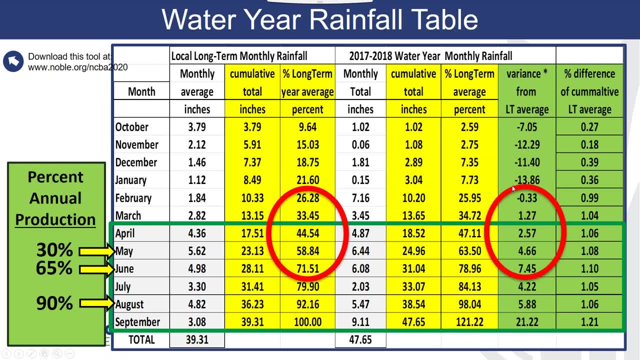 I'm paying really close attention to what that spring would be If I'm down, say, when we got into 2011,. that year, when we got into May, we had producers calling me up here by the time we got to 1st of May. 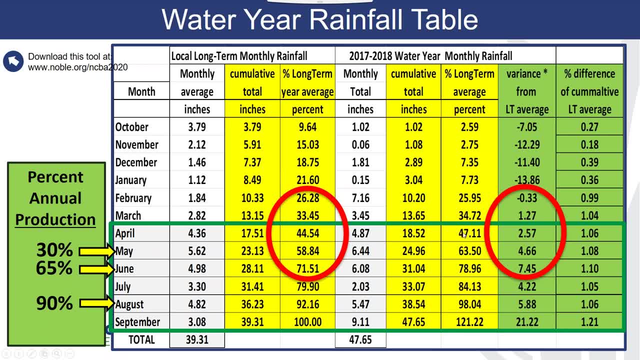 And where we should be about 47% of the long-term average. by that- or I say 44% by the long-term average- at that point We were down at 20.. So we were 24 percentage points below where we should be at this point. 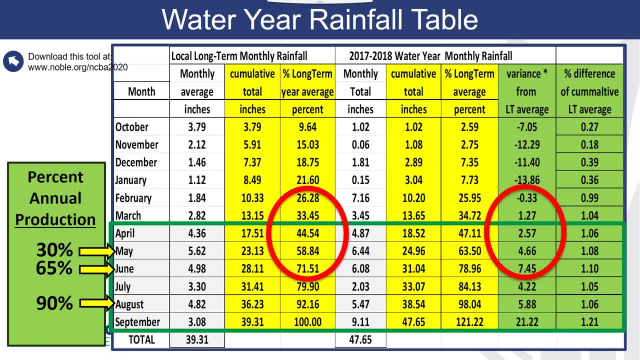 And that was the trigger point. So you know, I had producers say I think they're going to destock. Well, I had several of them destock completely. I just said, look, I want to save my land resources as opposed to sacrificing. 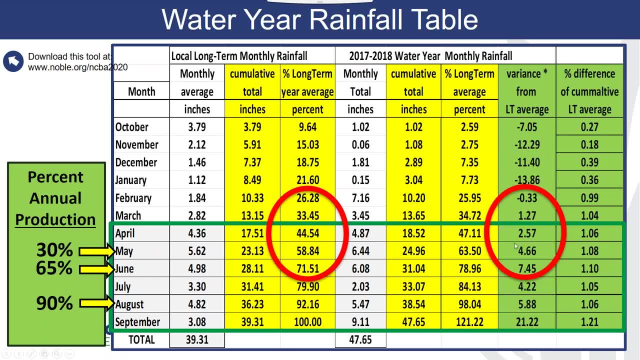 or trying to manage the drought. I had others that had pretty large operations, that were pretty proud of the cattle. They destocked by 20%. That was their trigger. is they if they were 20% here? they destocked by 20% and then reassessed it. 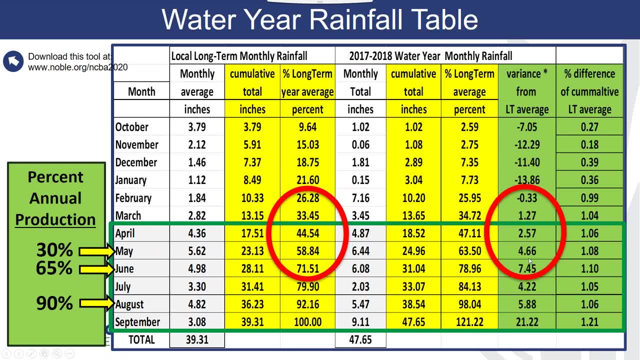 And then when they got down into the end, into May, and they saw that the long-term forecast was that for that drought to continue through 2011,, maybe into 2012,, they destocked another 10%. So this was the trigger off this variance that indicated how much they wanted. 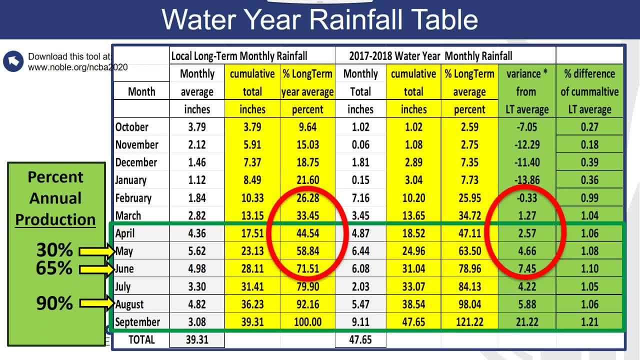 to reduce their stocking rate initially. Did that help explain that? Yeah, I think so. And you're, you're running, you're you could do this calendar whatever you know, starting and stopping with whichever month made the most sense for your grazing season. 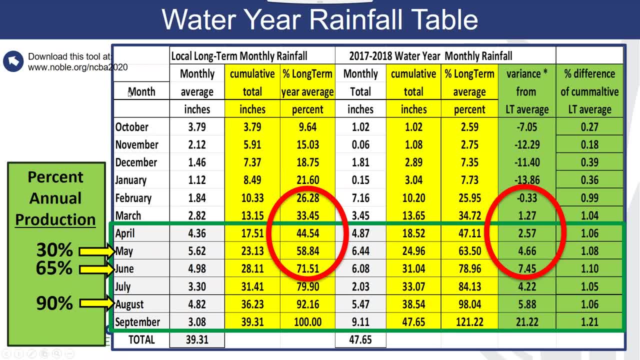 or production system, right. Right, You know, depending on where you're at this, this, this may look a little bit differently. especially, get over into California, Scott, you know, it may not make any sense at all for you. 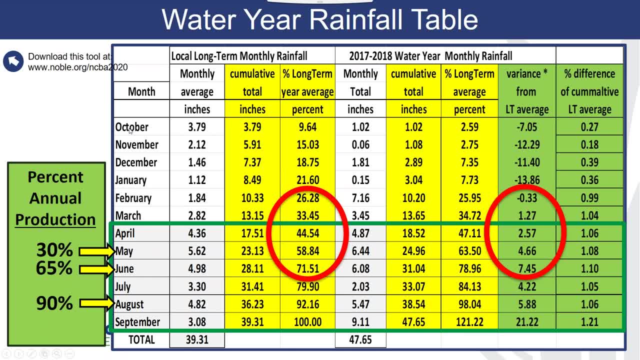 depending on when you typically expect your, your, your range and the recharge to occur. But in this part of the country where we have this bimodal rainfall, where we get fall, I mean rains in the spring and then another, typically you know- set of rains in the fall. 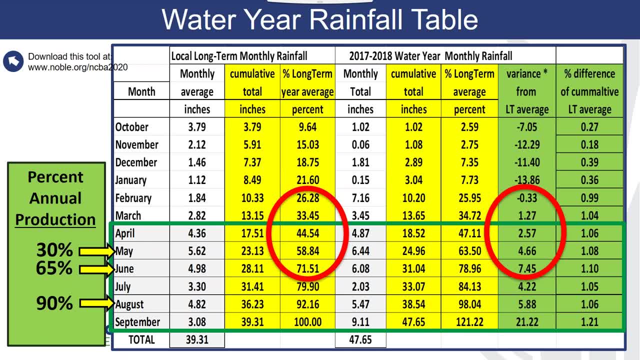 this tends to be relatively accurate for us, But until you put it out and study it, it'd be you know it can be easily adapted to fit your purposes. All right, I'm just catching up on the questions here, Okay. 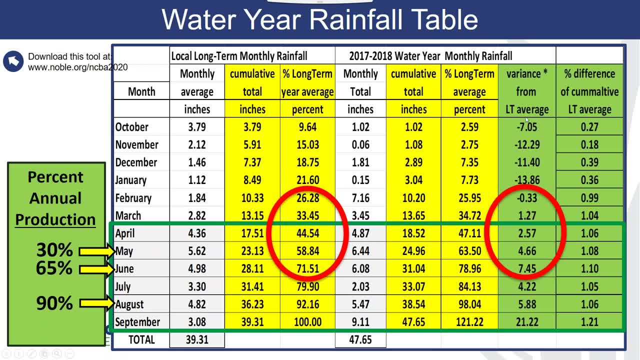 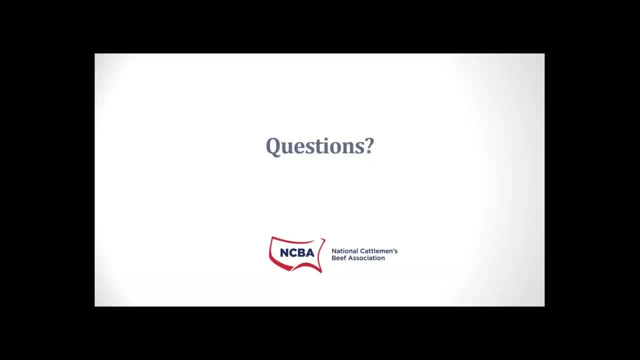 Um, you can take it back if you need to. Yeah, I'll do that, Scott, you. um, I have one on water resource development. You talked a lot about that. Everyone talked somewhat about that, but, um, you know, explain. um, I guess. 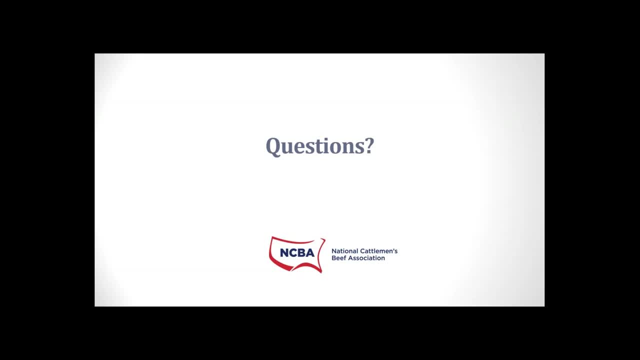 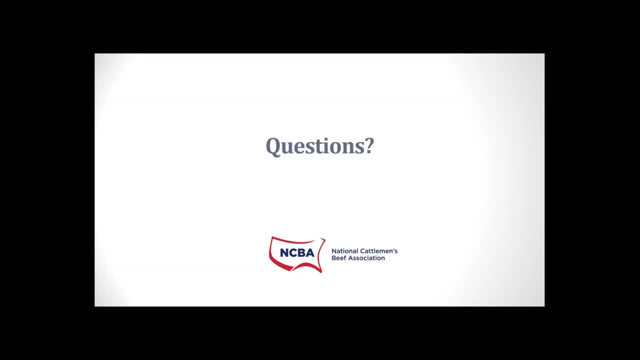 So that's when we got together with NRCS and came up with some additional methods to put this system in and trying to maximize what we could do, which included, you know, drilling for new wells. But yeah, we it's, it's, it's a product of having to deal with those droughts and not 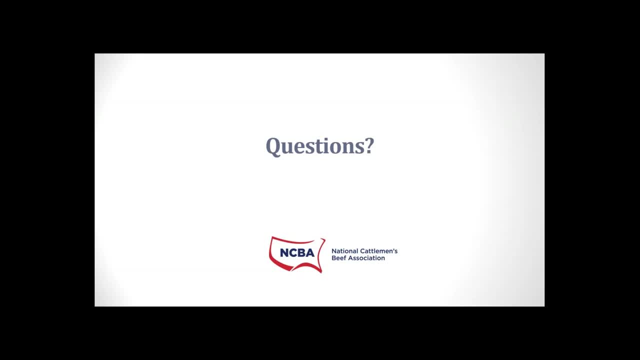 having enough water and trying to figure out ways to have more water available throughout a drought throughout the ranches, And have you guys been pretty happy with setting it up on solar? Has that worked well for you? And I guess what's the longest running system there that you've had powered by solar? We started using solar 20 years ago and thank goodness that the technology has come a long way since that time And we have a couple of systems where we had put in two different – the original system failed after about eight or nine years and then we put in another system. 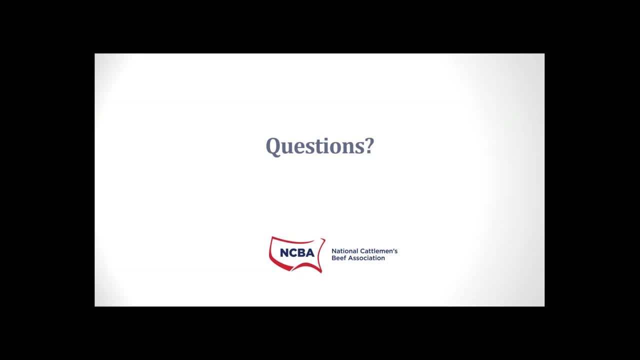 And then when we went – put in this two-inch line and connected all these different systems. So there was actually some places that we had solar pumps, that they weren't coming from a well. They were lifting water out of some of the ponds and putting it into storage tanks. So we took those solar pumps out of the ponds and hooked it into the main system, which was much more reliable. We're fortunate enough to have a really good spring at one end of the ranch that's never gone dry, So that's always – that's kind of provided to be a good base built the system off of. 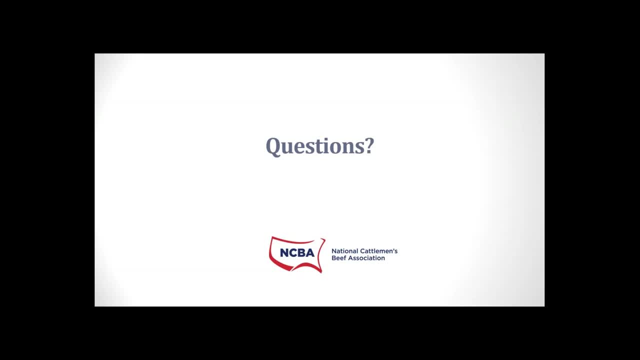 And so we're looking for ways to maximize that water source and spread it out to different sites. on the ranch Frank, one for you. You mentioned having good results putting more cattle into one group and rotating maybe a little more frequently, or just changing up your grazing rotation a bit. 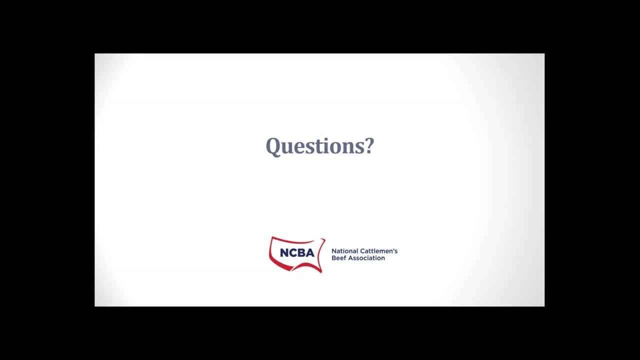 What – I guess what's your experience with that? Was that something that you worked into, Because I know you mentioned that you might want to ease into that and not try that all at once. maybe just go into a little more detail about your experience with that. 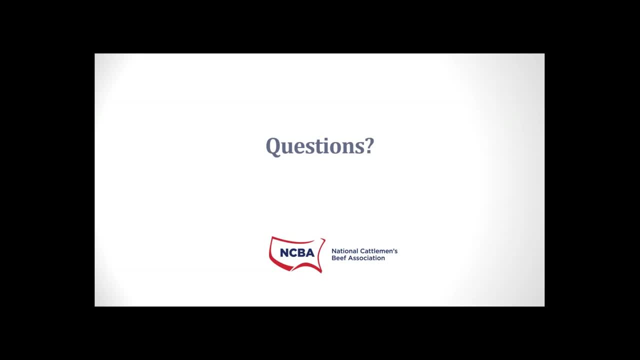 and and what you've learned with that process. okay, when my father was a continuous grazer- relatively live stocking rate and through ag teacher fitness college courses and whatnot- I recognize the benefits in rest and we started from time to time resting a pasture and then I had the opportunity. 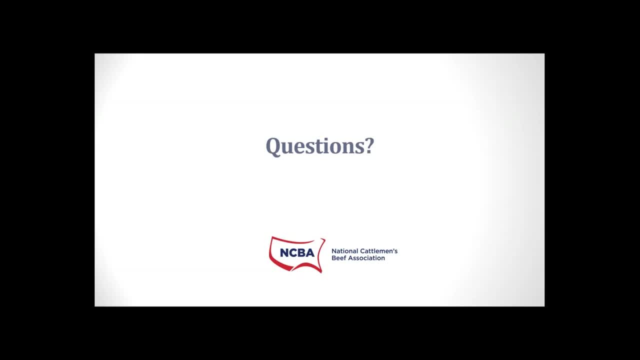 to attend Allen, savories and Parsons grazing school. came out of that school put in several sales and I wasn't real satisfied with them for a number of reasons. first, it wasn't I wasn't home. you might put me back onto my screen. you know I'll show. 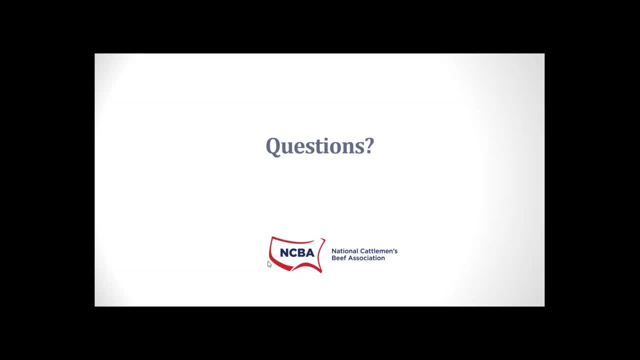 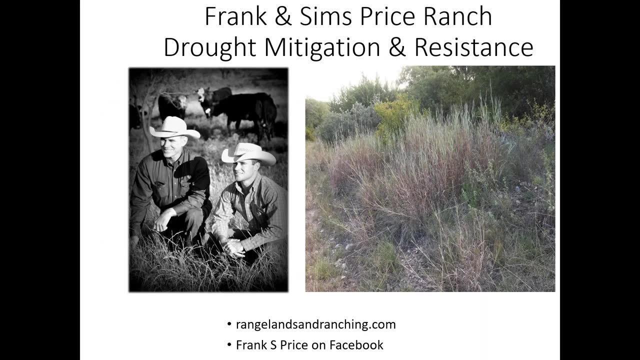 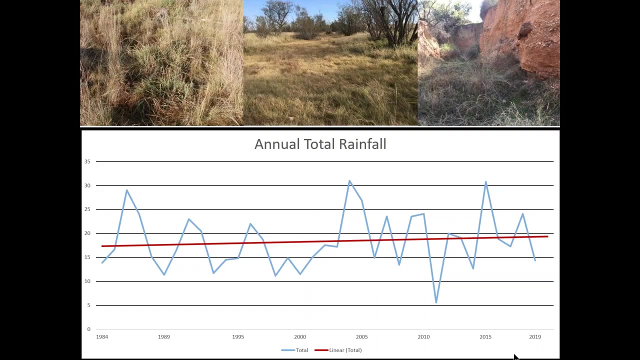 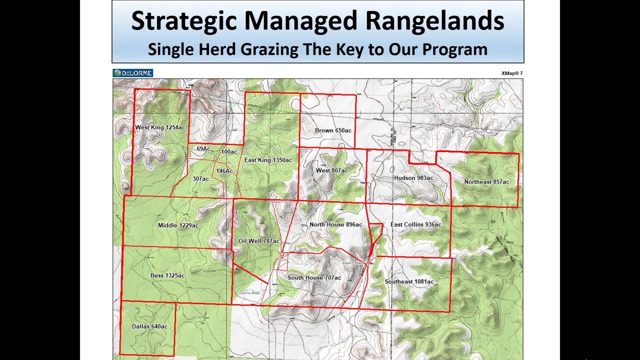 a a the pasture situation we utilized there, but we got away from grading sales and went back to continuous utilizing the pastures that were available. all right, this picture is a place that we lease. there's 17 pastures in that range. this picture is a place that we lease. there's 17 pastures in that range. 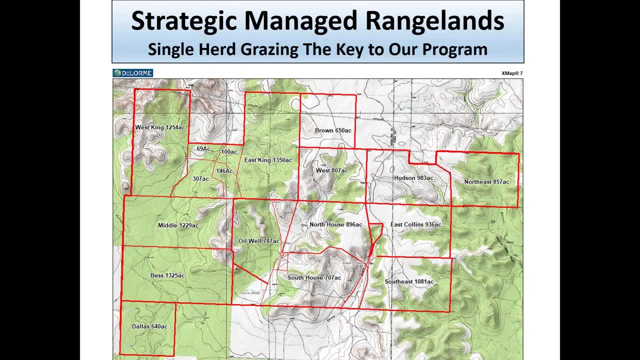 originally, it was two ranches that were put together, thus the number of pastures we had, and when we leased the place, we looked at it, we considered splitting it into two different grazing units. we were in the middle of a 2011 drought and we selected to go to a single herd program within that 17. 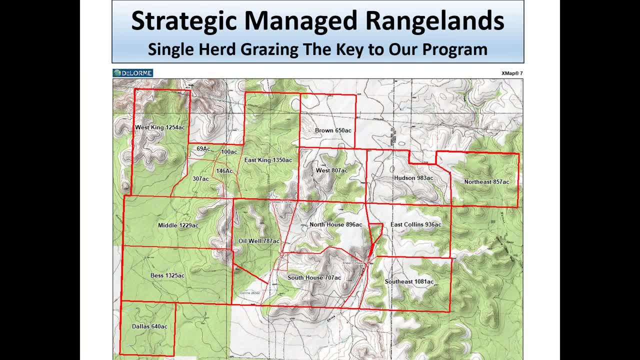 pastures and just any ranch I've ever taken on or looked at or anything. even it's just got four pastures. you configure a planned grazing program within that range without doing the going to the expense of building a lot of finches. now you can look at this topo map and 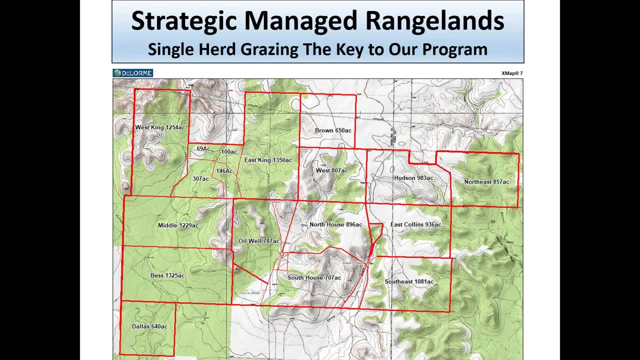 we've got considerable elevation change, brush issues and whatnot, and it's really hard to build temporary fences in this country, so we utilize those pastures. now we're talking about water quality when you've got a ranch like the one we're looking at here and which was the traditional 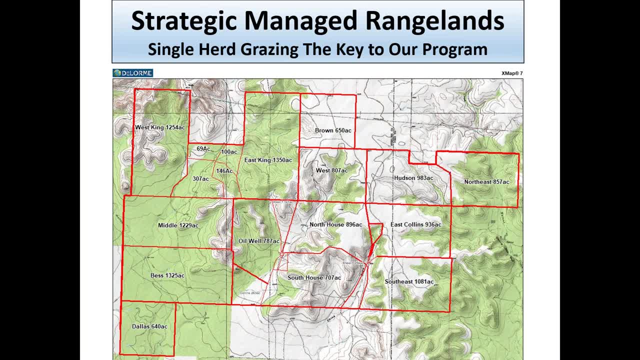 continuous grazing. each pasture had water systems that were designed for the number of livestock. it would be in that pasture year round. when you go to a single herd, suddenly you put a lot of demand on a single pasture. granted, it's for a short period of time, but you got to have a lot of water there. 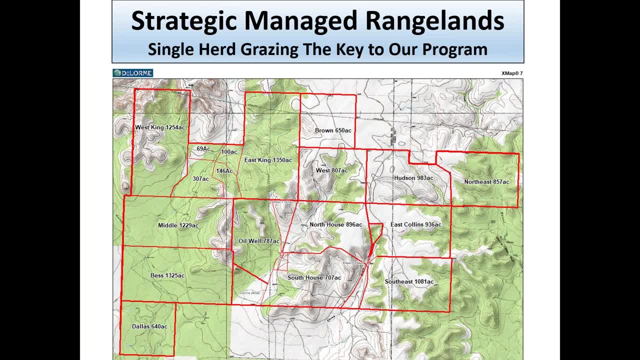 so once again, uh, as scott, through nrcs and an equip program, we were able to do some pretty extensive water development on this ranch and gave us the ability to have that single herd program. well, without that water development we could not have done it. great information. thanks for sharing that um. 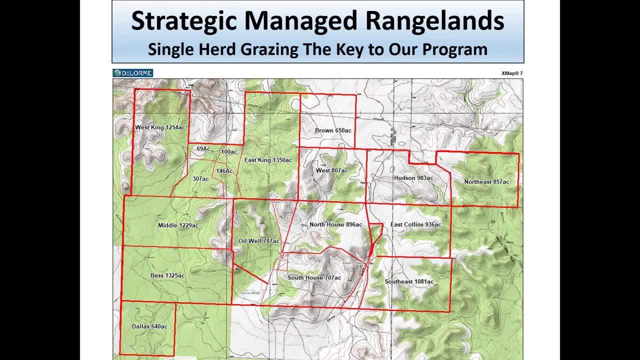 that's all the questions i have coming in from the viewers on the webinar. joe, do you have any, or do any of yourеру have a question or an answer to any of our questions? please feel free to contact us and we'll put them into the chat room or we'll get to them and we'll talk to you very soon. 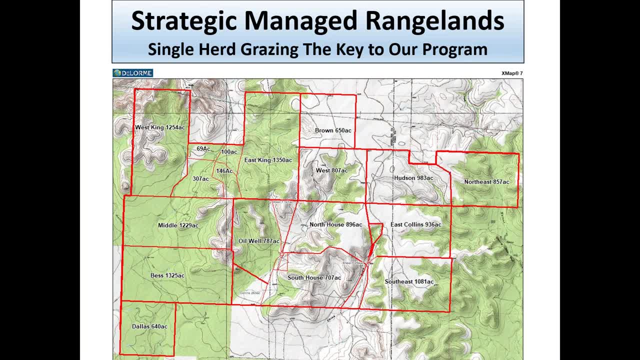 you as presenters have any questions for each other, happy to open that up before we close things out tonight. I tell you I've got. I've got a question for both Scott and Frank, but as as you look at moving into more of them, intentionally managing your operations, what was the biggest challenges that you had to? 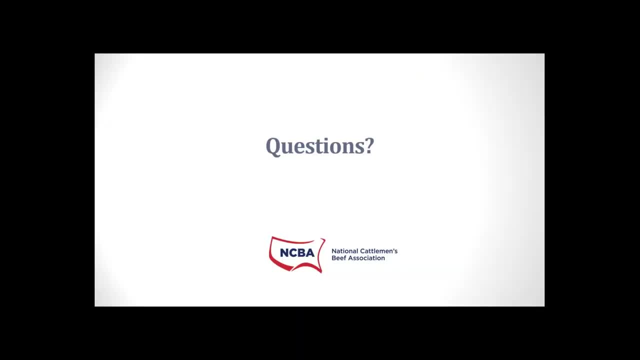 overcome? granted, one of them is water, but what was the biggest challenges that you've had to overcome and what were the successes that told you early on that you were on the right track? once again, I went through that grazing school, came out this plumb full of vinegar and went into too many grazing sales. they got too. 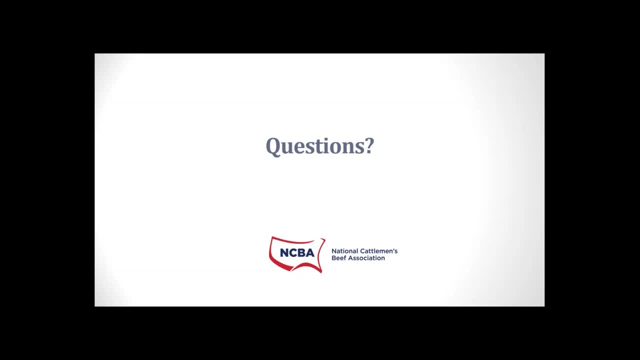 complex for me. I was disappointed in livestock performance and that's when I went to working my back way back to traditional pastures, probably because, uh, i liked uh paddling up riding through that traditional pasture versus uh riding through electric tension in the wagon wheel and that. 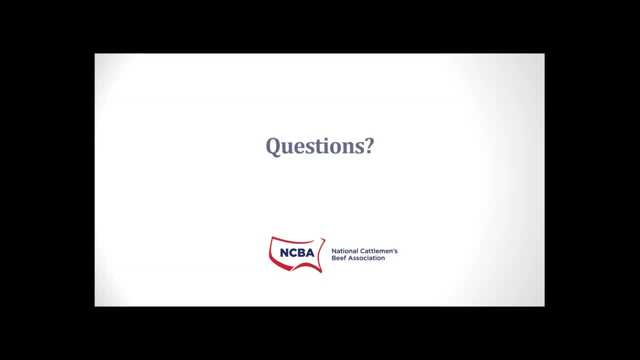 that's not a very uh. i don't know if that was a financial decision or not, but it's a lifestyle decision. but as we developed into that process of using traditional pastures, uh have become very comfortable with it and when i see things like that big blue stem that i highlighted, so 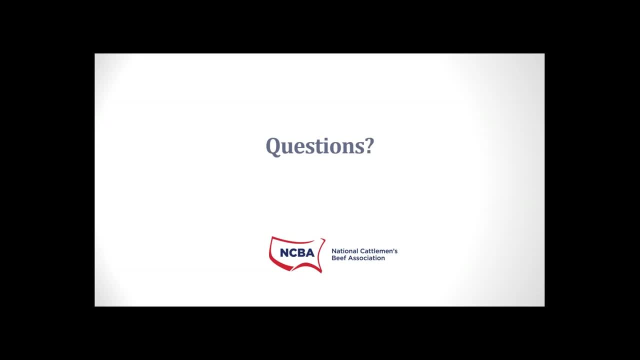 much, and the texas cup grass and the density of grasses, i get just plumb beside myself. it's seeing us improve and when we reach the point that we did not feed mature cattle, and when i say don't feed, there's no hay, no tubs, no blocks, no cake, with exception of the cooking cake to keep them gentle. 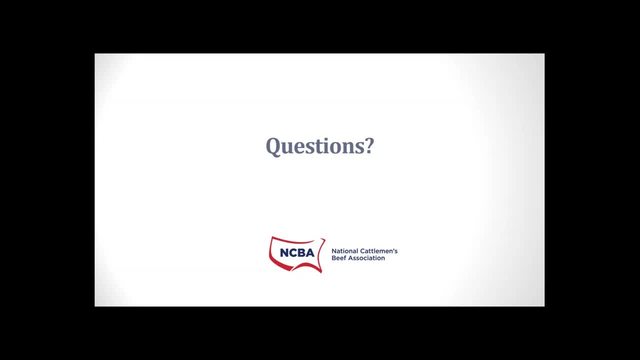 and whatnot. suddenly that operation has become consistently profitable. you take that ranch that i was showing you there with those 17 pastures. if you had livestock in every pasture- there's 22 sections there- you would have one full-time man. if you had livestock in every pasture, he would be a busy. 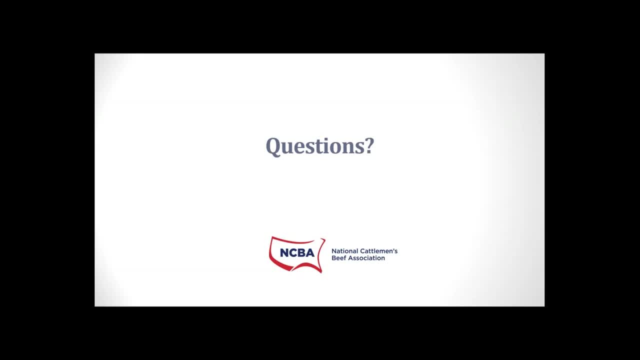 feller, tending to the water, the fences, the feeding of the livestock, and we've gone to this single herd. that's reduced our labor needs. so, uh, ultimately, profitability has been the key factor in what we do, and it's uh really exciting what i see happen on a continuing basis. 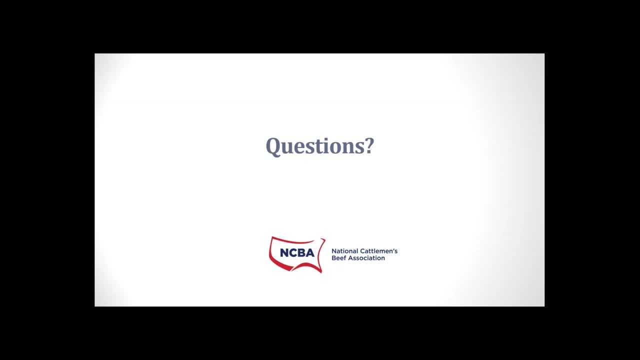 so i also went to a ranching for-profit school with stand parsons back in 1995 and when you come home from one of those fields- it was she laid滿. you're all fired up, start doing all these different things. but the problem is is when then you have five family dynamics and you come back from one of 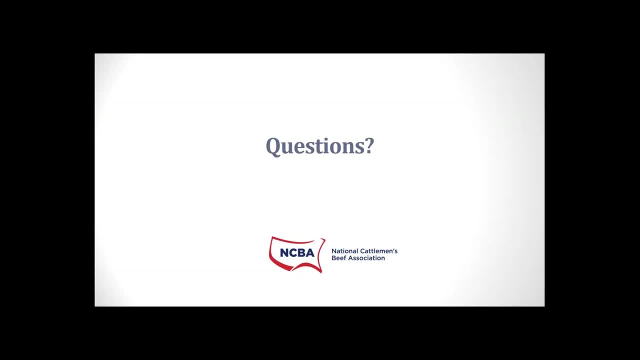 those seminars you're speaking Russian and the rest of the family speaking Chinese. so the challenges are the family dynamics of getting everybody to get on to the same age and start moving in that direction. when I came back from that- those seminars with my dad, who was a tremendous cattleman- he would have 30 to 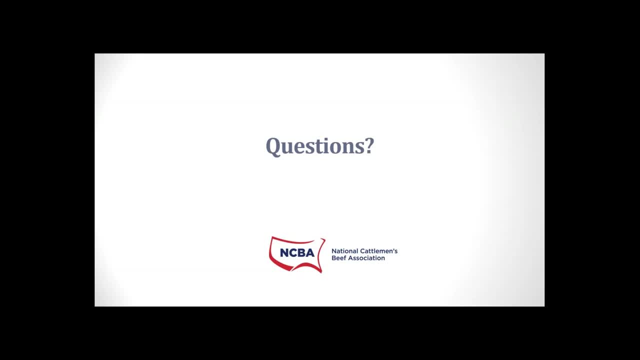 50 head and each of the different pastures throughout the ranch and that's where they would stay for the whole fall and winter season, spring, and so they're all fall cows and we would feed them after we brought him back from the irrigated pasture. so you're going to a multitude of different pastures to feed. 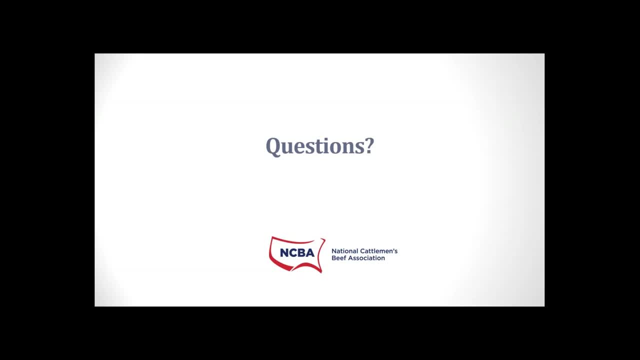 your cows, cattle, so the amount of hay that we fed, the labor that was involved, all those things, um, you know that they, they take a toll on your bottom line and so slowly we started working together to try to implement some changes and figure out ways to change the cost liability of some of the ways of doing things and uh, 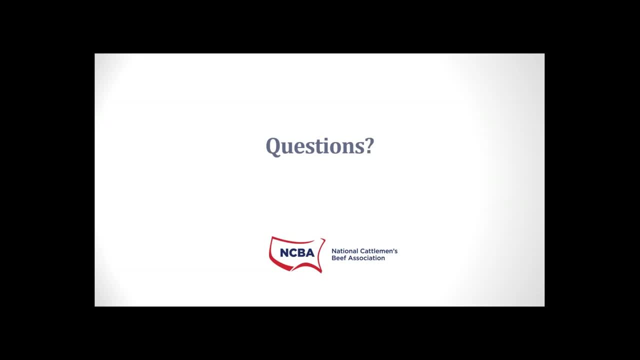 it's much easier to move some cattle, as it will get to look at them pretty darn well if you're, you're moving rotationally on a regular basis and so I've seen, I've seen the pastures are in better condition, they hold up better, they come back better from doing the rotational grazing with larger groups of cattle. 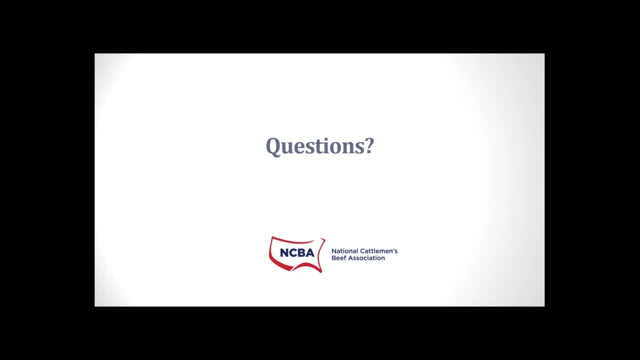 um, and the cattle get trained, they're easier to move and you get, we go to the gates and whistle, and sure we have to go after some with the horse horses but or the Honda's, but for the most part it's. they're kind of trained to move themselves because they know they're going to fresh feed. so we've had 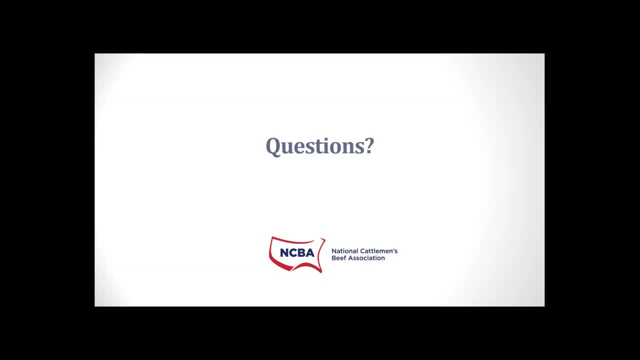 some good successes, but early on there was family dynamic challenges and we've got all that past us. okay, thank you. all right, yeah, go ahead. I know some Bob grazers that are extremely successful in what they do. I mean, it's amazing the livestock performance in the land change for the better and I honor them for what. 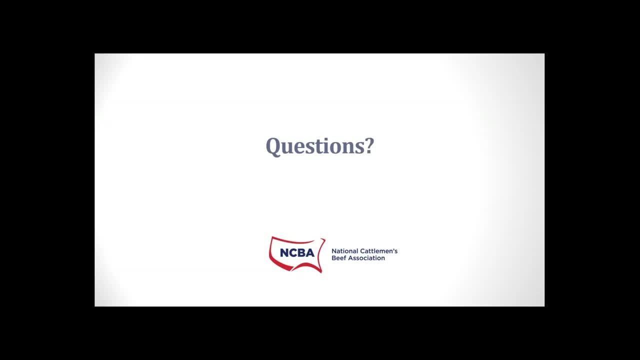 they do. I'm not structured mentally to go to that intensity level. that was one of the things with the studies with savory and portions. I had to admit to myself that that was not the route I wanted to go, and so I kind of backed off to what fit.